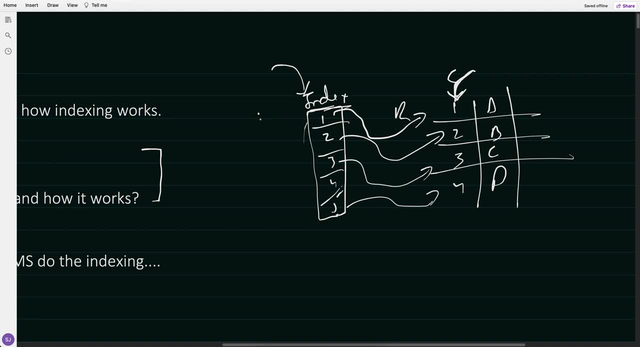 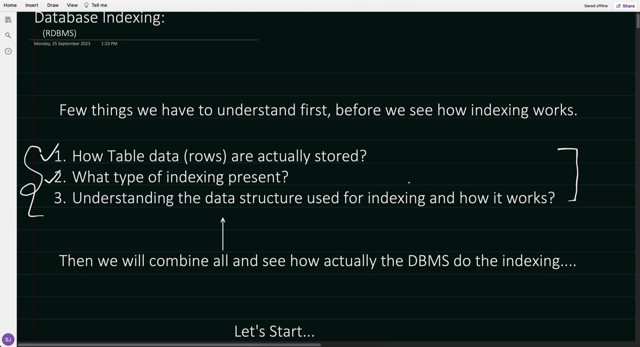 it will able to fetch faster. okay, you want four, so on this index it will able to find the faster and it will goes to point to the particular row, okay. so what i'm trying to say is that this is very high level, but today we are going to step down into one level deeper, because that's where 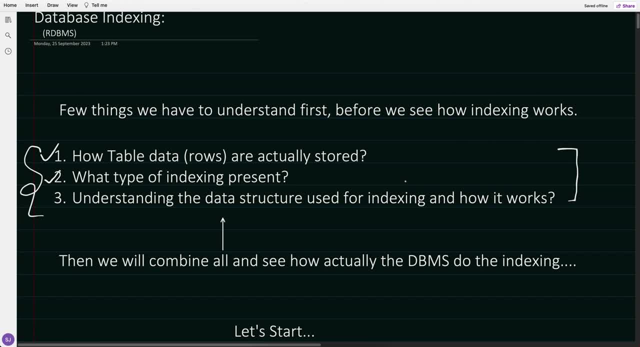 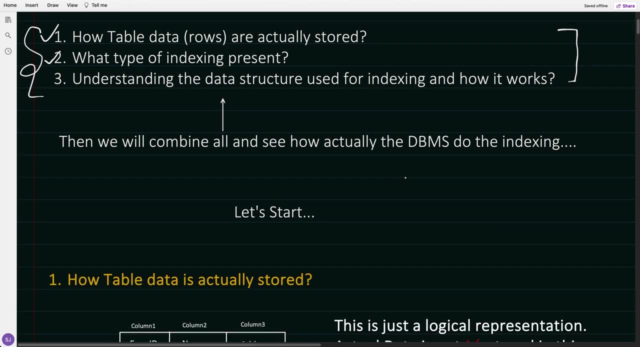 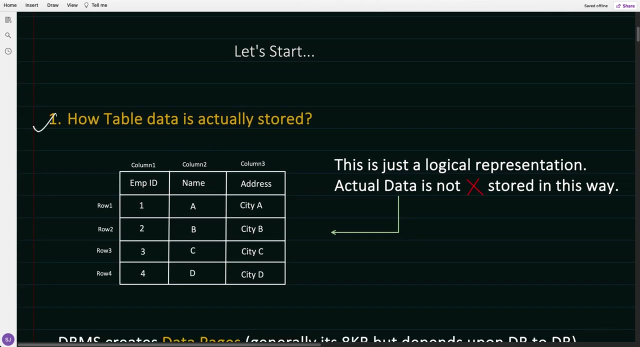 the interview follow-up questions ask: okay, so now let's go into little bit deeper, and i'm not going to shut down or cut down this video shorter, because if even if it is go little bit longer, i will continue to it. i will not do any trimming for sure. okay, so let's first discuss how data is actually stored. 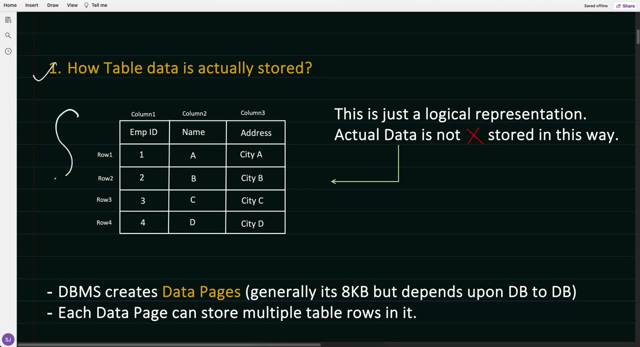 very, very important. so now let's say: this is your table. you have a row one, two, three, four rows and three columns and let's say: these are the three columns: employee id name and address. so this is generally a very, very- you can say that- typical table, let's say employee table. so this is just. 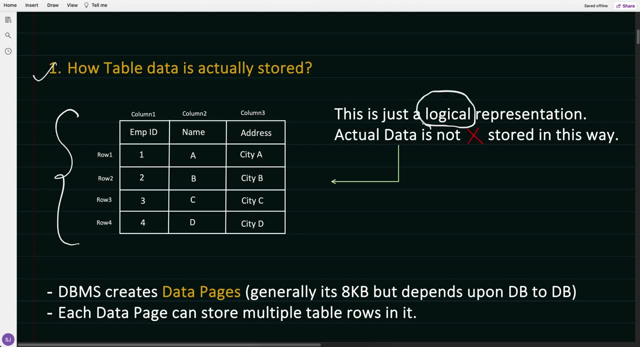 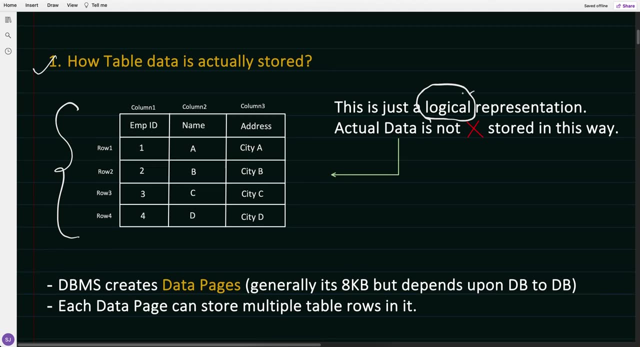 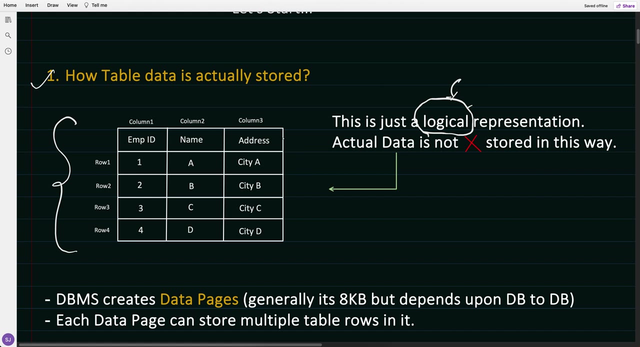 a logical representation. this is just a logical representation. this is now. this is not how actual the data is stored in the db. right, this is just a logical representation, not a physical representation. remember that. okay. so when we say that, hey, this is logical representation, then how the actual data is stored, okay. so now let's say in our table we have this data: four rows, three columns. 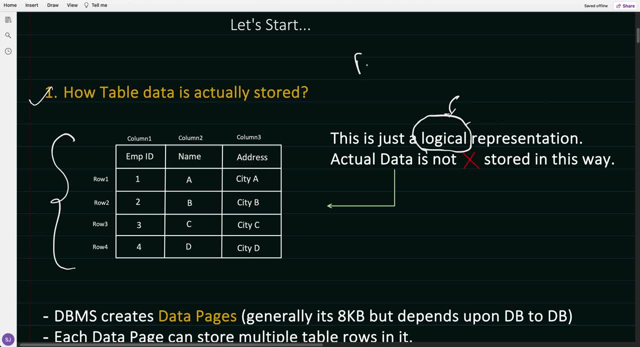 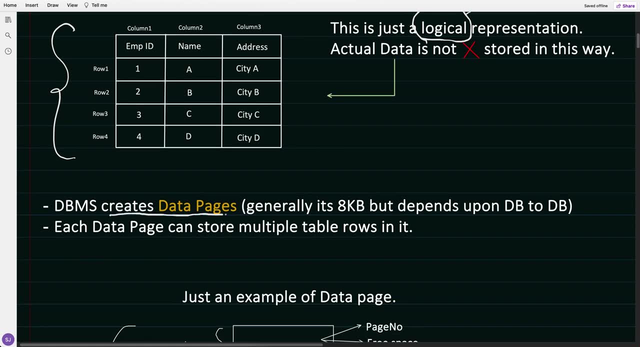 so what dbms will do? what dbms will do database management system? what it will do? it will create data pages, right, and one data page. generally it's generally of 8 kb in size, depends upon what db you are using. okay, but generally the size of one data page is 8 kb, okay. 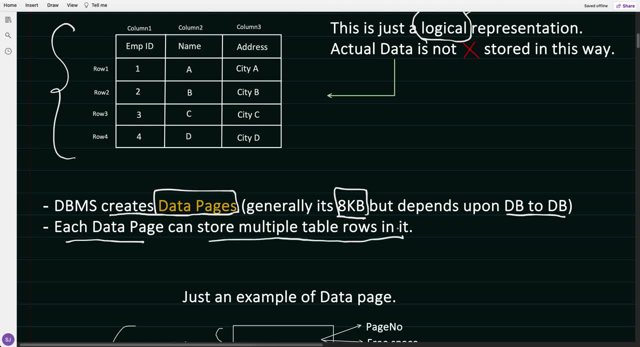 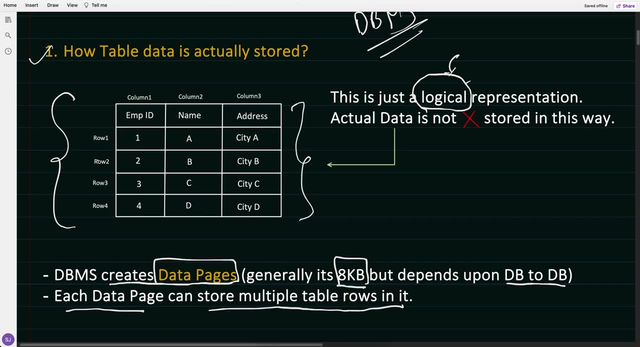 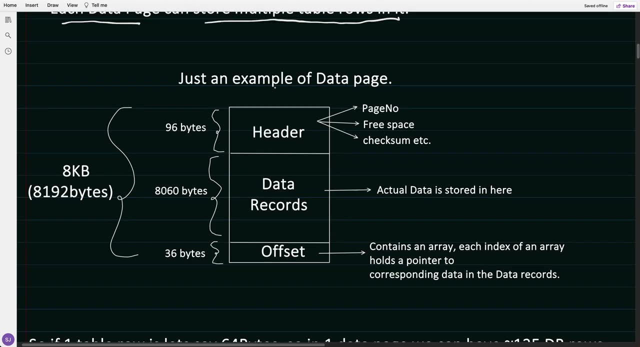 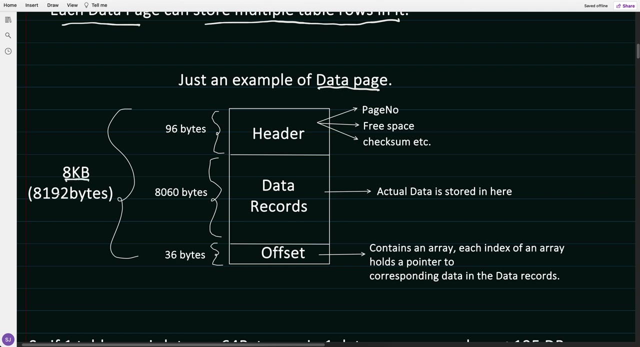 so that means each data page can store multiple table rows in it. okay, so now we know that this is just a logical representation. these rows are actually stored in data pages, which dbms creates, right, how? so this is how a typical data page looks like. so when i say that it's a 8 kb, so in 8 kb, how? 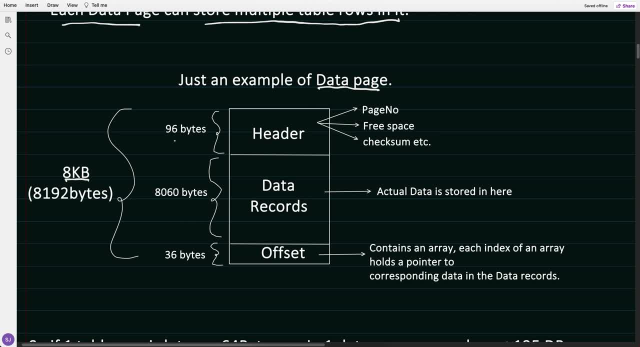 many bytes are there? 8192 bytes? okay, 96 bytes are reserved for the header In a header. what generally information it has. It has page number, how much free space this page has, checksum and et cetera. Okay, so header information. 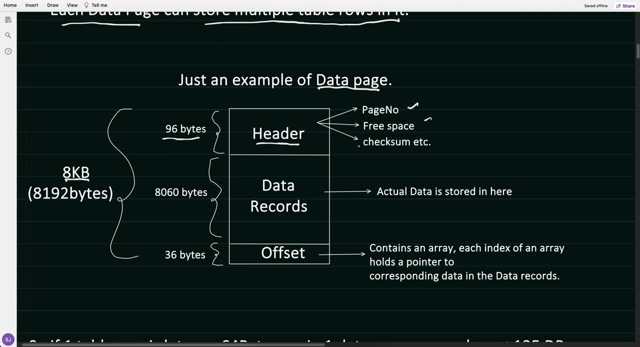 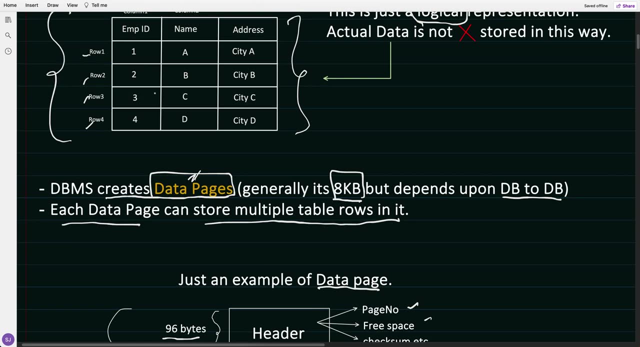 I would say that it has very basic information like page number, free space, checksum, et cetera, which is 96 bytes. After that, 806 bytes. 8060 bytes are totally reserved for data records. When I say that data records, it is actual. the rows: 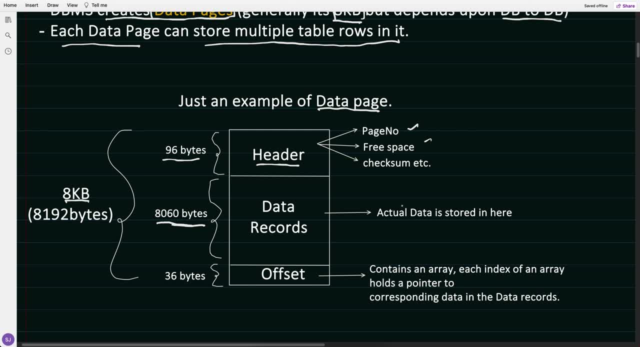 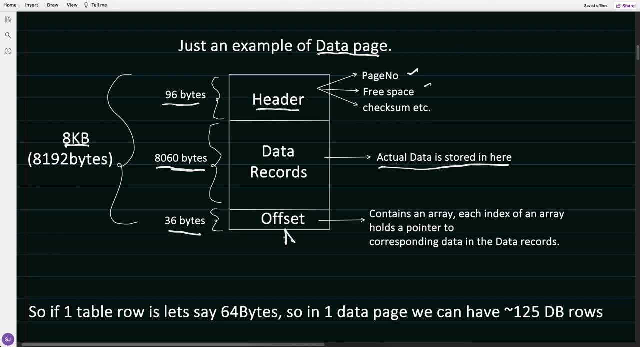 So here the actual, the rows will be stored. So actual data is stored in here, And last 36 byte is known as offset array actually. So what does offset contains? is it contains an array, And each index of an array holds a pointer. 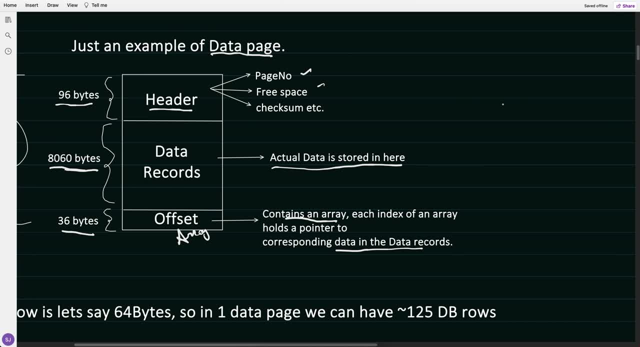 to the corresponding data in the data records, right? So in this data page this is an header, Let's say it has the pages. row one data. row two data. row three: data. let's say Only three rows are there. 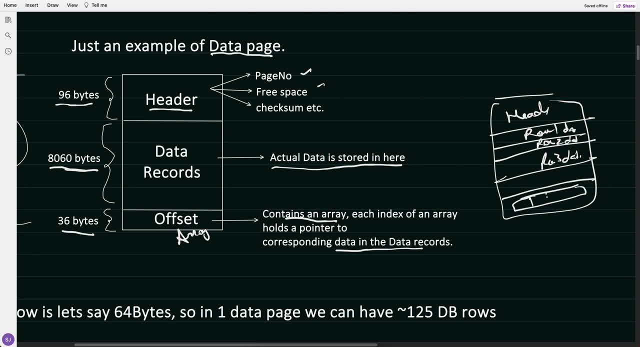 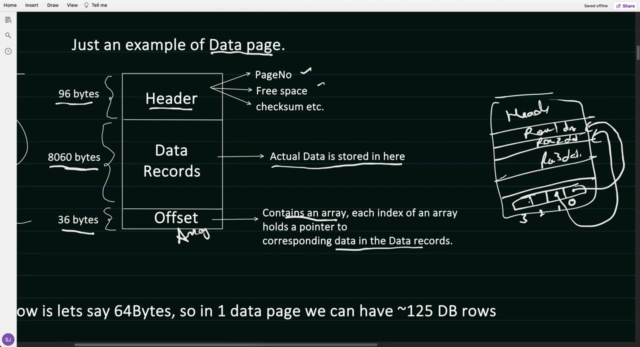 In this offset there is an array: Zero one, two, three. Zero one, two, three. So zero will point to, let's say, row one, One will point to, let's say, row two. So what I mean to say is that this offset array 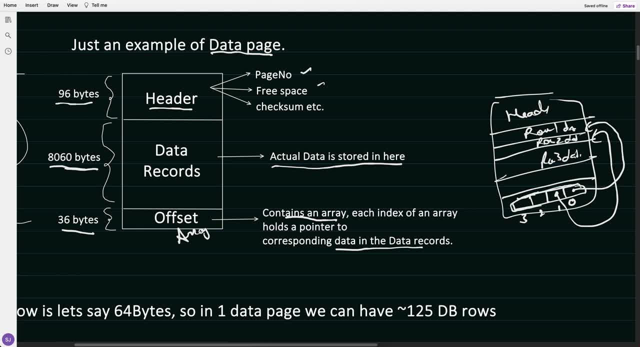 contains an array of. you can say that a pointer and this what it point to. it point to the actual rows. Now you can ask me, hey, why we need this offset array. We will see that how it helps. DBMS. 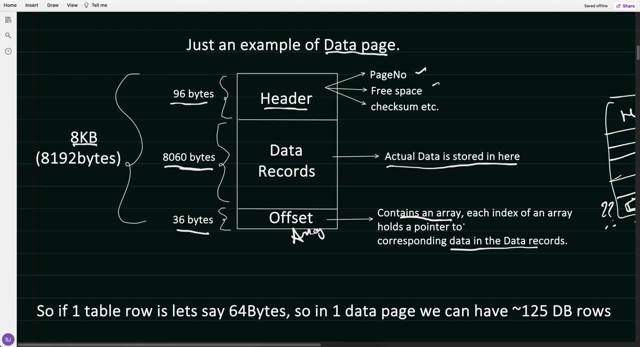 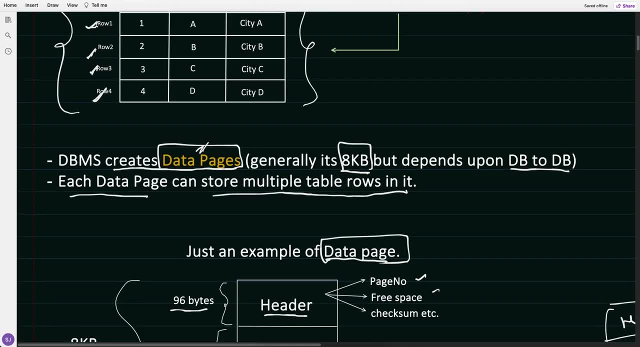 But don't worry. First of all, what I want you to understand is how data page looks like. So one thing, very basic thing you should know is: DBMS creates data page and inside a data page, actual rows are stored. okay, 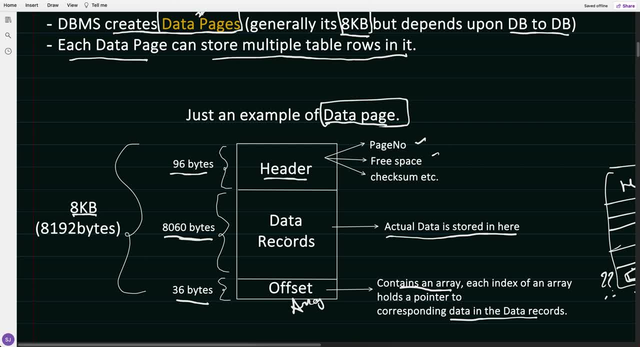 So that only you should understand at this point of time, And don't worry about the offset array. We will see with an example and how DBMS make use of it. Okay, So offset is just an array of you can say that pointer. 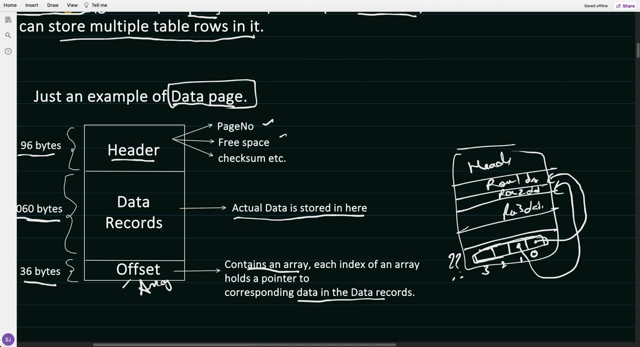 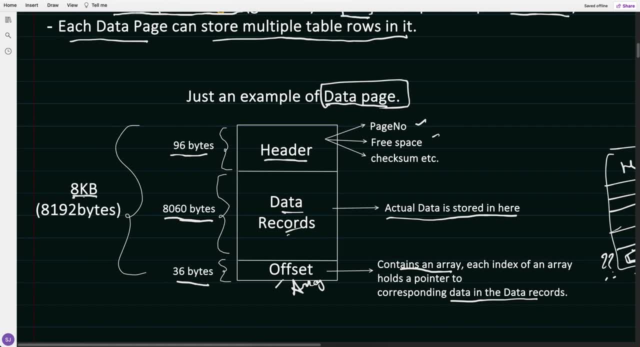 pointer to what? Pointer to the particular row inside a data records space. Okay, So, total eight KB data pages and out of this eight KB, eight zero six zero byte is actually there for the rows or actual data and rest is for header and offset array. 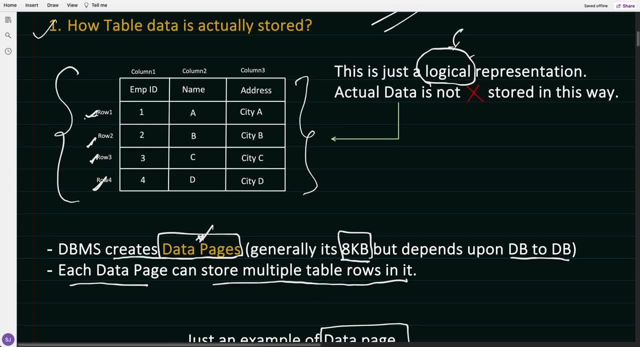 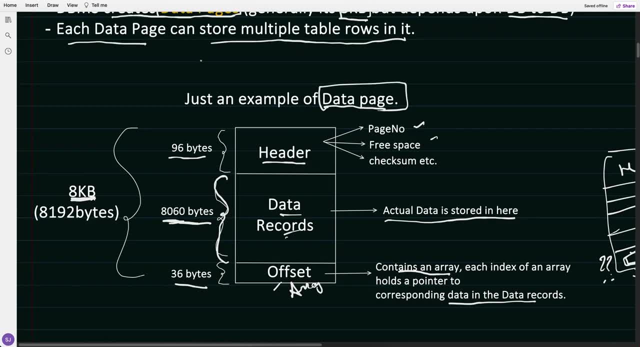 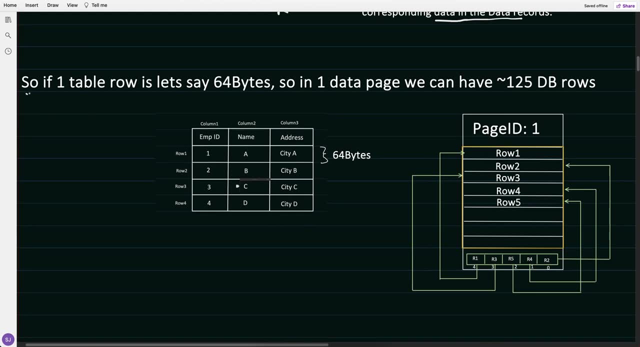 Okay, so now it's clear that these rows which we are creating- it looks like it is clear, okay, Okay, creating- it's stored like a table, but actually it is going here in the data page. so now let's see this. so if one table row is, let's say, 64 bytes, so now let's say this row one is of 64 bytes. so 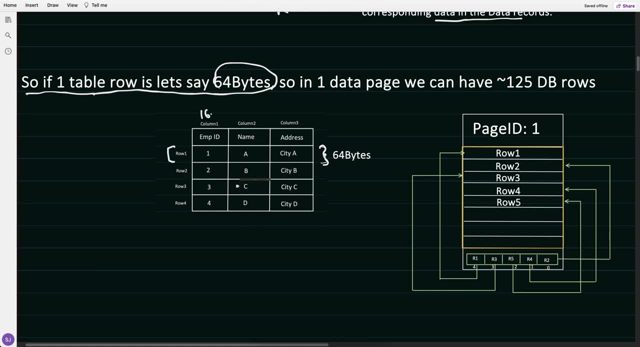 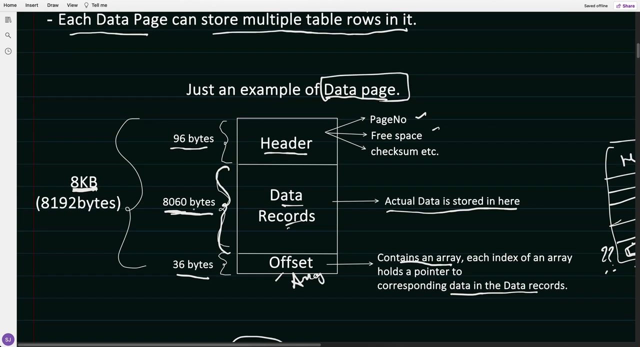 this is, let's say, i'm just saying hypothetically, let's say, it is 16 bytes, right? this is also 16 bytes, right? this is 32 bytes, i'm just saying, and it all combined to 64 bytes. so one row, one row is your 64 bytes, right? and we know that. for storing the rows, how many bytes? 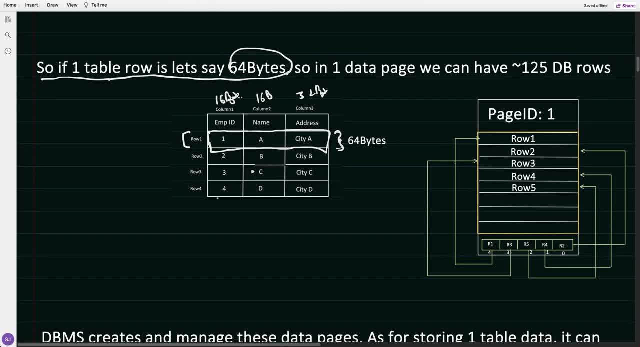 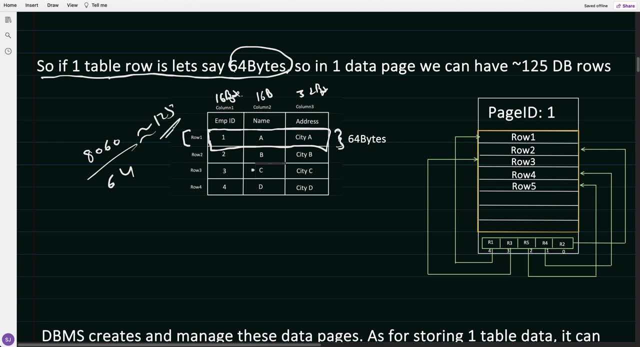 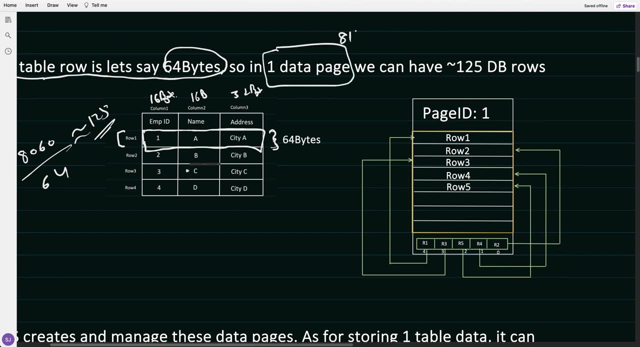 it is available in our data page: 8060 bytes, so 8060 divided by 64, so almost around 125. it comes. so means in one data page. if it is a size of 8 kb, then we can store 125 db rows in it. 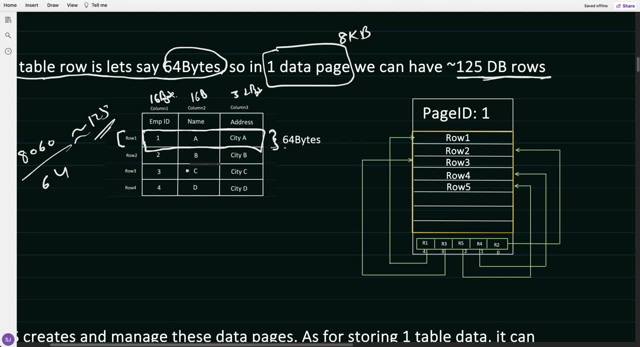 right. if one row is of 64 bytes and one data page is of 8 kb, then we can have 125 db rows in it. right, and how data page is generally look like. so we have header just kept for simplicity only page id or page number, like one right. and then the second part is: 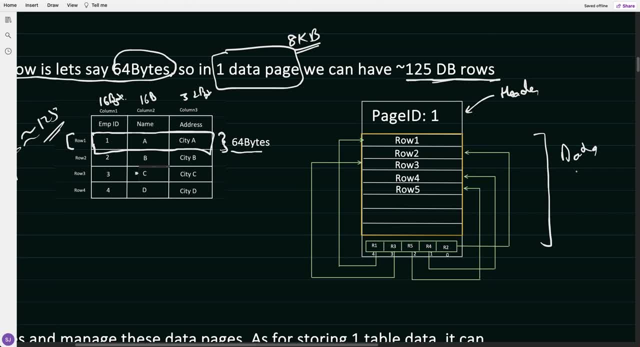 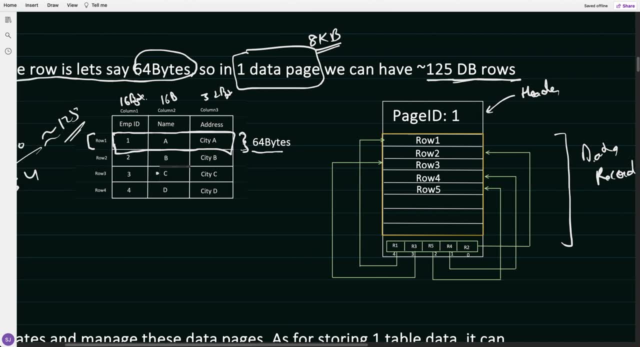 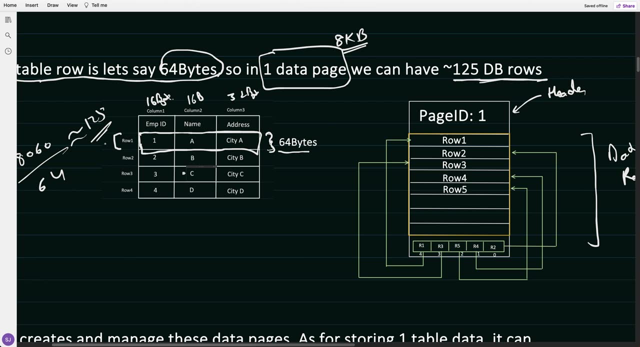 your data record, data record which actually holds the data, the way the row is inserted into a table or by a user. in the same way, generally the rows are inserted. so user has inserted row one, so it has inside this. it put row one, row two, row three, row four, row five, row six, row seven, row eight row. 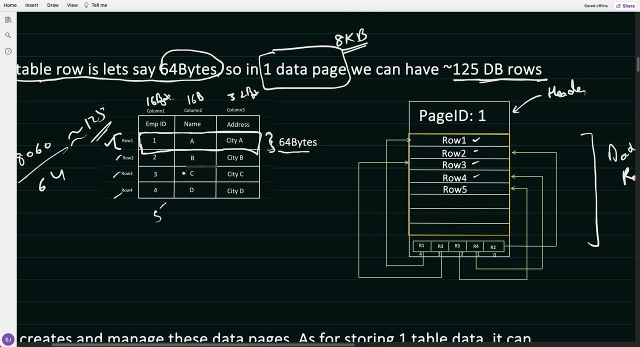 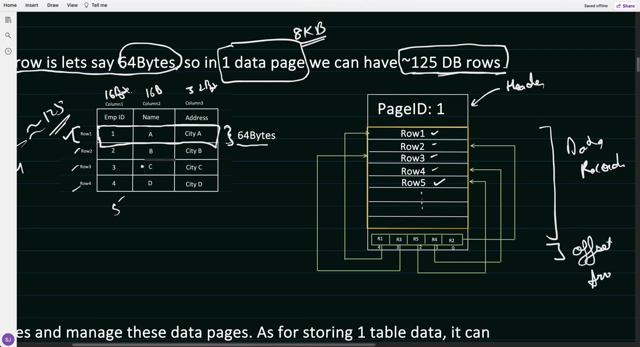 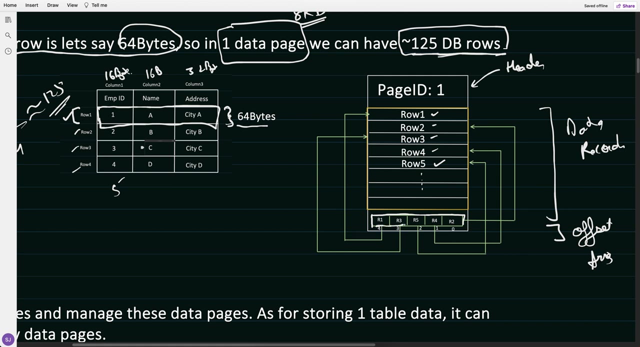 three row four, row two, row three, row four. and if let's say it has added five, row five, okay, like this, it will add how many it can store: 125 db rows it can hold. then what is the third step? third step: i told you it's an offset array. so here i have created an offset array. okay, so this offset array. 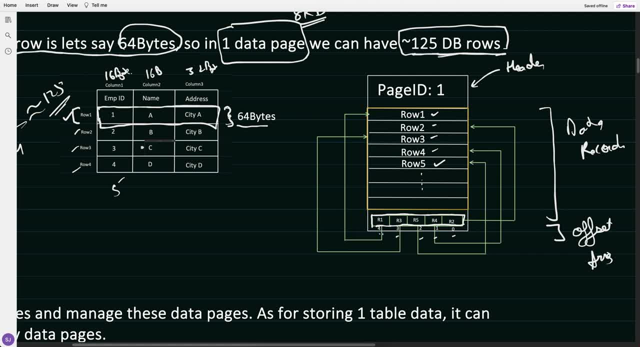 is indexed like an array: zero one, two, three, four, five right. zero one, two, three, four, so zero. it is pointing to, let's say, row two. this one is pointing to row four, two is pointing to row five, three is uh, three is pointing to row three, and fourth index is pointing to r1. 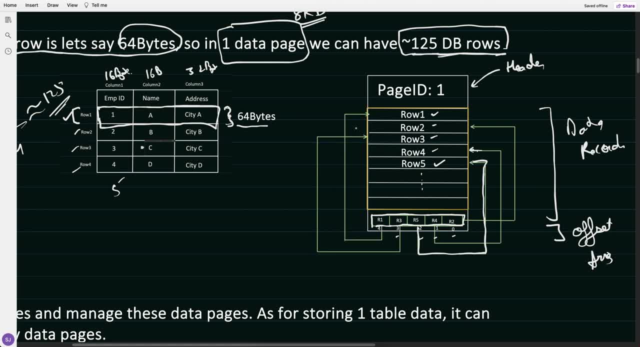 okay, so what does offset array hold is now it's clear, it's an array and this array actually contains a pointer, pointer to what the actual data which is present inside the this data page. now you can ask me, right, hey, what is this ordering? at zeroth index, r2 is stored. 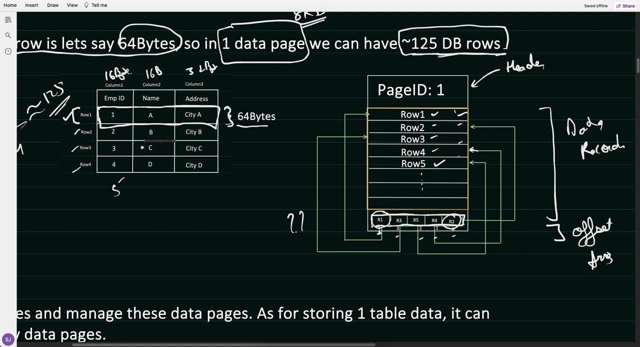 right, and at fourth index r1 is stored. so it doesn't make sense, right? it is not ordered. not increasing order, not decreasing order. what is this order right? so don't worry about that part, because when i will come to that then it will make sense better how dbms is. make use of offset array. 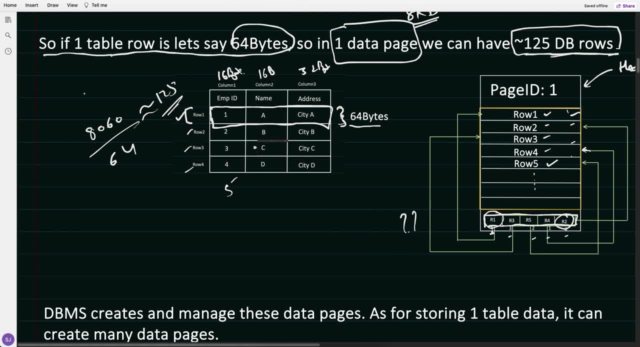 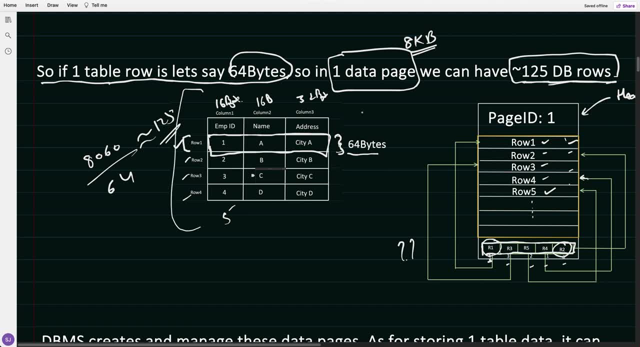 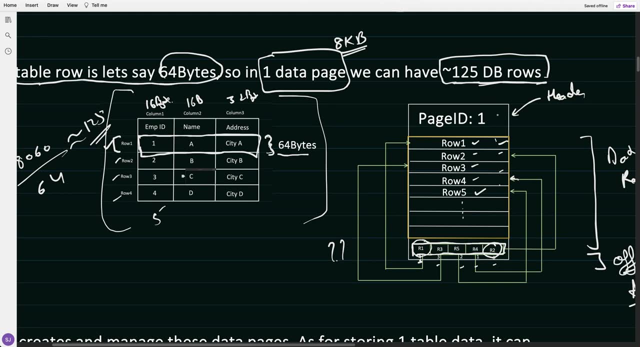 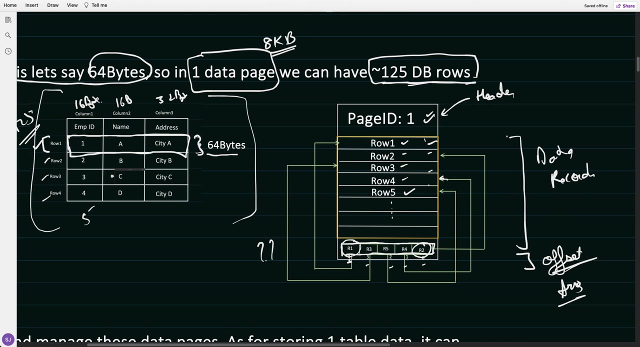 but now you should be clear with this that how your data is actually stored by our dbms. so this table is actually visible to you, but for dbms the way it is stored is like a data page, so for each page it gives a number and it stores the data in a page right in this data records area. 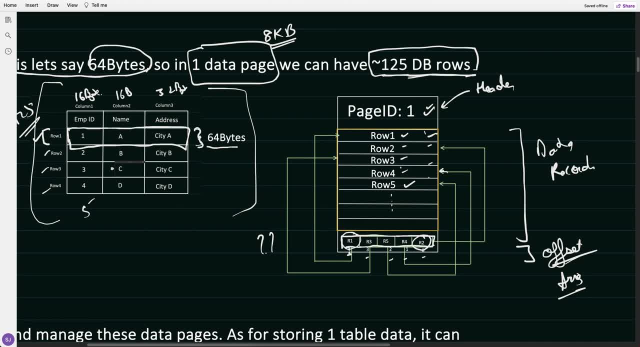 right, and for each this rows there is an offset. it also maintains the offset, also where it put a pointer and the ordering dbms will decide when we discuss about indexing. okay, till now it is clear, right, all these numbers, which i am saying is the number of rows that are stored in the data page. 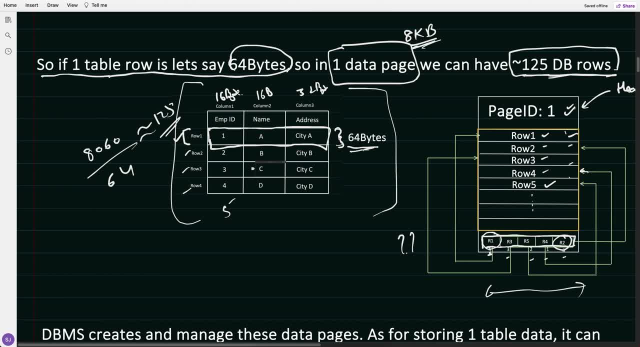 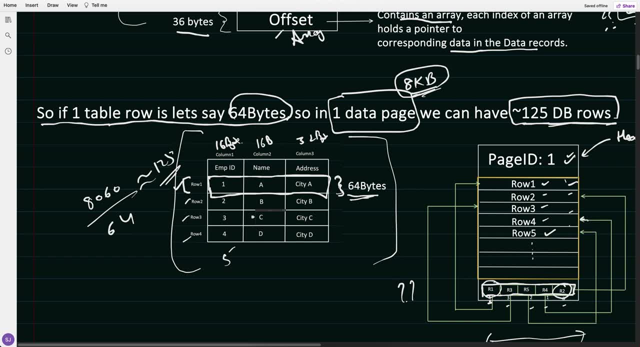 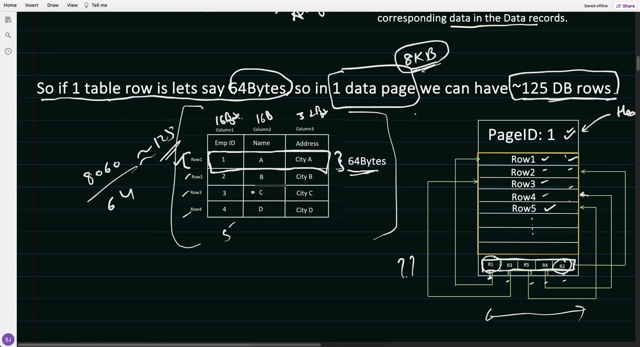 so, for example, if i am saying 8 kb, 8 kb, 64 bytes, that depends right, that depends upon db to db. so but for this one this is the most common. generally you will see data pages 8 by 8 kb. cool. so till now we 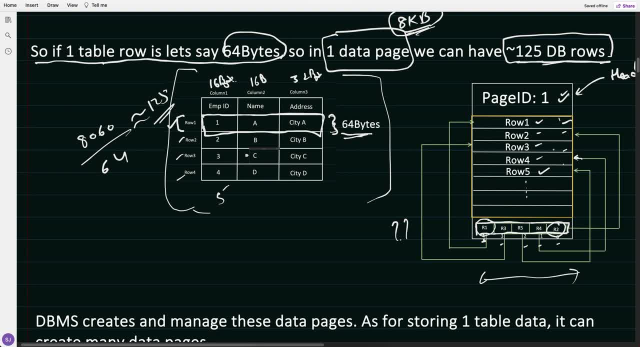 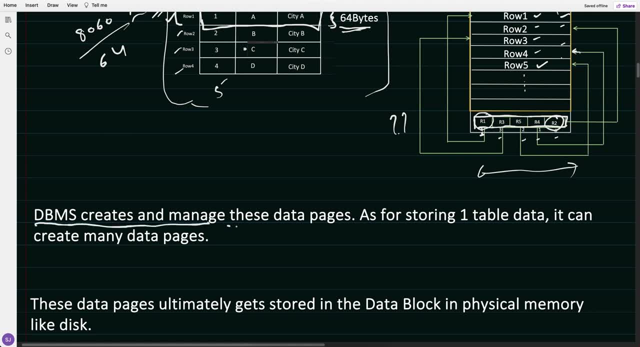 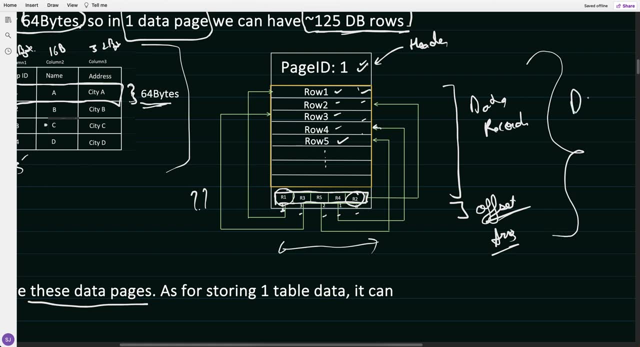 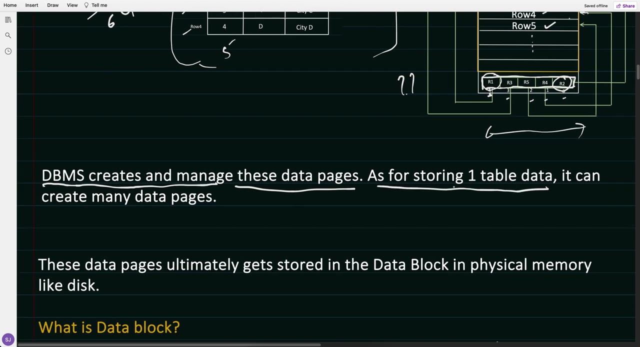 know that. okay, this table how it is represented in one page. so dbms: remember that dbms creates and manage this data page. so this pair, this page, whichever i we have talked, who manages dbms? so total control over the dbms. so for storing one table data, it can create many data pages. so now let's say, this table grows and it 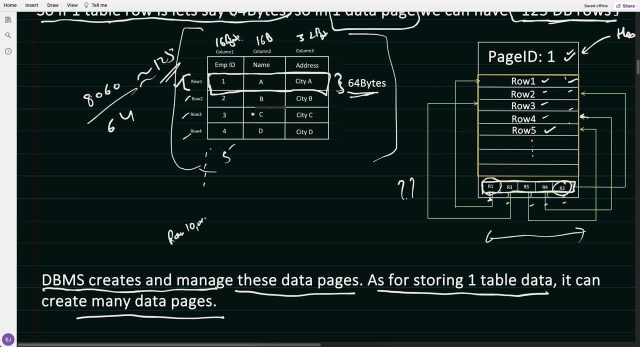 contains, let's say, row 10,000, like low 10,000. so definitely 10,000 rows cannot come into page 1, right? so it's upon dbms only to create a table. so, for example, if i want to create a table, i have to. 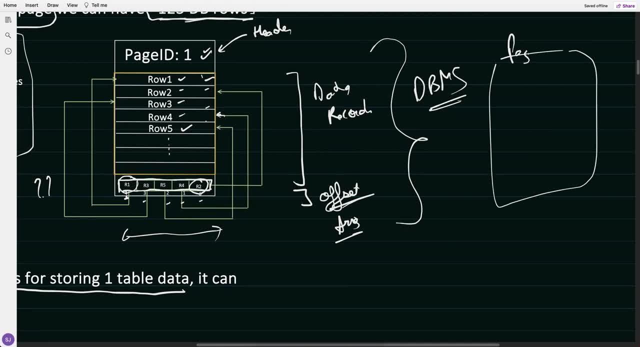 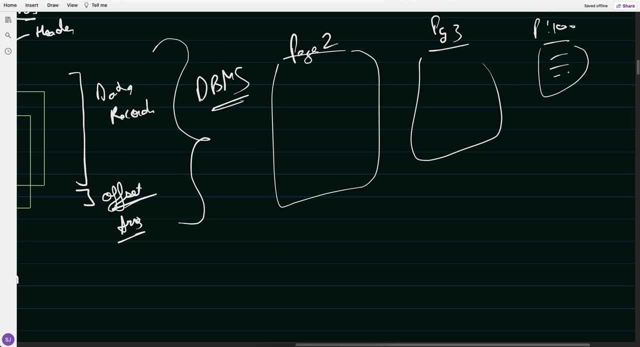 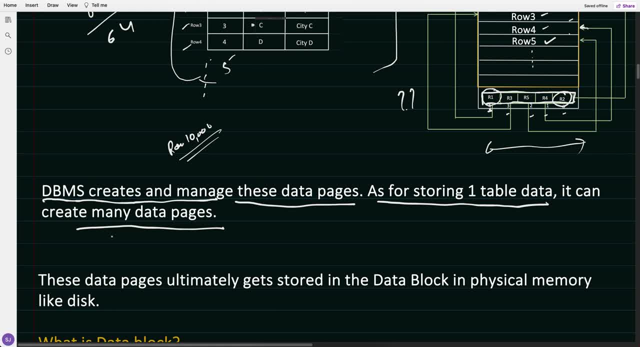 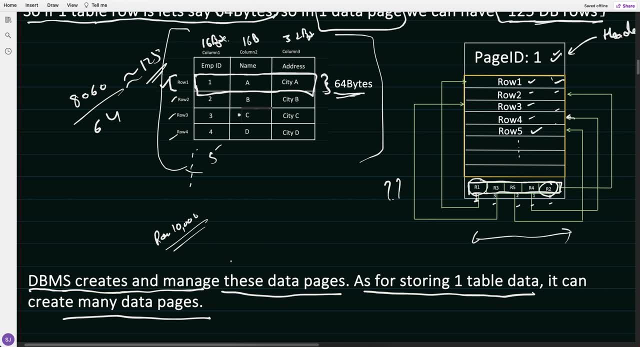 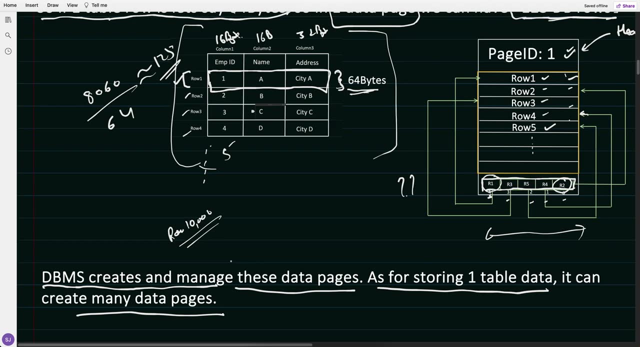 data pages and for storing one data table data, it can create many data pages. okay, i know that the very big questions come into your mind. hey, if there are hundreds of pages, if there are several views pages, how dbms gonna manage it? right, we will come to that one, but for now, for simplicity, 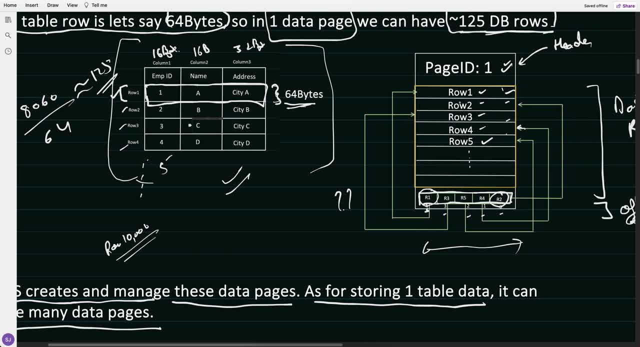 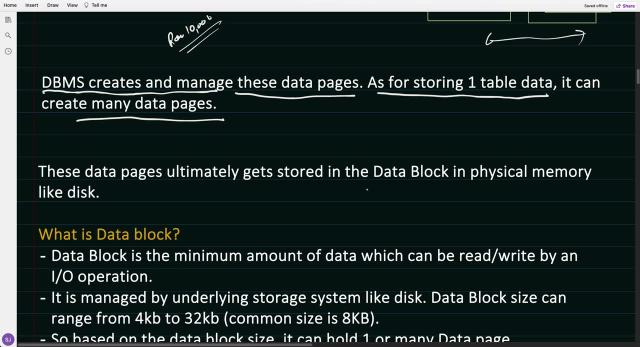 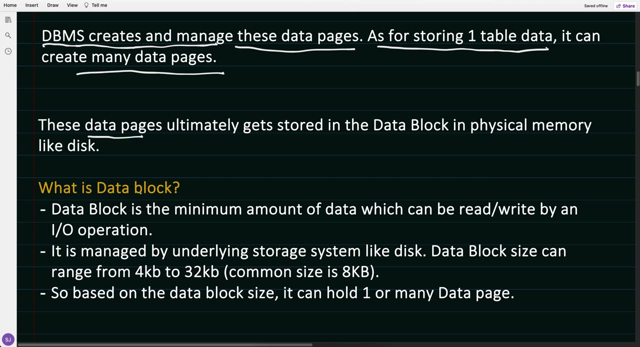 a table data is generally stored in a data page and one data page is full. dbms can create more data pages and keep on storing the table data till now very basics. we know now where these data pages ultimately get stored. these data pages ultimately get stored in the. 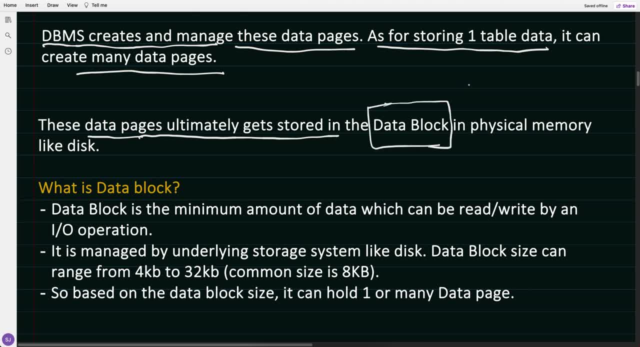 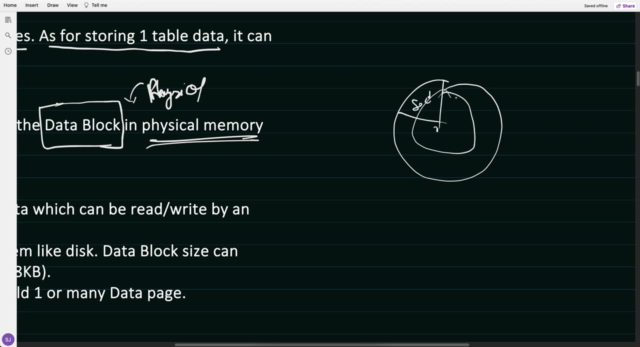 data block. now, this data block is actually a physical memory. this is actually a physical memory, right like this: on a disk there is a- so you know right- disk, and then there would be some sector track, so there would be one data block. you can say that data block. 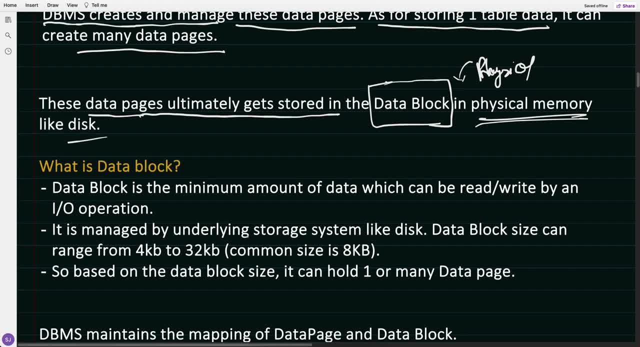 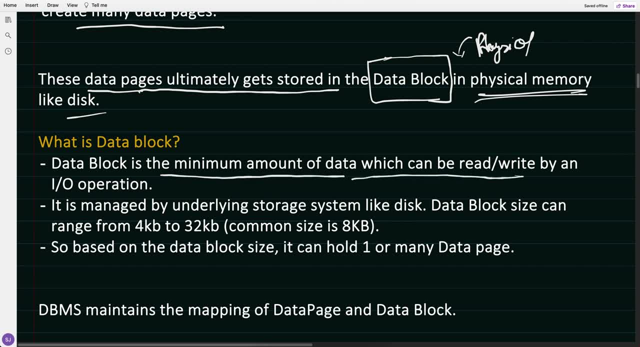 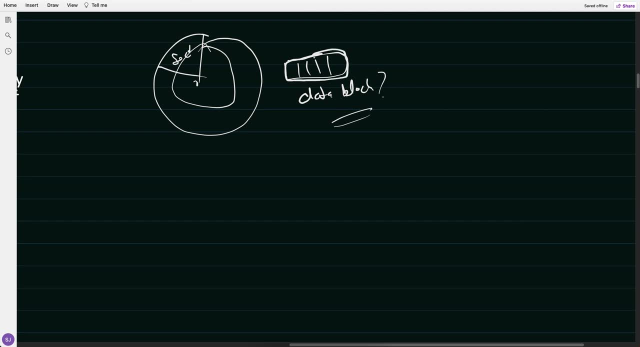 so what does data block means? first understand what is data block means. so data block is the minimum amount of data which can be read and write by one input output operation. so you can say that this is the minimum amount of data which one iu operation can read or write. right, so this is the minimum. 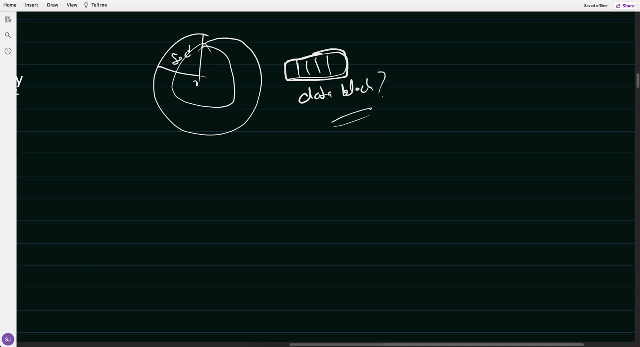 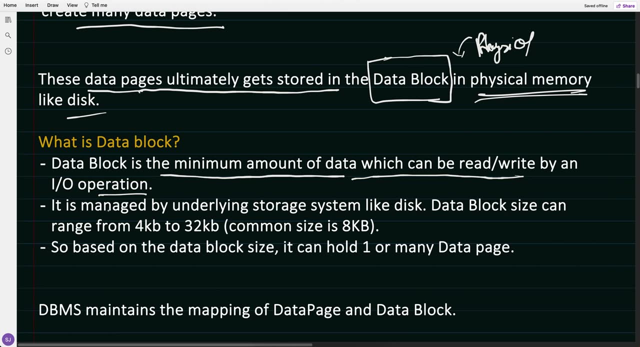 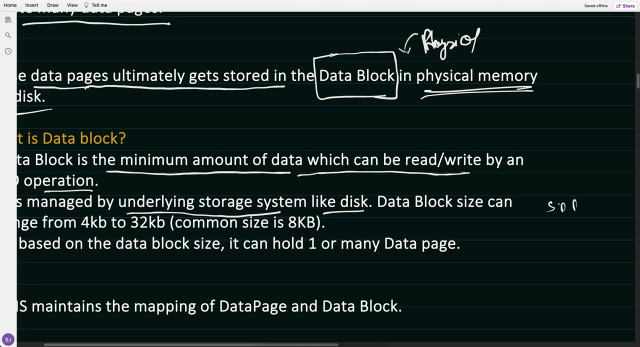 amount of data which you can fetch in a single shot, or which data blocks can have one iu operation. okay, and who managed this data block? it is managed by the underlying storage system, let's say like disk or sdd. let's say, if it has data block, so it is managed. 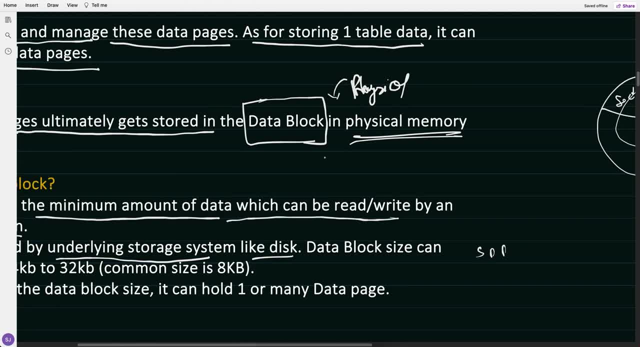 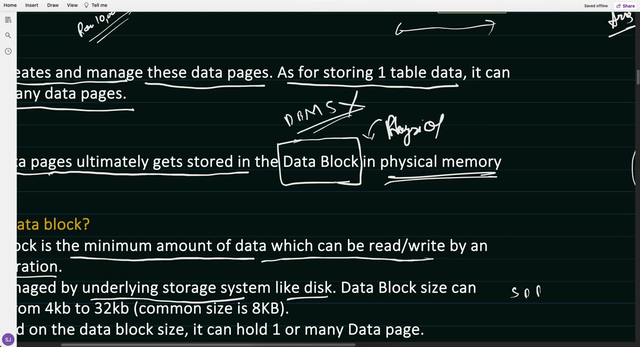 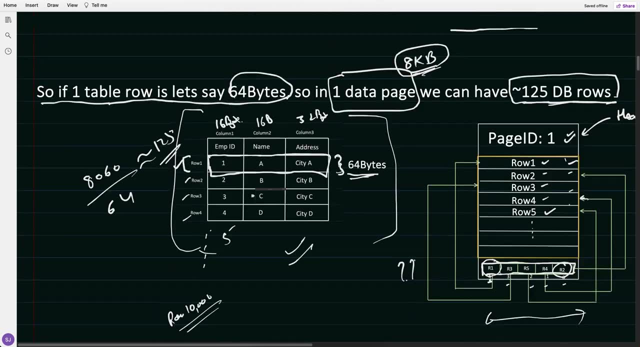 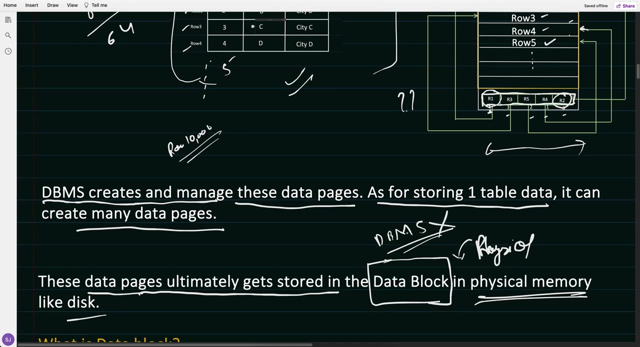 by storage system, underlying storage system. so remember that data block is not managed by dbms. it is not managed by dbms, it is managed by storage underlying storage system like this: data manage. dbms manage only data page, right. whatever the data you have, you have to put into somewhere into the memory, or 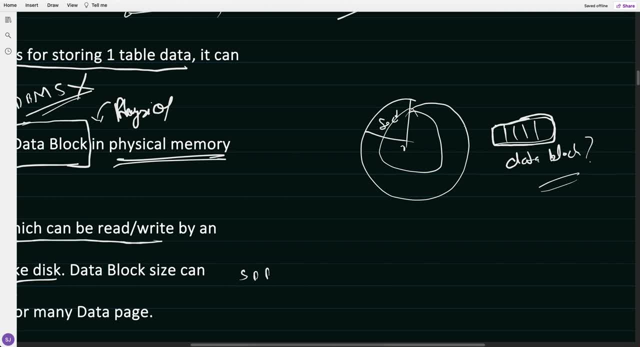 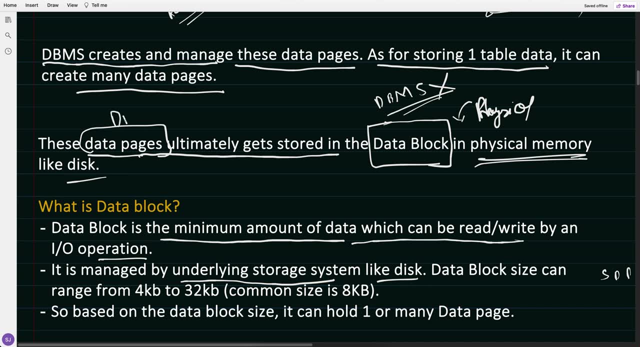 a disk right and inside a disk, what ultimately we have is data block. so these data pages which dbms creates, who creates it, which dbms creates, ultimately get stored where? inside a disk or inside a memory right inside a disk. so it is stored actually in the data blocks. 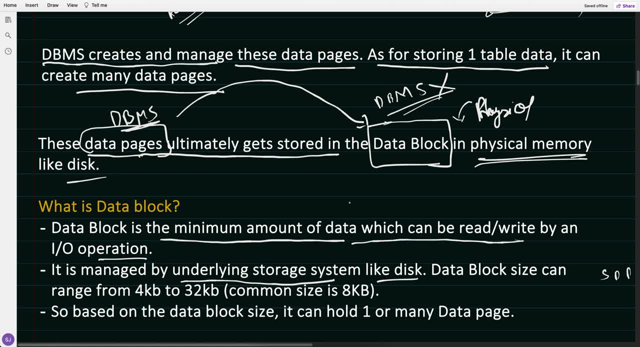 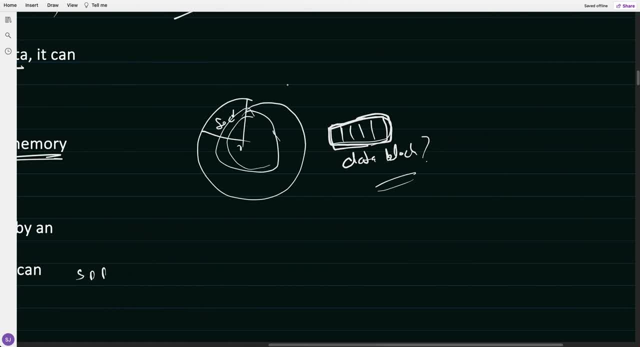 and dbms has no control over this data blocks, it can be scattered. so now let's say it. if this disk has thousands or millions of data blocks, let's say dbms has no control, that okay, my page one goes here in this data block. my page two, for example, it can go into this data block. data block, let's say 100. 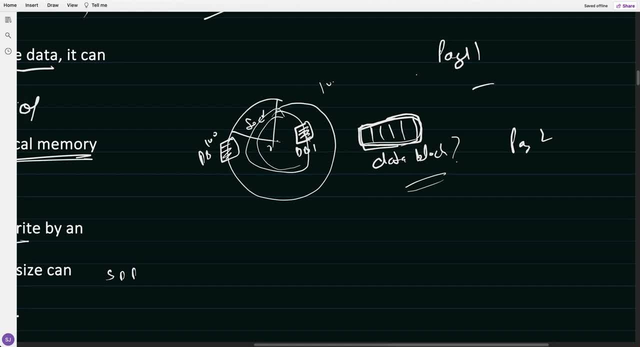 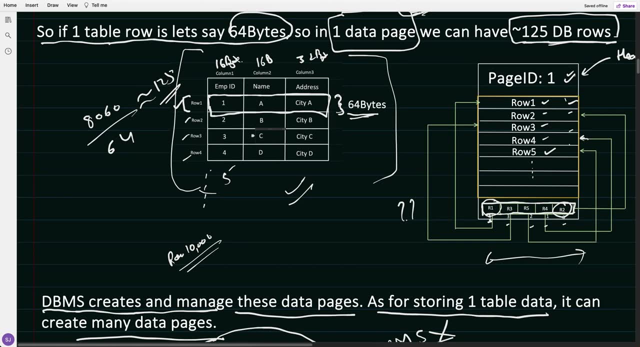 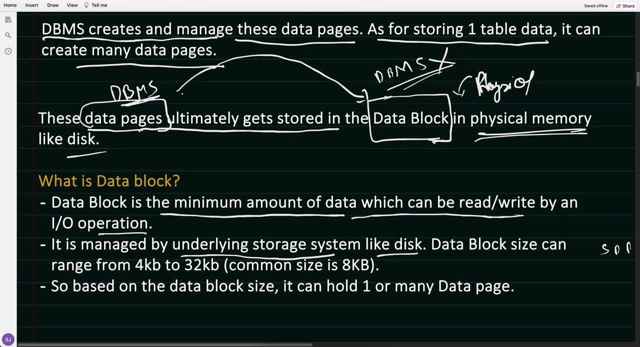 data block, let's say one. so what i'm trying to say is that dbms only has control till data pages. it can decide what data i can store into this, what rows i can store into a particular data page, right, but when it is writing to the d- uh, actual disk memory, right. 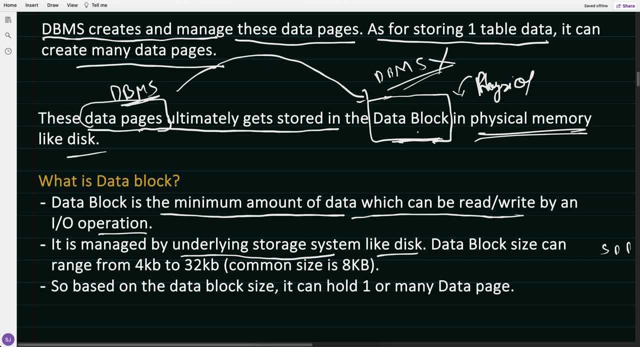 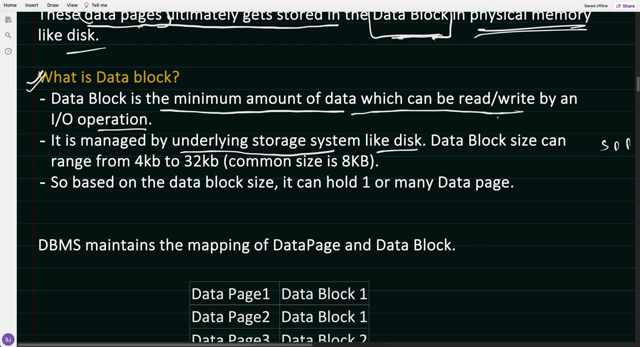 then it ultimately gets stored into a data block and it has no control over it. okay, so now you know what is data block? it is the minimum amount of data which can be read and write by an input output operation. so data block size can range from 4 kb to 32 kb, and most common size is 8 kb. so now 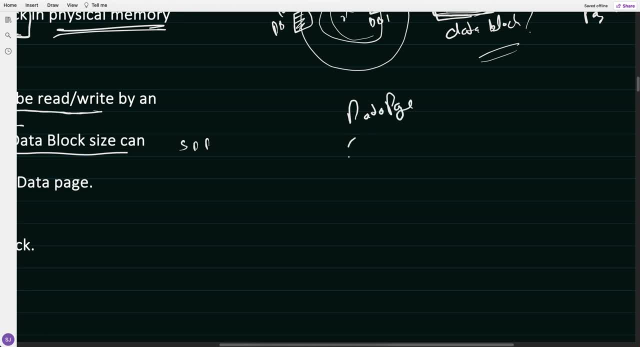 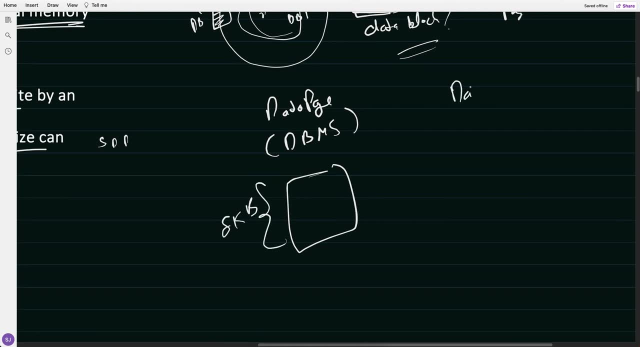 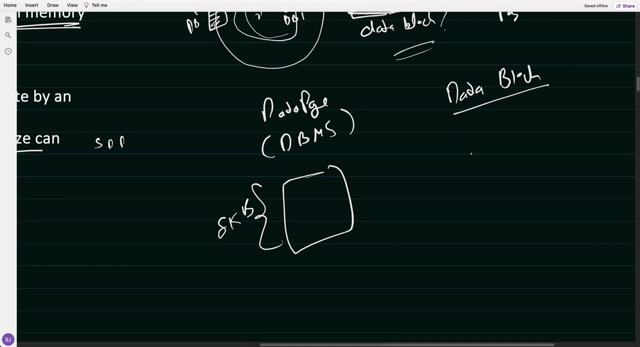 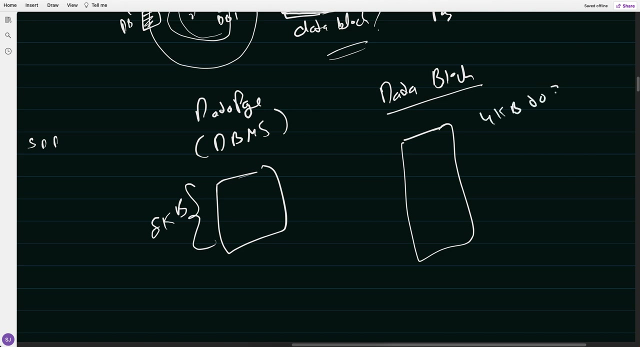 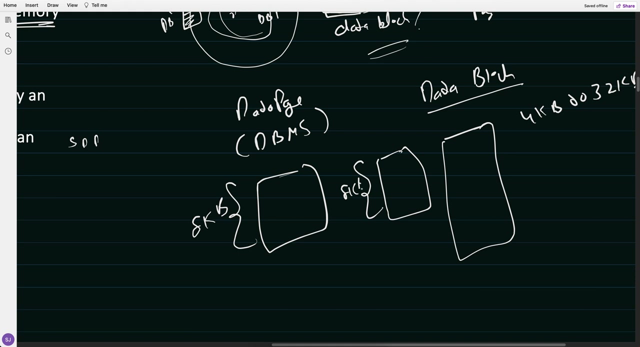 let's say your data page which dbms manage. it is of 8 kb data block which actually stores the data in the like a physical location. it range from 4 kb to 32 kb but most commonly you will find is also same like an 8 kb. so if it is 8 kb means one data block. one data block stores one data page only. 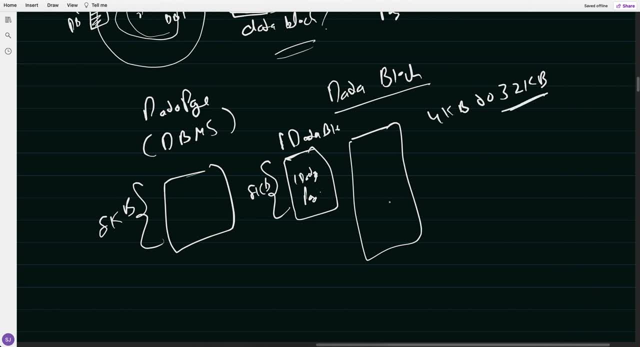 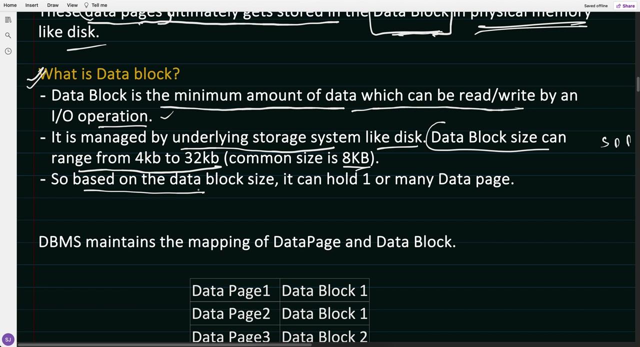 but if it is, let's say, 32 kb, then it can con store multiple data pages: data page one, data page two, data page three- right, so one data block itself can store multiple data pages. okay, so based on the data data block size, it can hold one or many data page. okay. 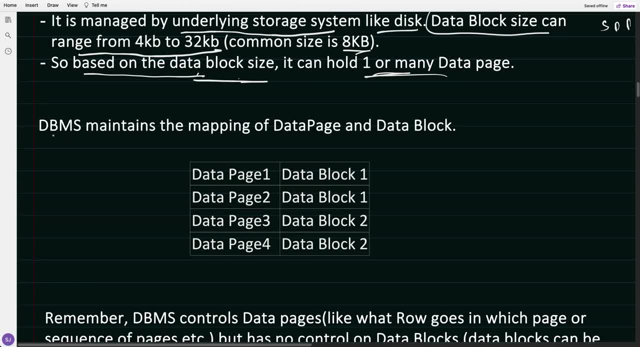 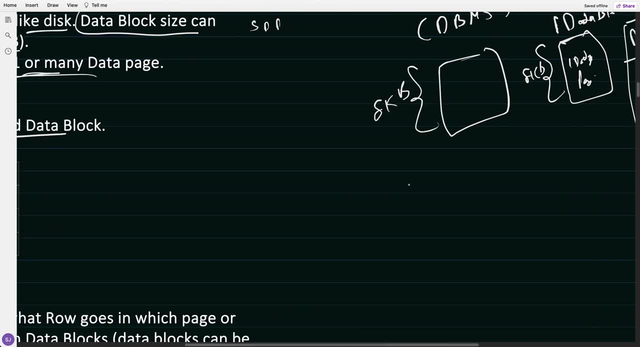 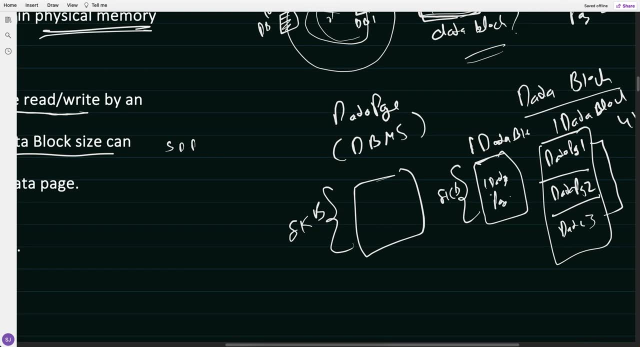 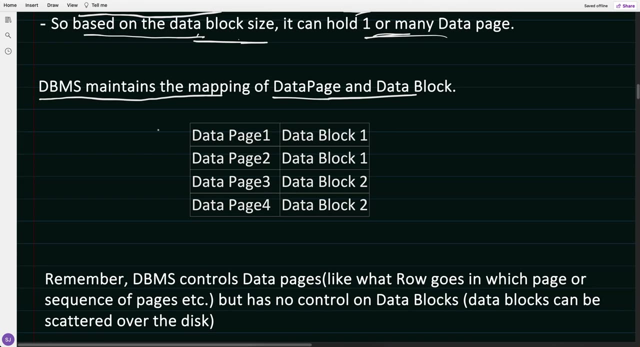 see here. what is that new filter item? so that's why i have named it dbms. okay, now there is one more thing is dbms maintains the mapping of the data page and data block, because i told you that dbms has no control over the data block, where this particular page, where my page, where the data page is stored. 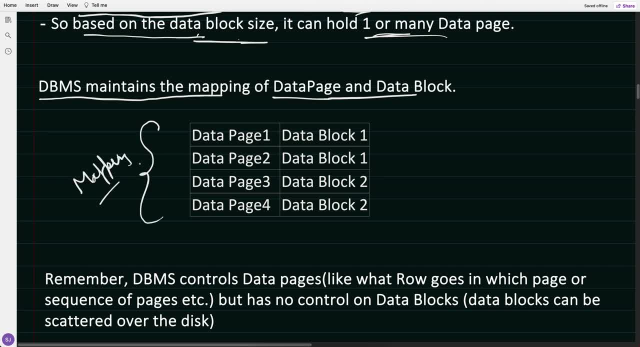 it has no control over it, so that's why it maintains a mapping. ok, maintains a mapping that. hey, data page 1 goes into this address, data block 1. data page 2 ultimately goes to this address, data block 1 itself. so it is possible that one data block- this is, let's say, data block 1- one data block can hold. 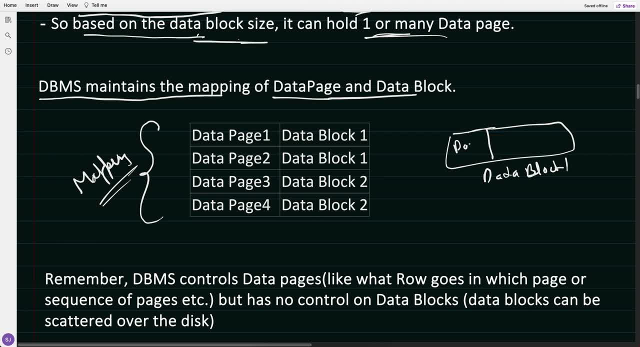 multiple pages. data page 1. data page 2. it's stored in the same data block because data block size can be higher than the data page, right? so DBMS maintains this mapping, that, okay, this my, my, my, this page, because DBMS maintain this page, right? okay, this page 1 is stored in this block. this page 2. 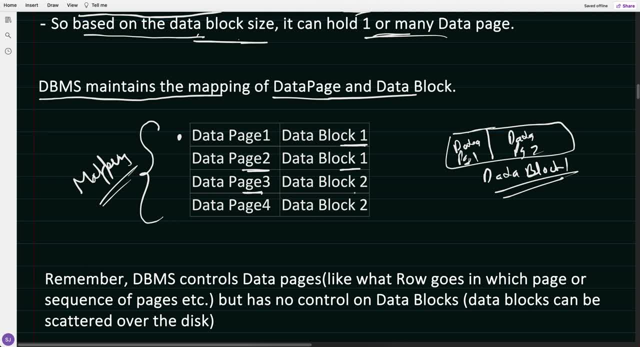 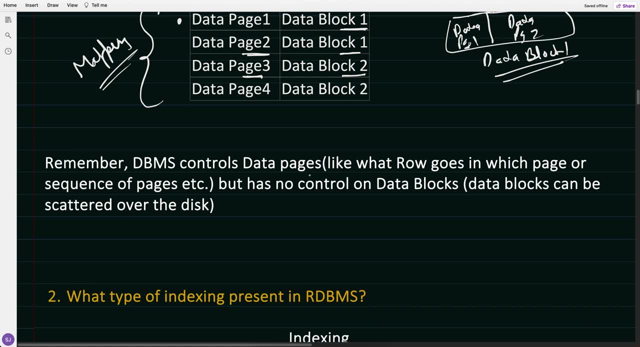 stored in this block. this page 3 is stored in this blog, right like this. so, remember, DBMS controls the data page, like what rows goes inside in which page, or sequence of the page, etc. but has no control on the data block. data block can be scattered over the disk, okay, so I think you should be clear with. 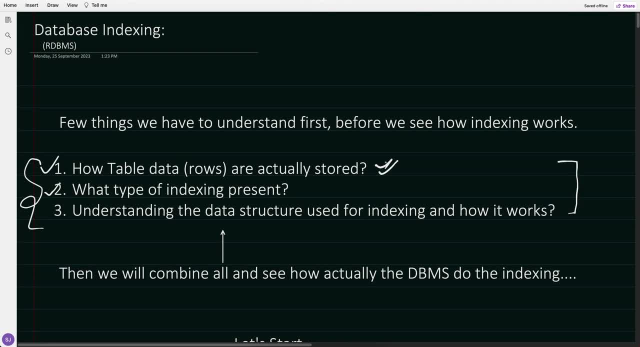 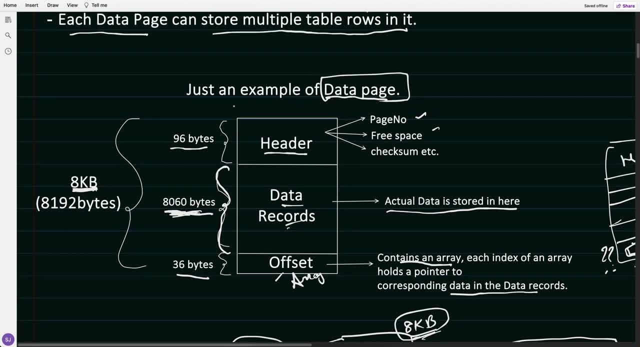 till now, though, first part, how the table data actually stored in the table data- извест을 수 있는 JOHNS- DB. So this is not, this is just a logical representation- The ultimately stored in a data page For one table there can. 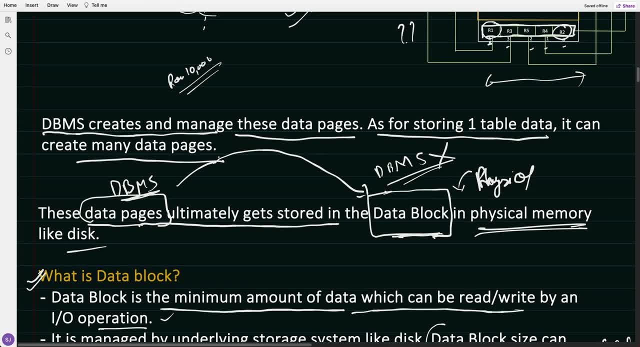 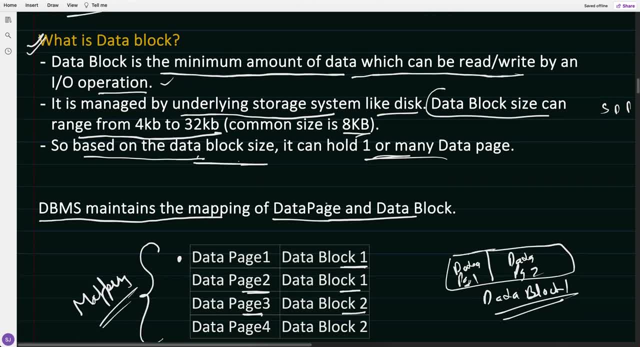 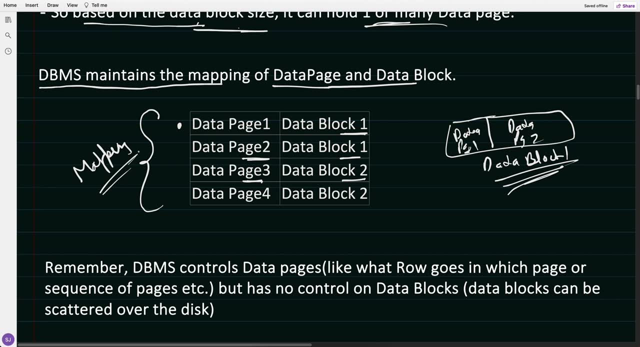 be so many data pages right, And each data page is stored in, ultimately, the physical memory of data block And one data block can hold many data pages right, And DBMS maintains the mapping also which page goes into which data block. Okay, 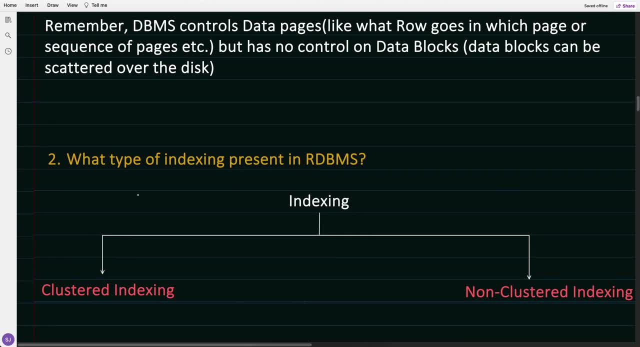 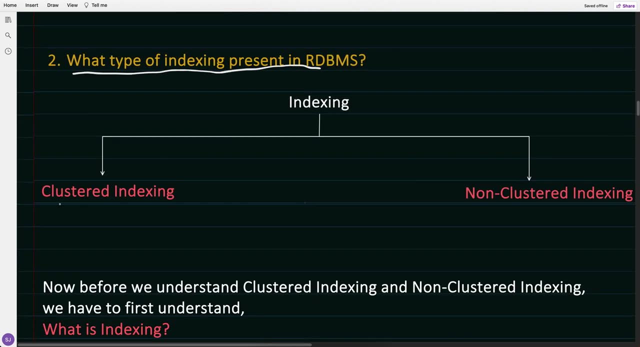 Till now we are clear. Now let's see the second part. What type of indexing present in our DBMS? Now here, if you see that the things become little, you can say that interesting. So this name you might have heard a lot: clustered indexing and non. 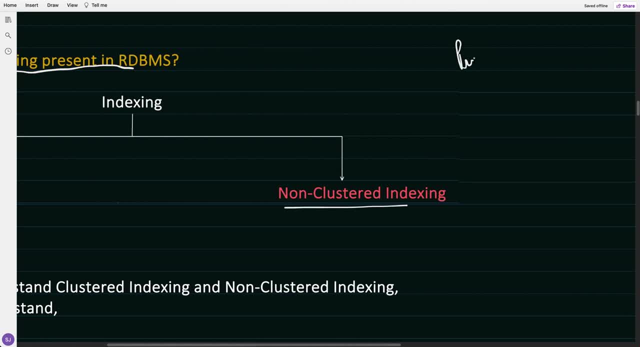 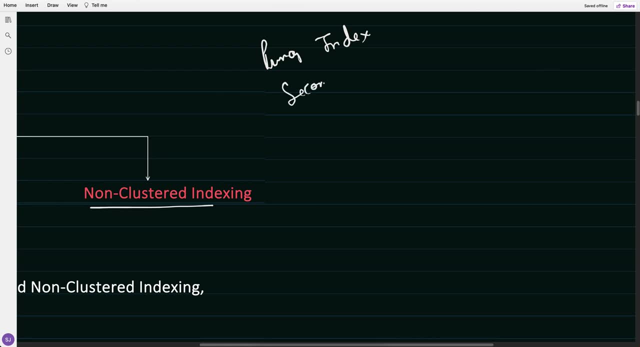 clustered indexing. I know the things which will be going into your mind: Primary index- as soon as you heard a name, indexing, it will be like primary index, secondary index And what is that? Composite index? like there would be so many indexing. So all these things should have. 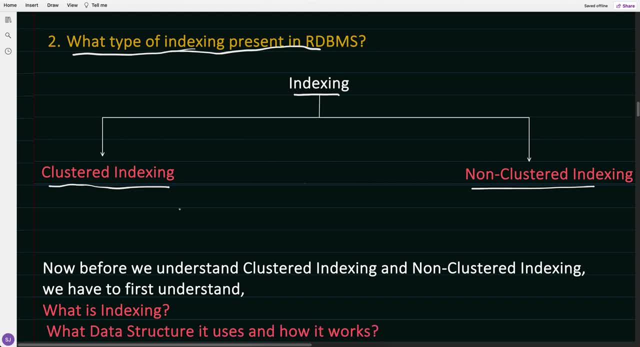 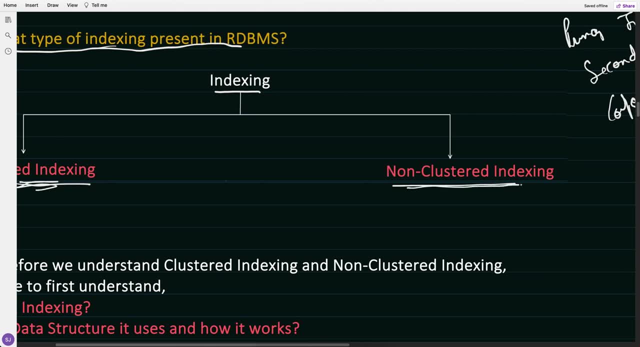 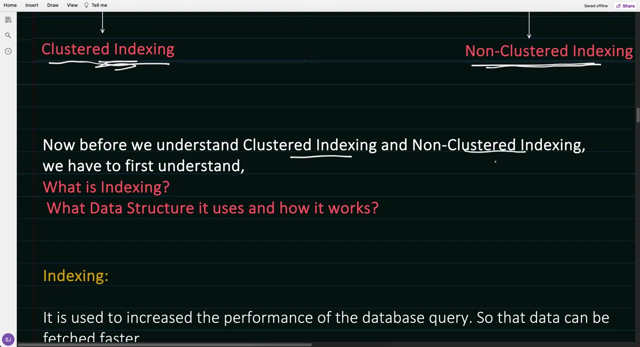 come in your mind, But from the indexing DBMS perceptive they are categorized into two type: clustered indexing, non clustered indexing. So forget about like before. we understand clustered indexing and non clustered indexing. First we have to understand what is indexing When we are saying indexing, indexing, indexing. but 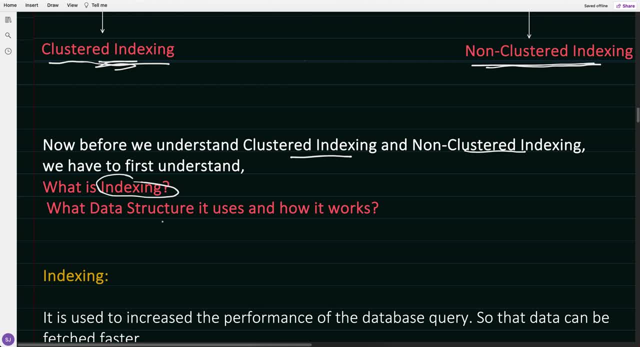 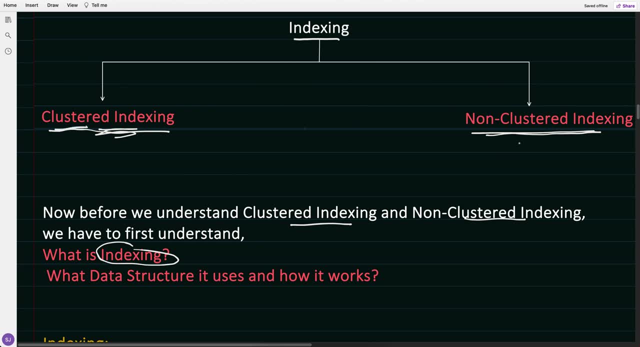 what does indexing means Right, What data structure is used for doing that indexing how it works? then we can come to that okay, cluster and non cluster. But first we have to better understand what indexing is, how it is done. 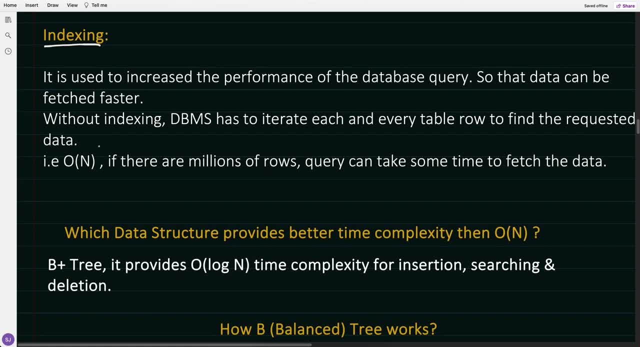 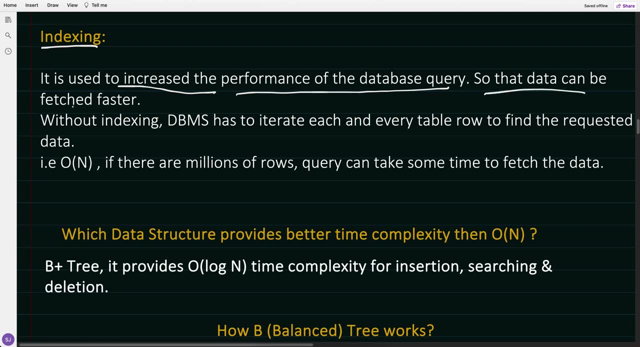 So, in a simple term, if I say that what indexing is, it is used to increase the performance of the database query so that data can be fetched faster. Okay, so indexing is just nothing but doing to increase the performance of the query. so 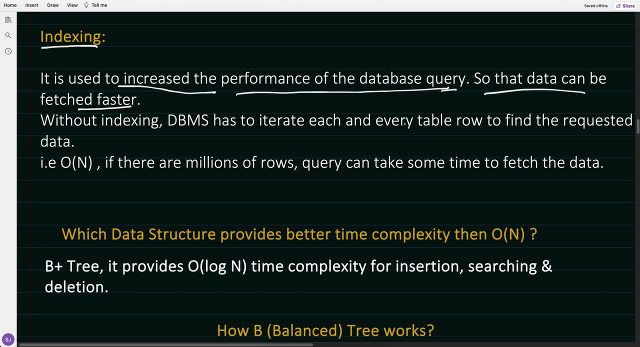 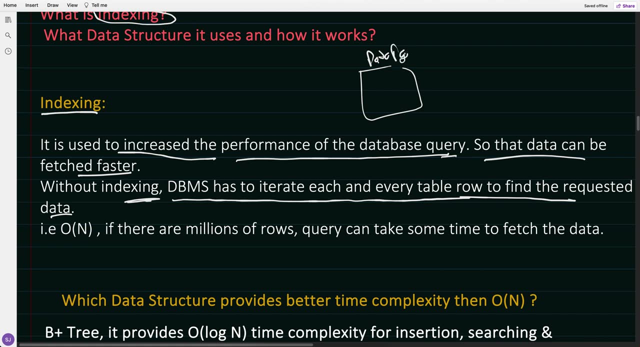 that it helps us to find the data much faster Without indexing. DBMS has to iterate each and every table row To find the requested data, So you know that it maintain the data pages, data page one. let's say there are 1000 data pages. 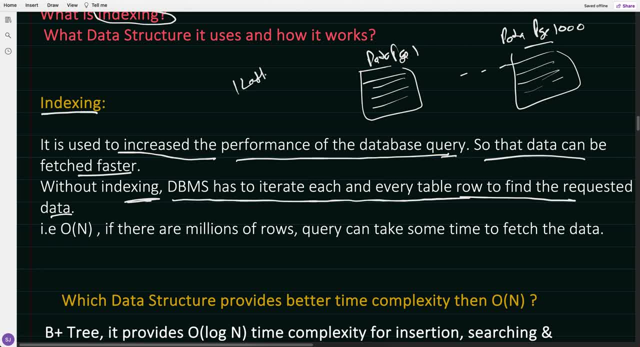 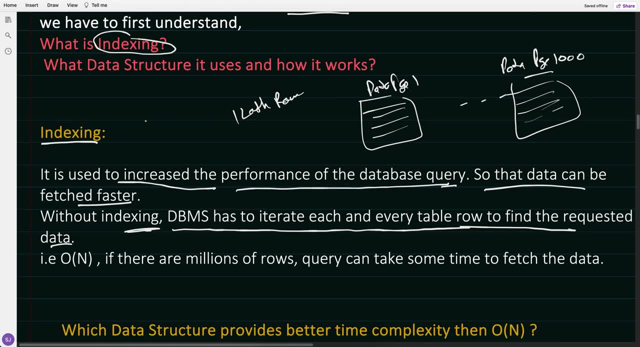 Inside this 1000 data pages, there are, let's say, one lakh rows data. right Now, if you have to find something, that Hey, give me a data with employee ID. Okay. Okay, ID 35.. Now, DBMS doesn't know that which this employee 35 record. 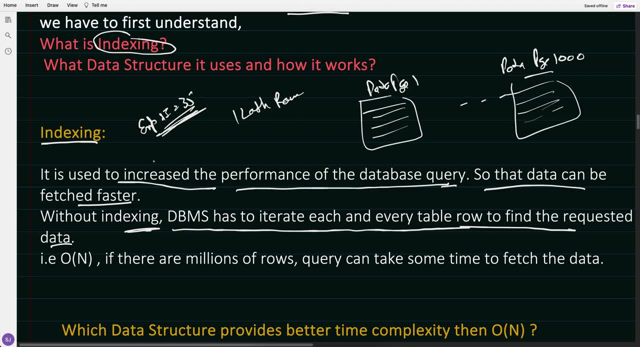 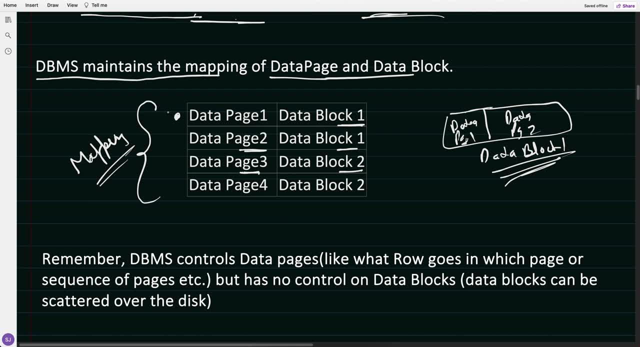 goes into which data page it doesn't know. All DBMS has till now is indexing. Okay, this data page is goes into this block. So what it can do is that in a worst case, it will iterate over this mapping. Okay, my page one. it will go to this physical. 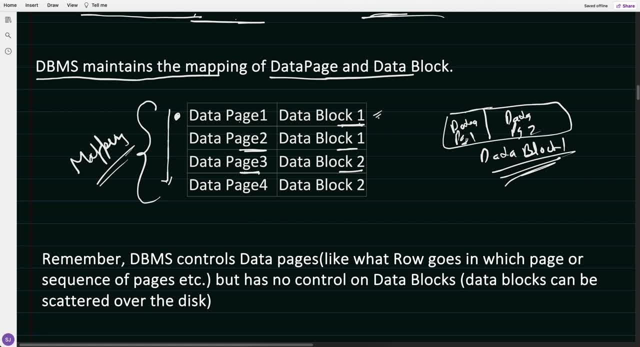 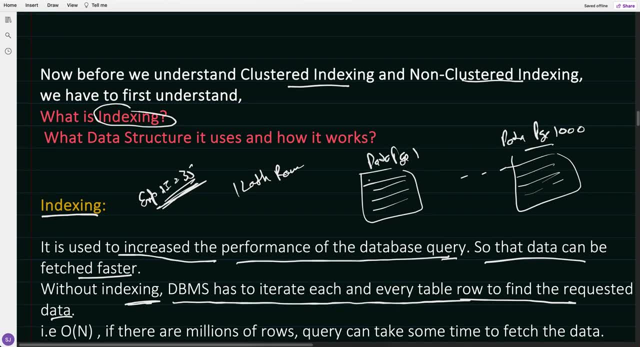 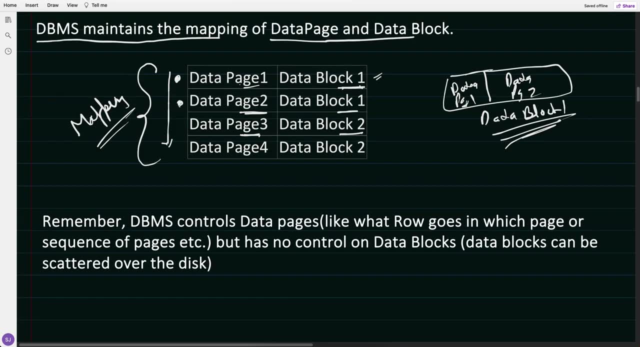 memory row. load the data. load this block into the main memory. take out the rows. read this page And see it. read this page and see that. Hey, does employee ID 35 present? No, if it is no, it goes to the second one. Okay, my page two is store. 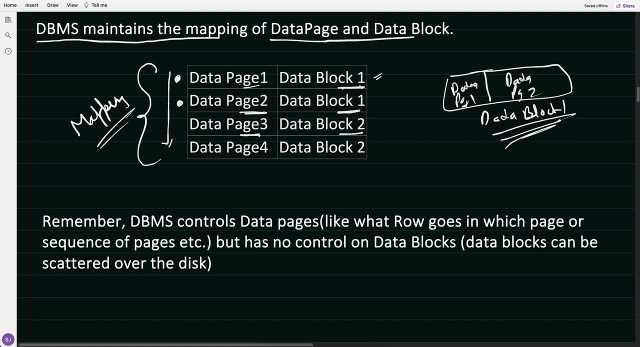 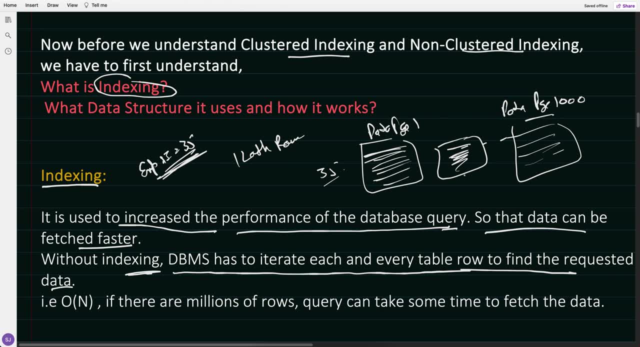 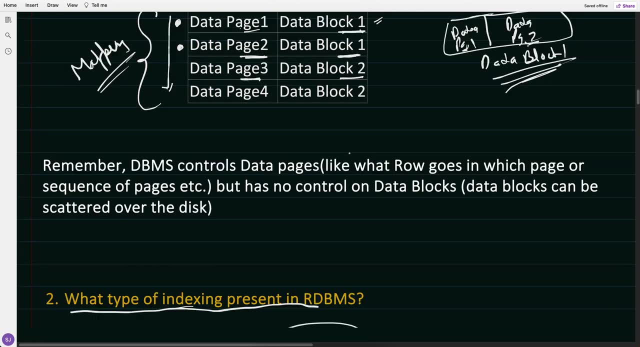 is in this block again. So it is already in memory. So it will load that page, page two, Right, And then it will again. it's page two. it will check all its rows. Hey, have I found this employee ID 35 or not? Let's say, for example, worst case, this employee. 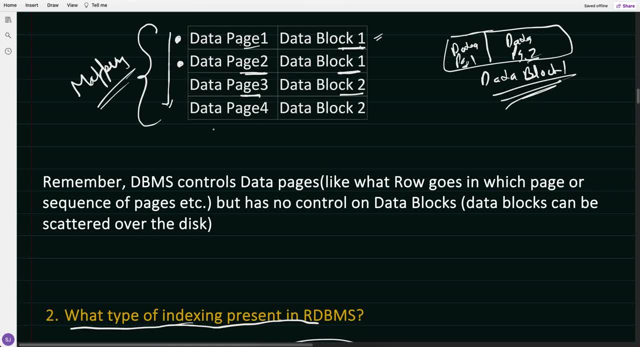 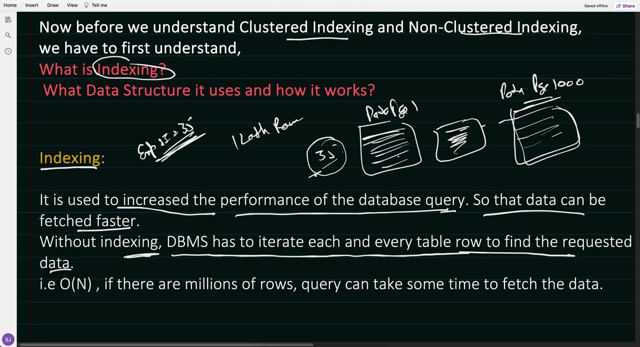 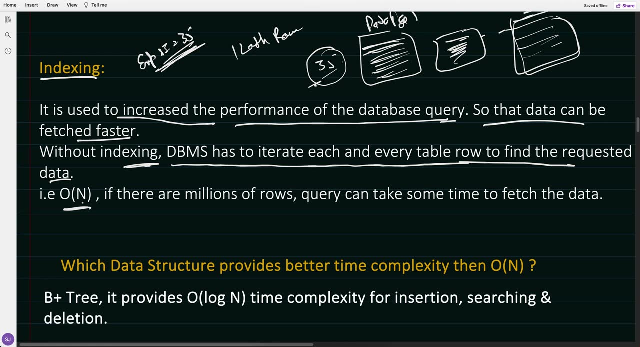 is present in the last data page, the last mapping which is present here, then it has to iterate over all the data pages and inside all the data pages it has to iterate over all the rows. So what is the worst time, complexity big go off in. So 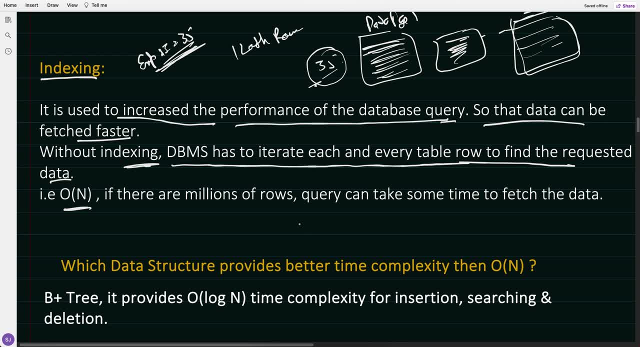 without indexing. it has to check each and every row Right and if there are, let's say, millions of rows, then query can take some time to fetch the data Right Because it has to go to that particular data block from the mapping. 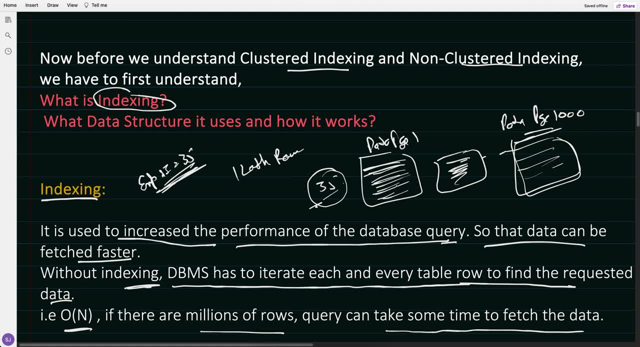 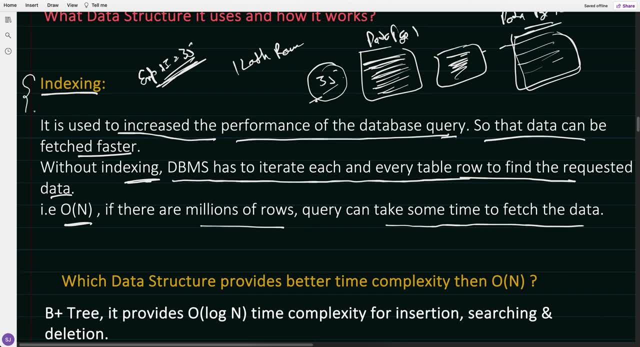 fetch the data, load into the memory, read the data page, take out its rows and then read it and see. So we know that indexing is used to make the query run faster. Without it, it would be big go off n, But with it, what would be the? 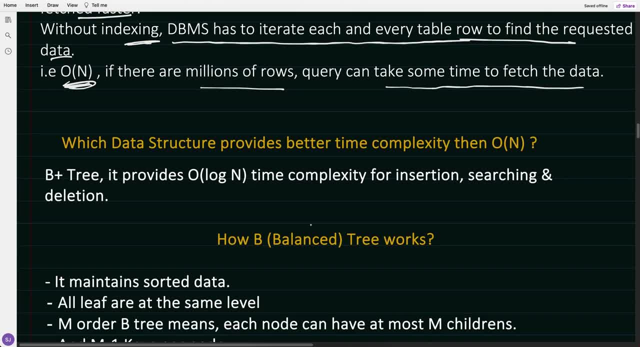 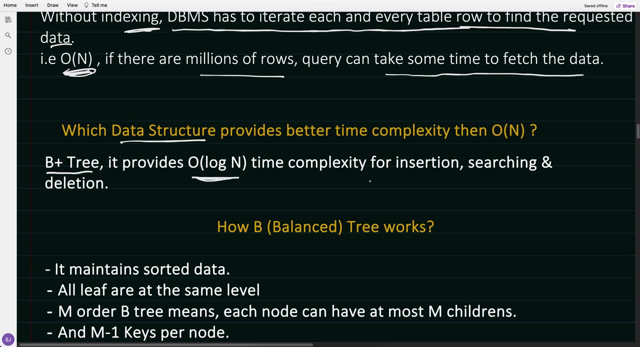 best time complexity we can give. So there is a data structure which is used which is known as B plus three. it provide big go off log n time complexity for insertion, searching and deletion. So this is very, very frequently used: B plus three. 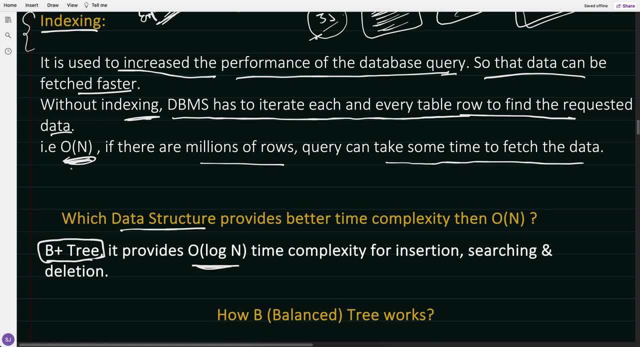 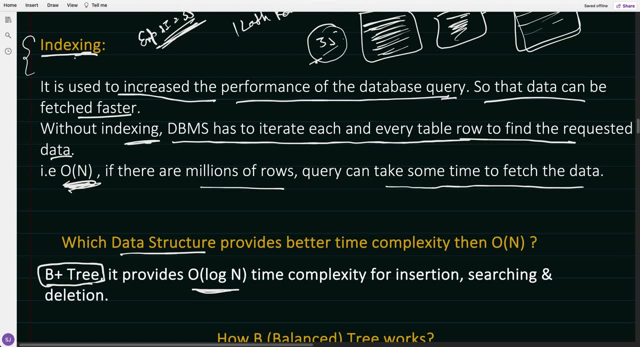 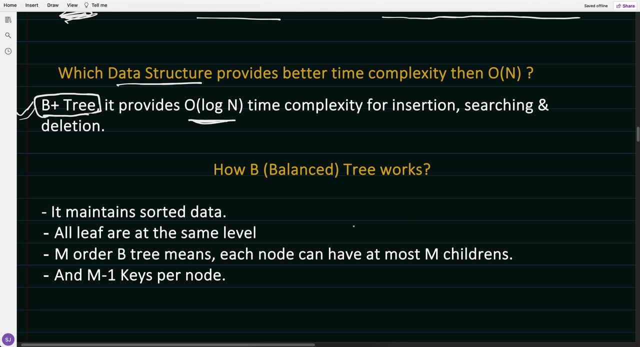 while for doing the indexing right. So without indexing, big go off. n is the time, complexity- to search any data inside a table With indexing. our purpose is to make our searching faster. and which data structure it use? it uses B plus three right, So B here is stand for. 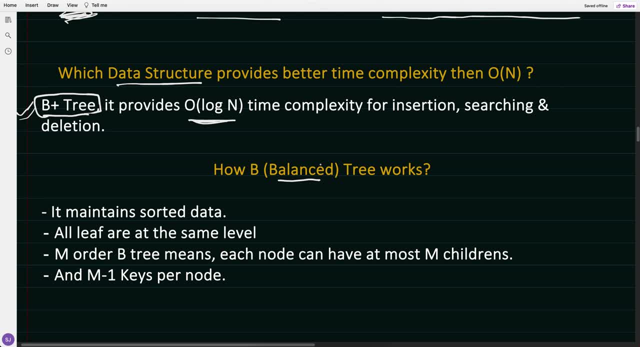 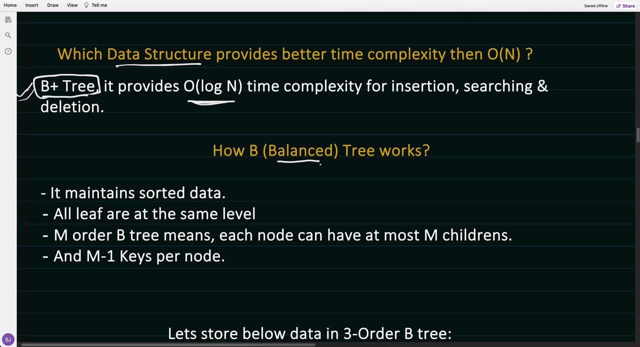 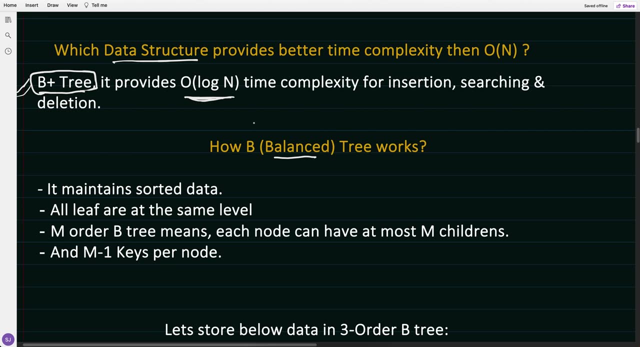 balanced actually. So now till now, we are slowly understanding, okay, what indexing is and for making the indexing works, what data structure is used. B plus three, it provide a big go of log n time complexity. So before I go further into the 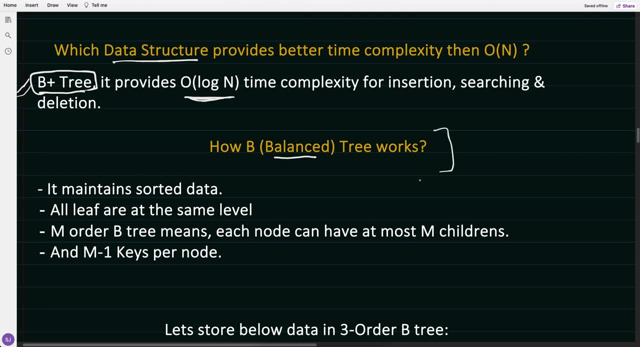 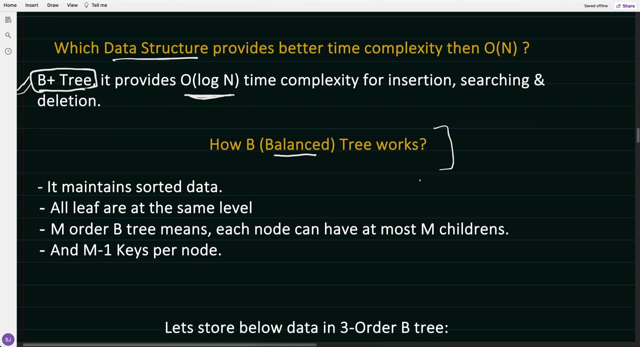 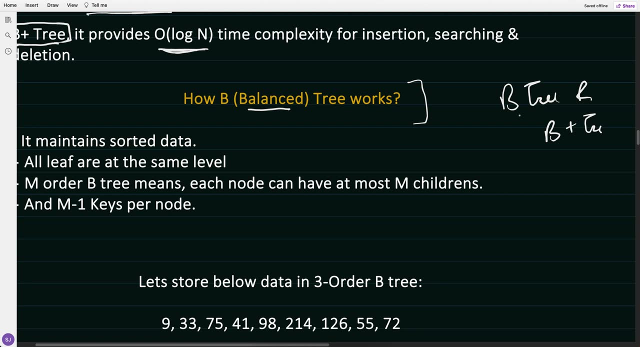 cluster, non cluster index. let's first see how B three works. it will clear your mind actually how this data indexing works. So I'll talk about B three. So B three and B plus three is very, very similar, Right? So if you understand B, 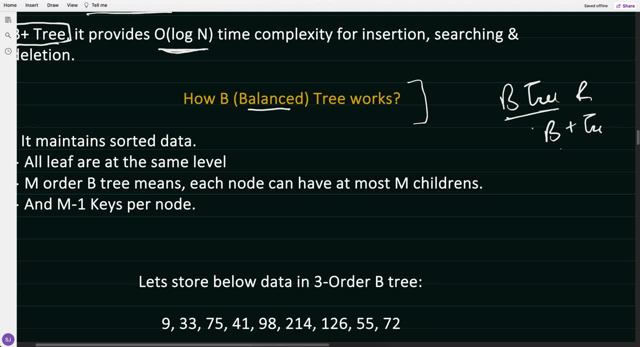 three. B plus three is somewhere near to exactly same. Okay, so now I'm saying B three And at last I will say that it gets a B plus three how it adds a certain additional feature, but both are exactly same. So I'm. 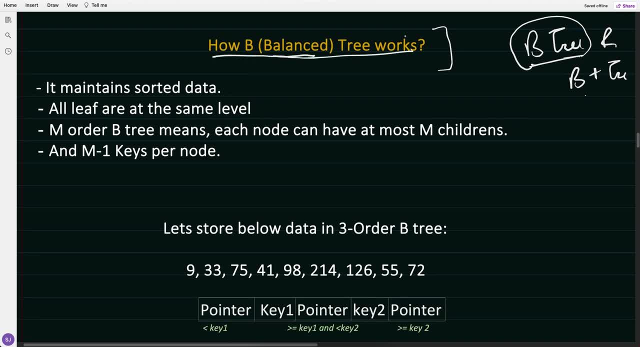 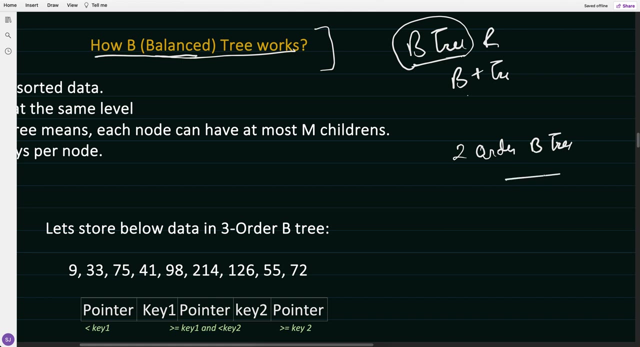 just telling you how B three works. So it maintains the sorted data. Okay, all leaves are at the same level. M order B three means each node can have at most m children's. For example, two order B tree means each node can have at most m children's. 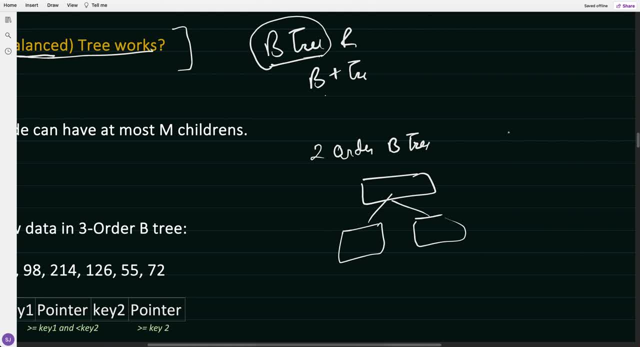 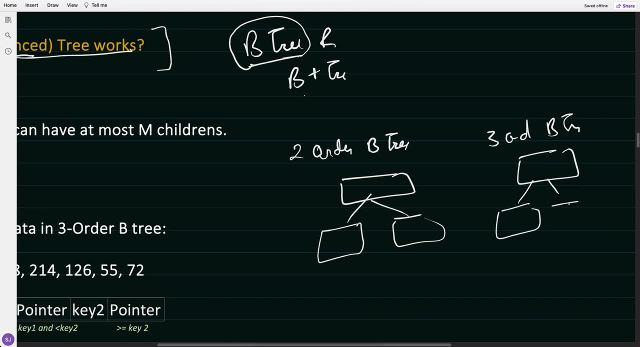 Okay, all leaves are at the same level. So it maintains the ordered data. Okay, all leaves are at the same level. So each node and the node can have at most two children Three order B. three means each node can have at most three children, Right You? 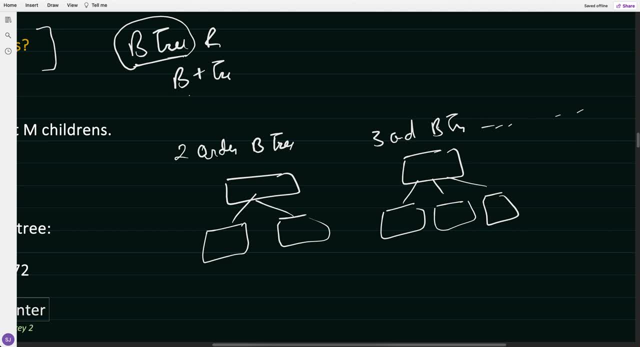 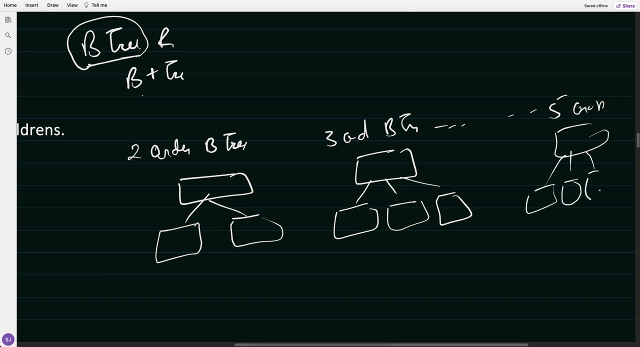 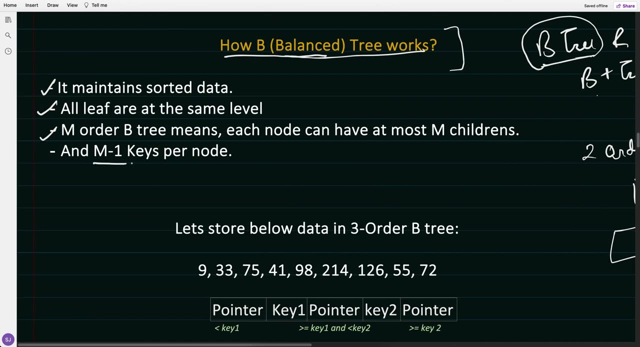 can have any number of this: m m order, So you can have, let's say, five order B. three means you can have at most five children, Okay, And m-1 keys per node. So now here, if you see that, When I say that, 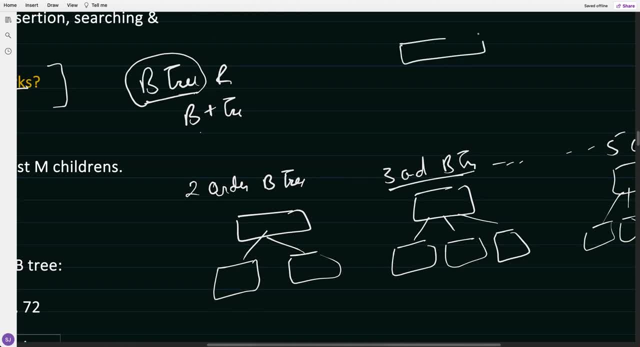 Let's say 3 order B tree. So let's say this is the 3 order B tree, So it can have 3 children. So in one node, So in the 3 order B tree, A one node can have 3-1. 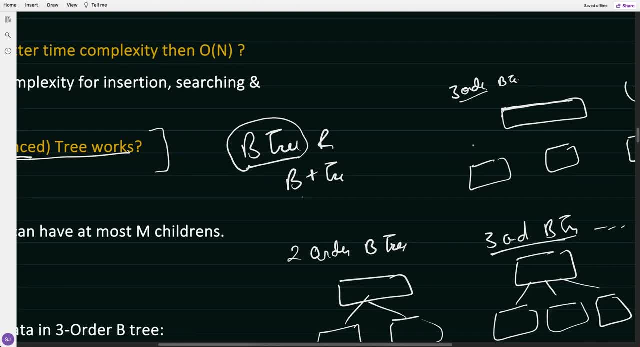 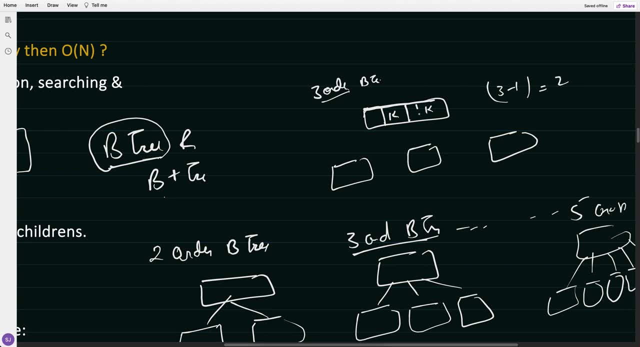 m-1 keys Right. So 3-1: 2.. So it will have one key here, One key here Right and it will have pointers here. So this is a pointer, This is a pointer, This is a pointer. 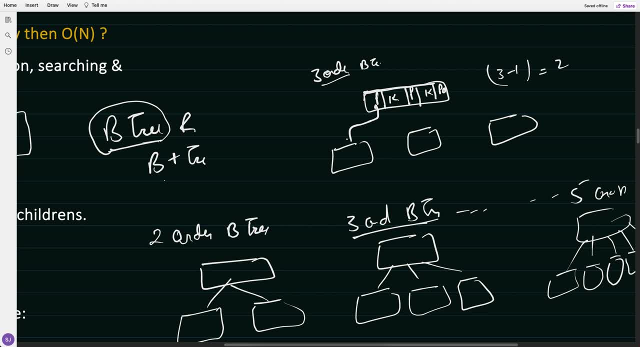 So this pointer will point to this child node. Let's say: this is key 1.. This pointer will point to this pointer, Child node 2.. And let's say: this is key 2.. And this pointer will Point to this one. 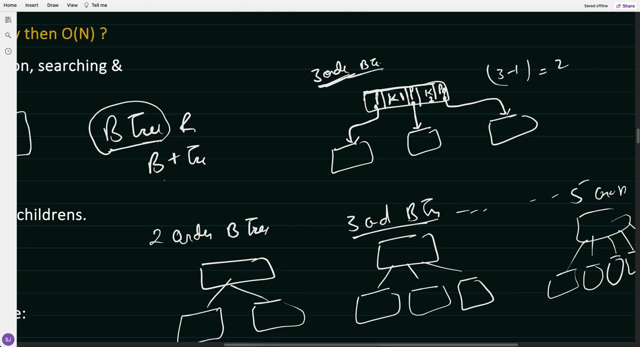 So in one node, If in 3 order B tree You can maximum have m-1, so 3-1, 2 keys Here And 3 pointers, And each 3 pointers can point to a child. So now you can say that, hey, what this 3 pointers generally signifies. 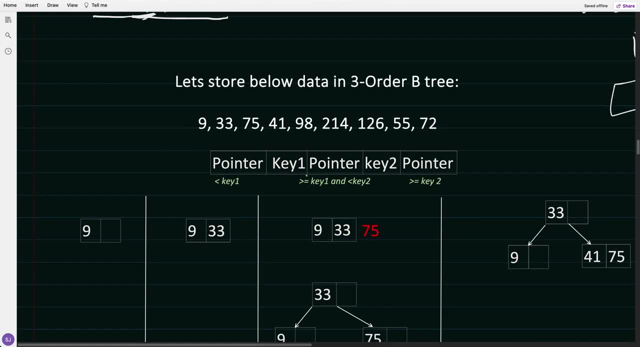 So let's see. that will come to that part. So now let's say that I'll totally show an example. However, it will become total clear. Let's store the below data in a 3 order B tree. So 3 order B tree means: 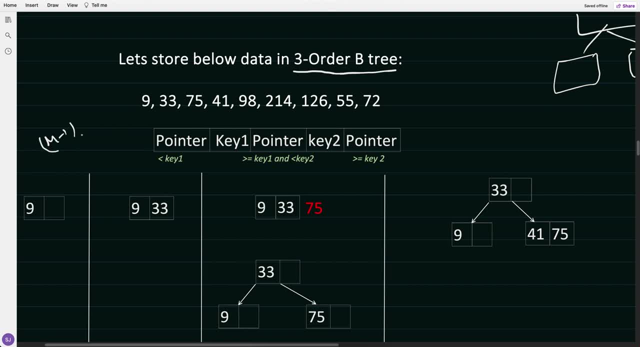 It will have how many keys: m-1, 3-1, 2 keys. So I have here key 1., Key 1. And key 2. And it will have three pointers: Pointer 1., Pointer 2., Pointer 3.. 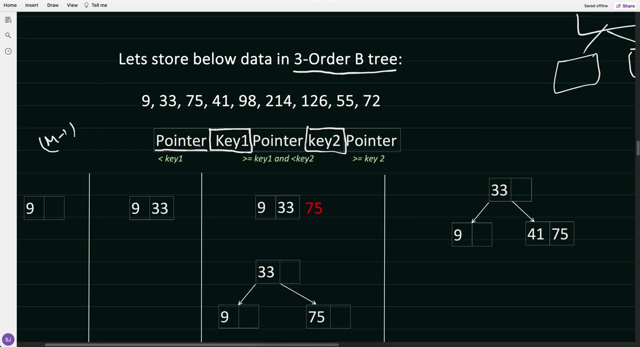 So now here, if you see that this pointer one, left one, So left one- is like always point to the child node which is less than this key, Less than this key. and the right one is like greater than equals to this one. So this pointer one will be, whatever the child it will point to, all its data would be less than this key. 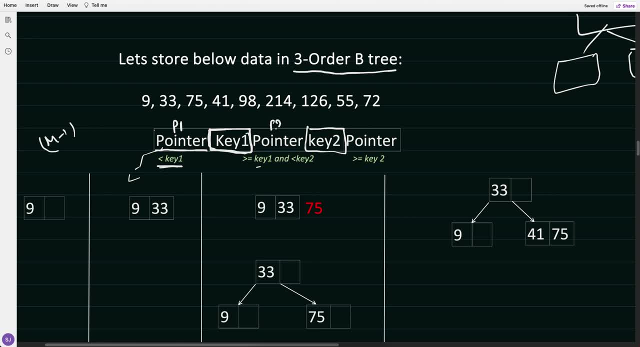 And whatever this pointer to which is on the right side of this key, whatever the child it will point to, ultimately all its data could be greater than equals to this key Right. So similarly, for this key to this pointer to is it's at left side. 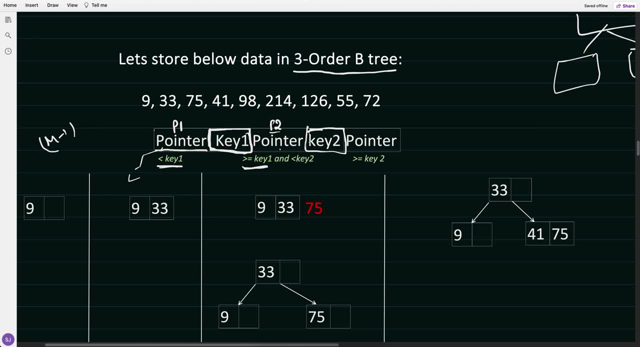 So, whatever the child it will point to, it will have a data less than key to only- and this pointer will have a- whatever the child it will point to, it will have data Greater than equals to Right. So that's why here we have two keys, three pointers. 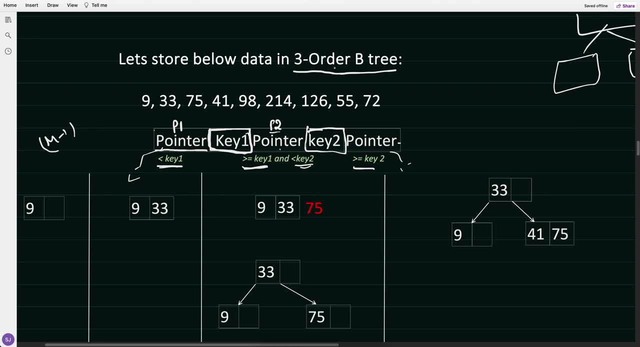 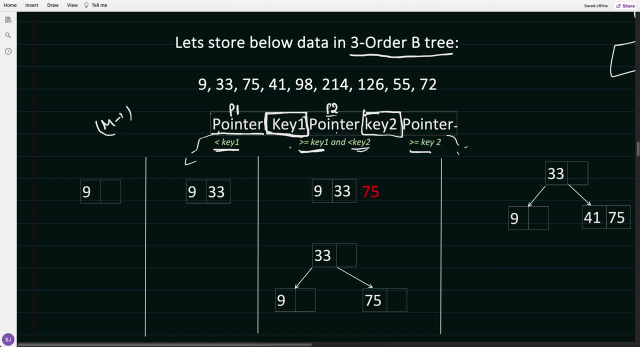 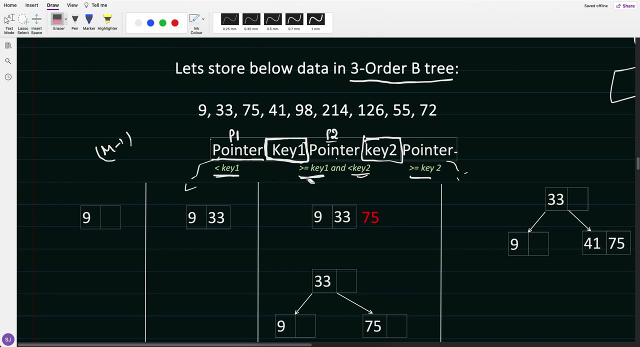 So that's how one node can have three childs. That's why the three order maximum three child you can have Right now. let's see an example. Let's understand with an example. It would be super clear. So don't worry about till now what we have understand about this DB, right pages and all. 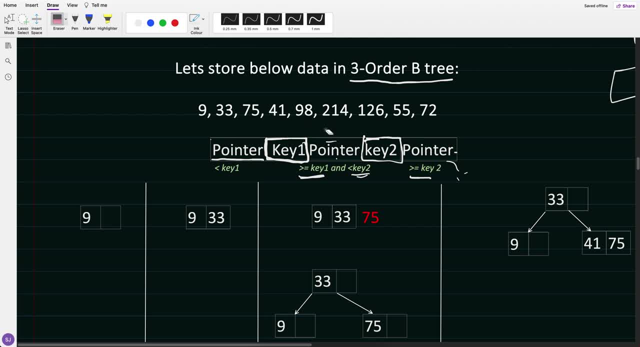 So we will come back to again and everything will start making the dots clear. but keep that till in your back of your mind that whatever we have is known till now. Okay, So now let's say we want to store this data into a b-tree. 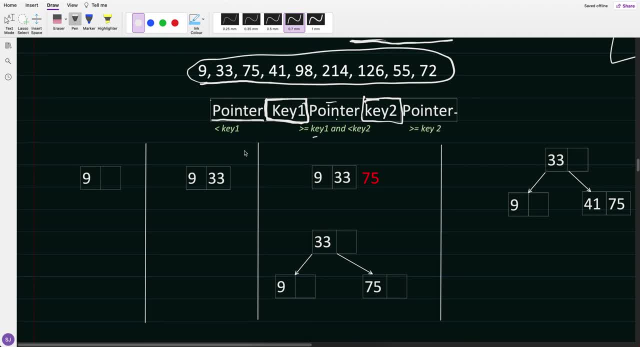 Okay, so I am using a three order b-tree. Okay, so how many? so understand this? this line is a pointer, Let's say this is one pointer to pointer. and third three pointer: Enter and two nodes and minus one node, So two nodes. 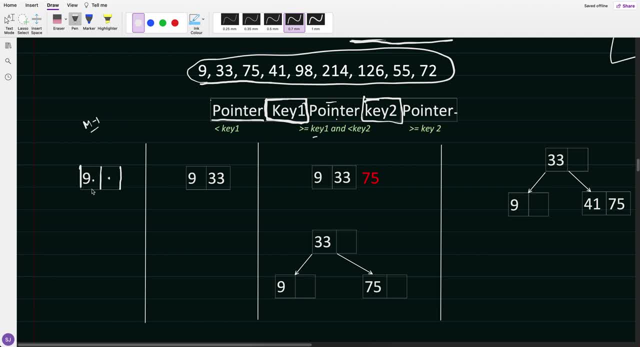 So this is the nodes slots I have. So first I want to store nine. So I have a key, So this is the key one, So I have an space, So I have stored a nine here. Okay, Now I want to store the data 33.. 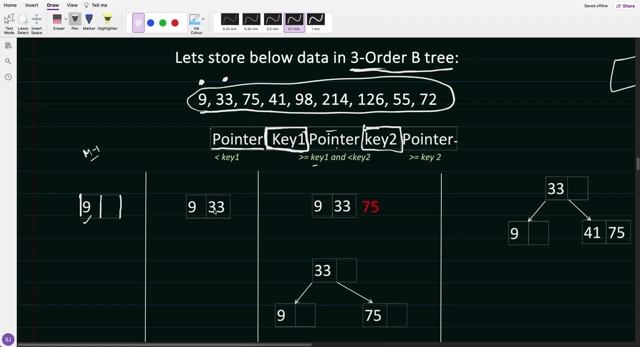 So it always maintain the sorted data. I have a space in this node itself, Right, So I have stored in the sorted order 33.. So both my keys are now full. So it also has the data. This also has the data. 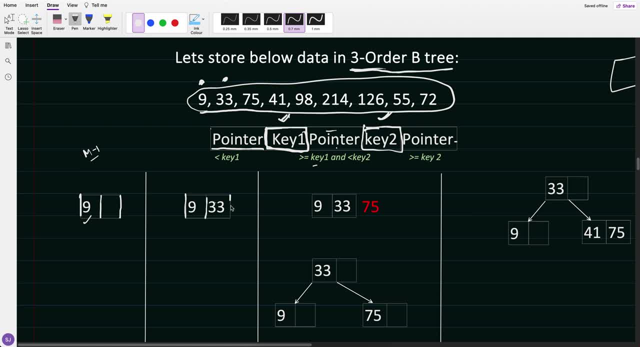 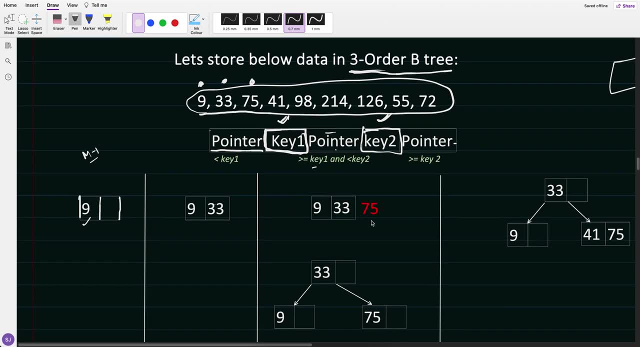 Currently these pointers are pointing to nothing. This is pointing to nothing. Now I want to store 75. So where I would store? now? because in my node, because I am creating a three order tree, So in the three order I can only hold two notes, two keys. 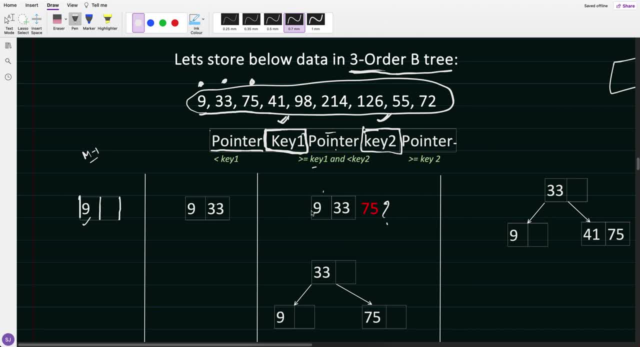 Now where I would store 75.. So now, what it will do is that in the sequencing order it is like 93375.. So what it will do is. so what it will do is it take the middle one and take it to the parent. 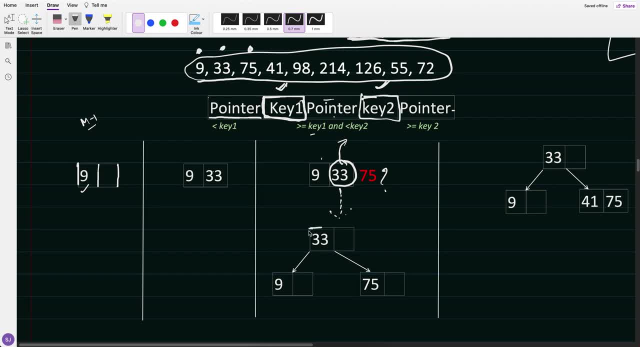 Right. So now what I have done is I have created a new node from the middle, one from the middle one of this three and make it to the parent of this. So now 33.. Now, 33 left pointer Points to this. 33 right pointer will point to this. 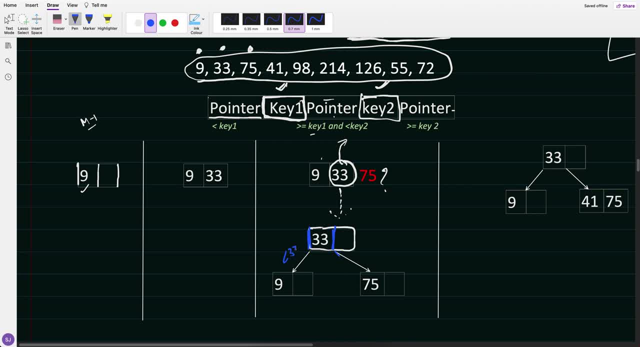 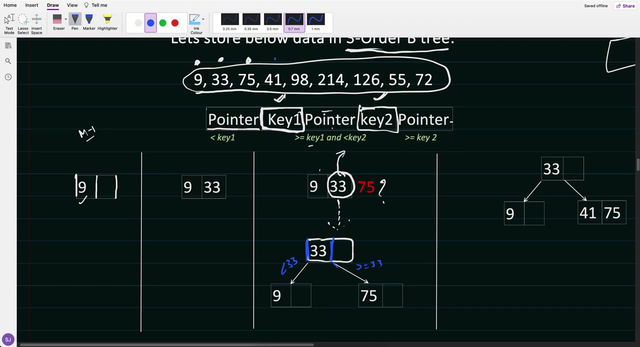 So left pointer means less than 33.. Right pointer could have, like greater than equals to 33 data It will hold. Okay, So till now it's all clear, and this is how the data will look now. Now We want to store. 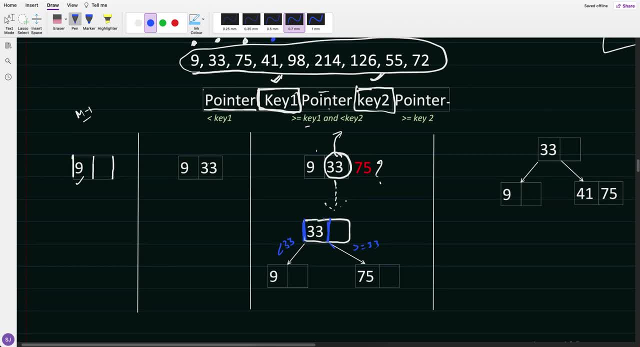 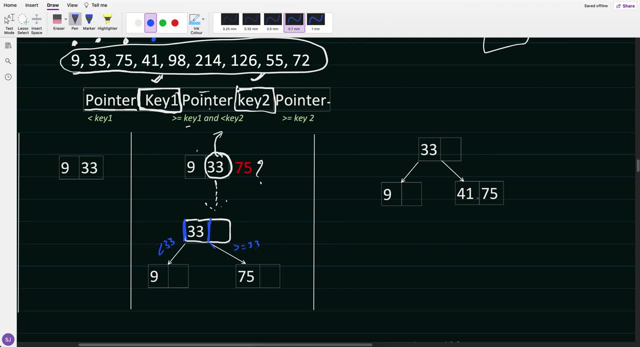 41.. So 41 where we will restore. So it will first check at the 33, 41 is greater than 33.. Yes, it goes to the right side. Now here, if you'll see that, a 75 so 41. so it will sort this, so it will do 41, 75 and it will see that, yes, there is a sufficient space. 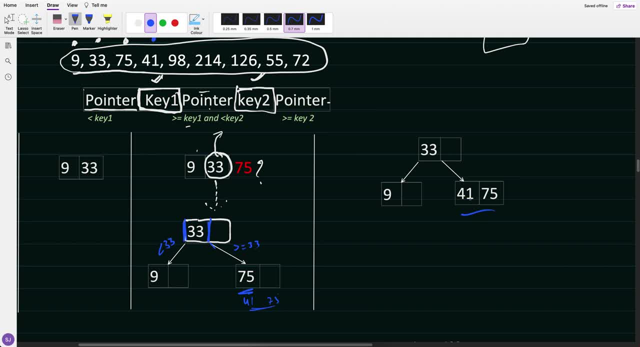 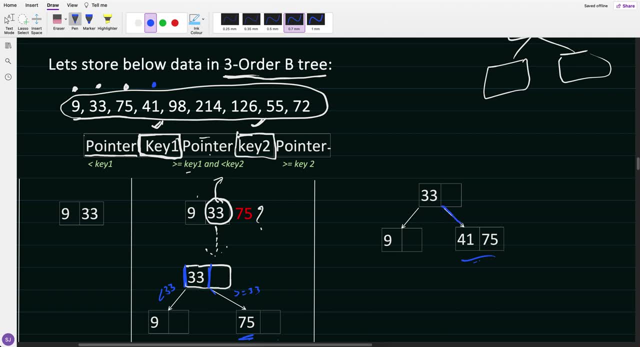 Right, So it will restore it. So this is how it will get restored after 41. Right, Because 41 is greater than 33.. It goes to a right side from the pointer and then it is stored in a sorted manner and it has two notes. 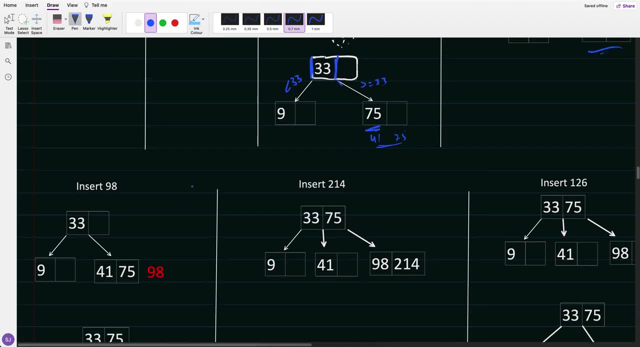 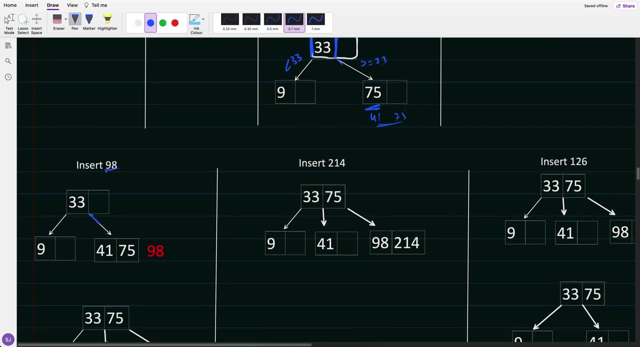 We can keep. so it's okay. Now we want to insert 98.. So 98 is greater than 33.. It goes to the right hand side. Now it want to store over here. So now again 41, 75, 98 in a sorted form. 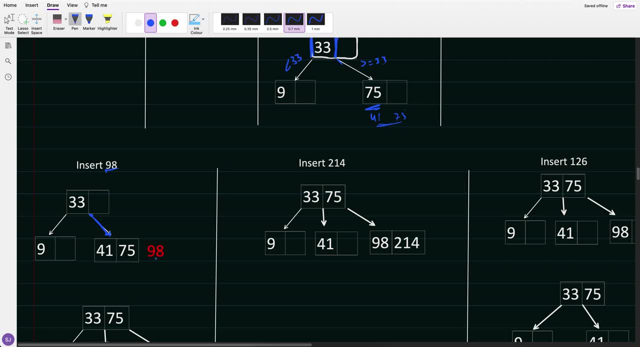 But again, we can't. They store three keys because it's a three level, three order be tree. We can only store two. So what it will do is we will take the mid one and take it to the parent. So it's parent is 33.. 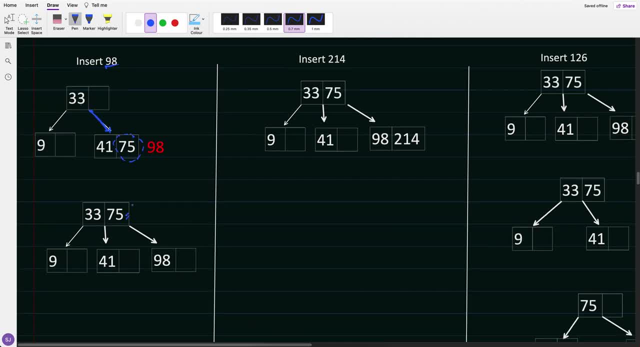 There is an space So it will store there, and 75 left Will point to 41 and it's right will point to 98. So this one is like less than data 75.. This one is greater than equals to 75.. 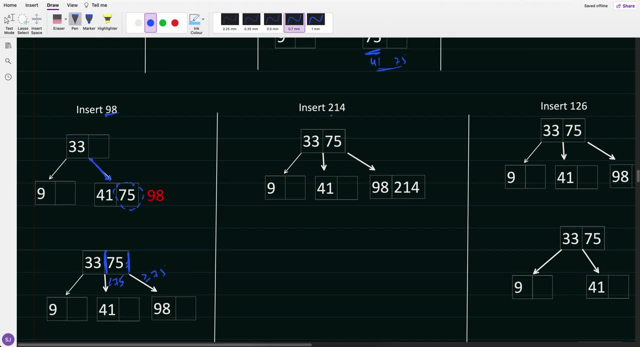 It will point to: Now we want to insert 214.. Now I think you got the point right, what we are doing. So 214, it will check where it will go. It will say that, okay, It is greater than 75.. 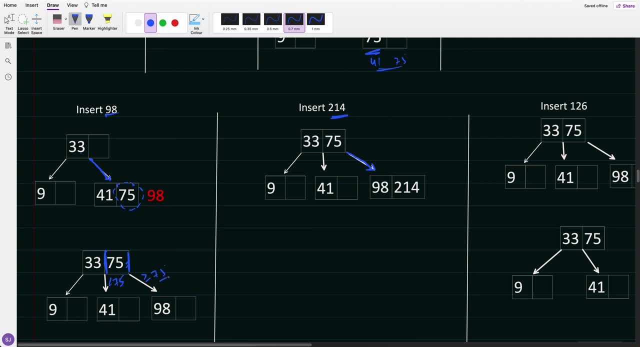 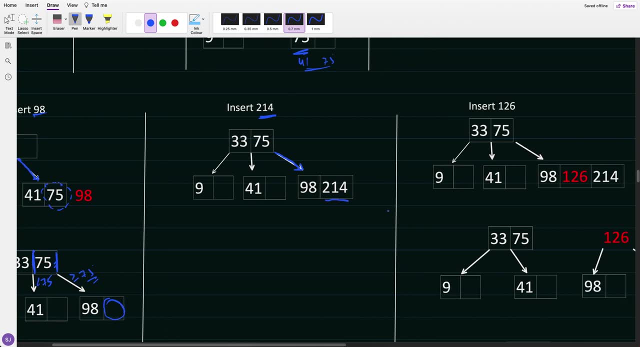 So it will goes here. greater than equals to 75.. It will go here. There is already a slot empty, So it will put it here in the sorted manner: 214.. Now let's say we want to insert 126. 126 is greater than 75.. 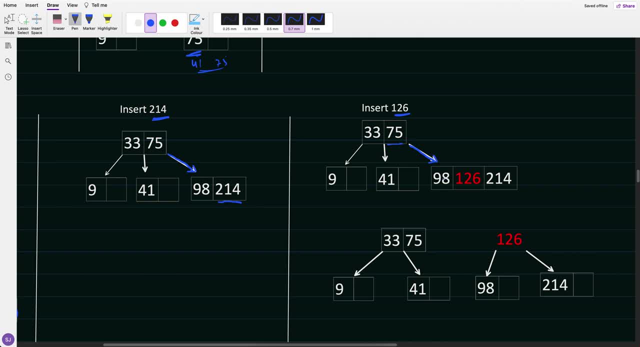 It goes to its right, Right and 98: 217.. So this is the sorted how it would look like, but it breaks the be tree because we can't store three notes only to know two keys we can store. So this has to be mid one. after sorting it has to take out. 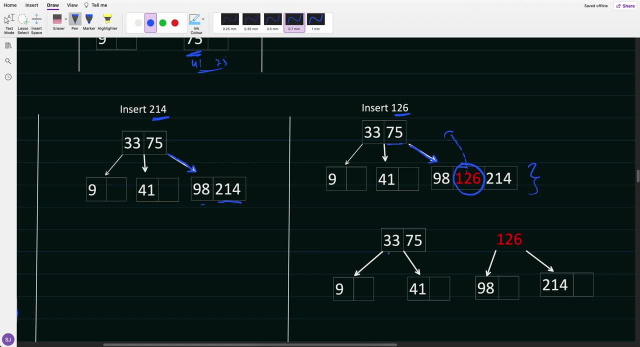 So now it has to take to the parent, So 33.. 75, 126, 126 left will point to this 98.. It's right will point to 214.. But here if you see that this parent itself will get break now because we can't restore. 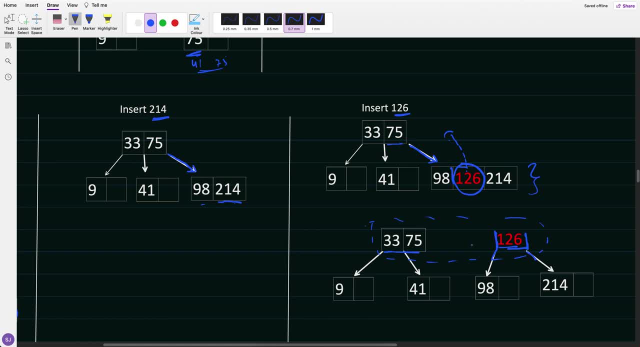 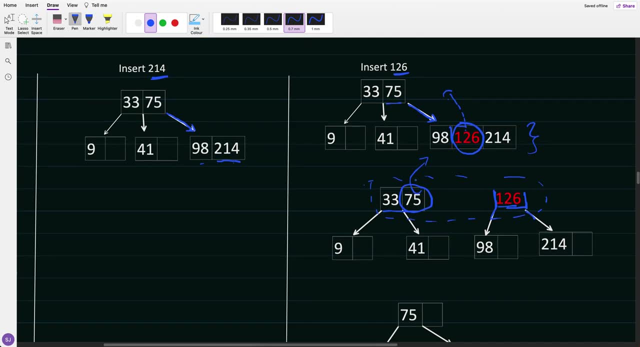 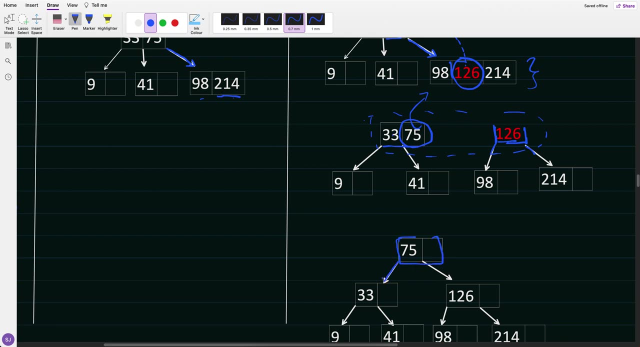 three: 33, 75, 126.. We can't hold it, So this further has to be taken out a mid one: 75. Now it should have. goes to its parent. So there is no parent. We created a new note: 75, 75 left will point to 33, 75 right pointer will point to 126, 33. 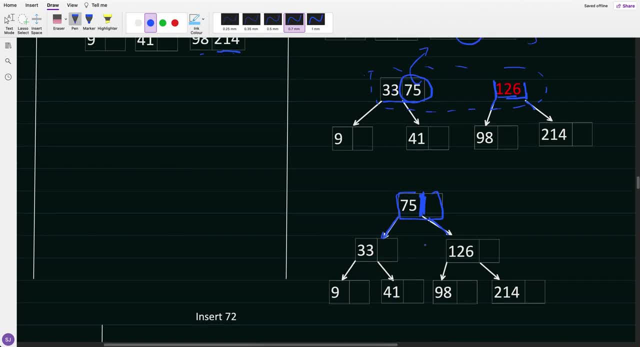 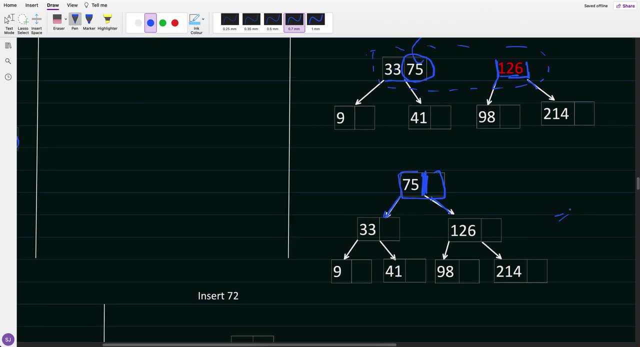 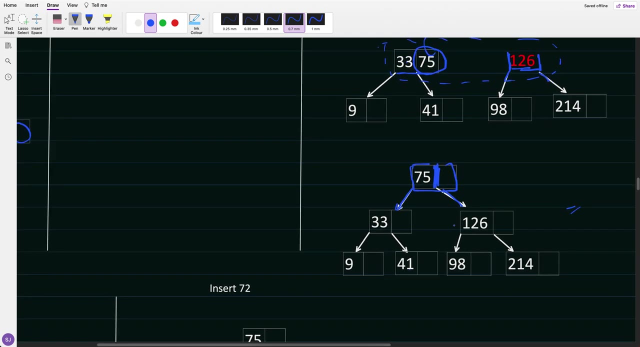 left is already pointing to nine. It's 33 right already pointing to 41. So it is like this. So you got it right. how be tree is towards the data in a sorted manner and plus it can. we can construct M array or M order of B trees. 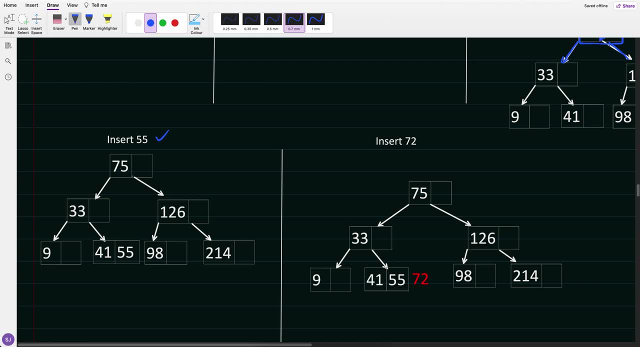 Right. So let's say now I'm storing 55. 55 is 55 is less than here. It is greater than this. It will go here. There is a free slot. 41 free slot was there, So it will restore the 55 here. 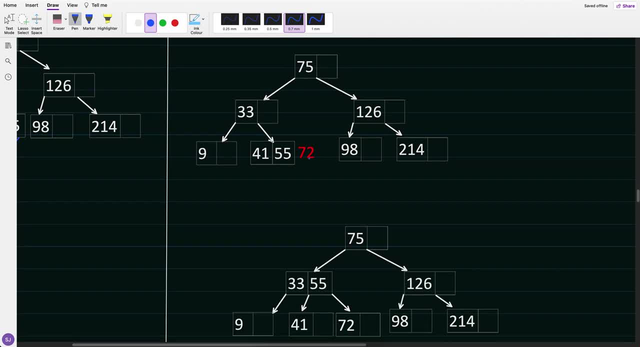 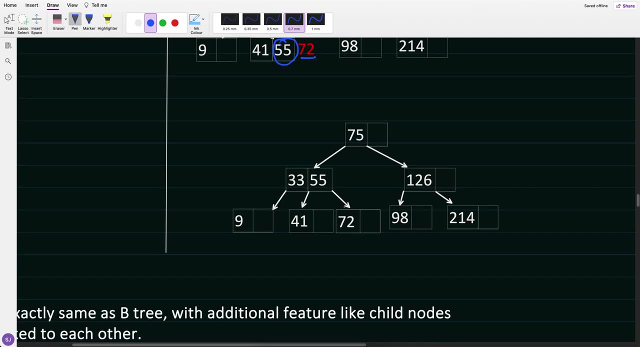 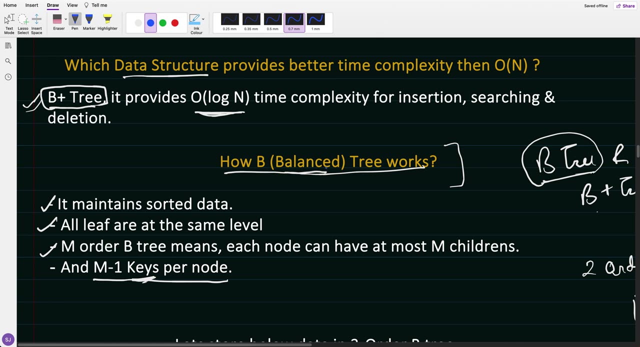 Similarly for 72.. I think you can do now yourself that it will come here but it will break, it will divide 55, it will take it to the parent and how it will look like. So this is how be tree works, Right. So now you know that balance tree, this works. 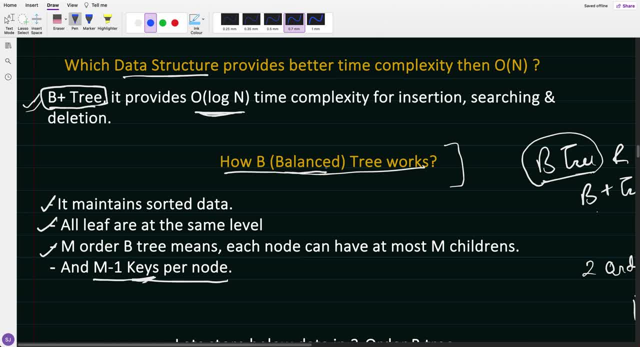 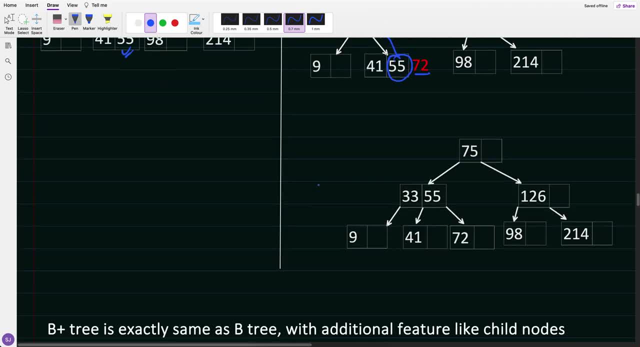 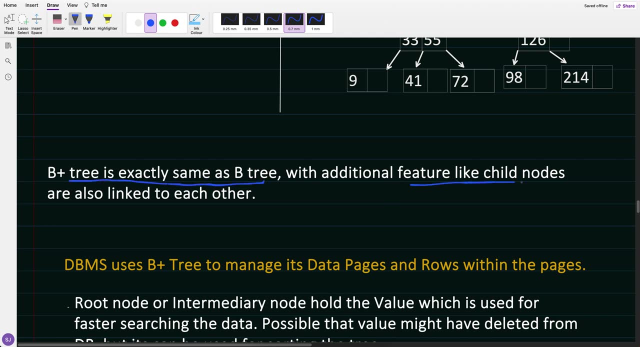 I might have explained faster, because you can learn this data structures more in depth or you can implement it, but without understanding this indexing, understanding the indexing would be incomplete. So beat B plus 3 is exactly the same as B tree, with additional feature that child notes are. 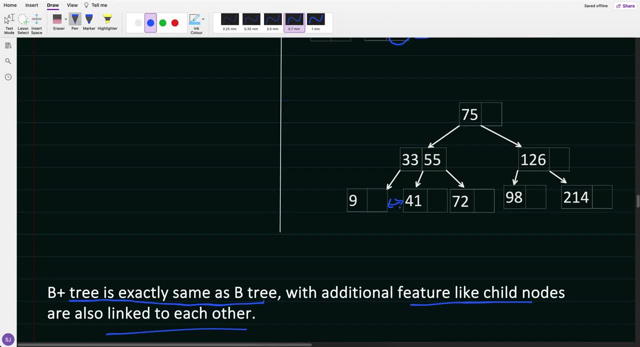 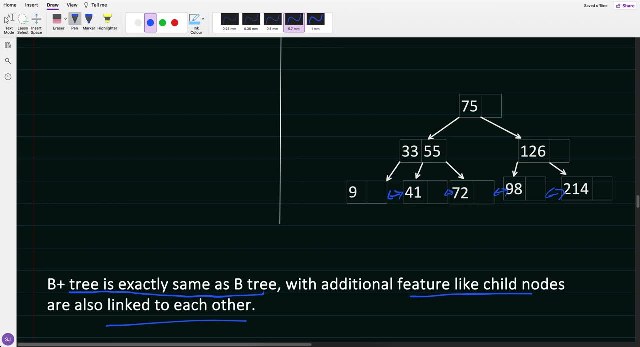 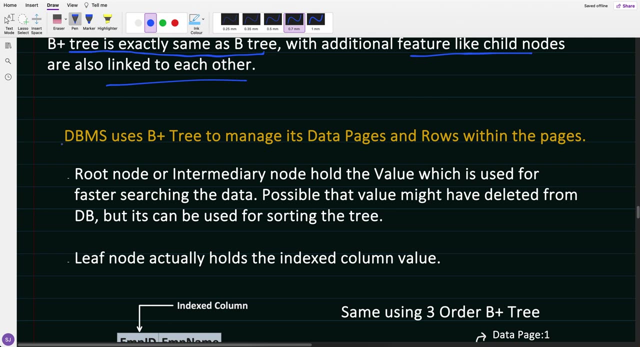 also linked to each other. So in the B plus 3 it has additional feature that this All child notes are linked to each other. So that's okay. If you understand the B tree, B plus 3 is also exactly the same. So now let's come back again to our DBMS. DBMS is using the B plus 3 to manage its data page. 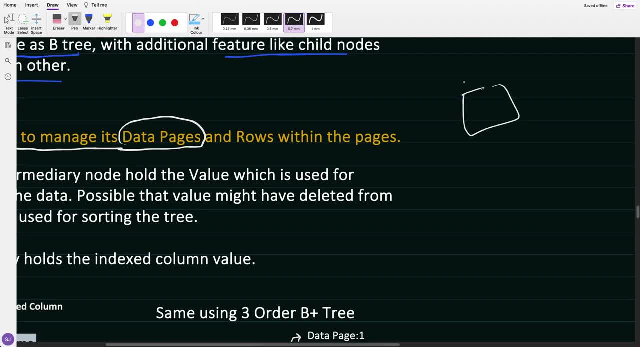 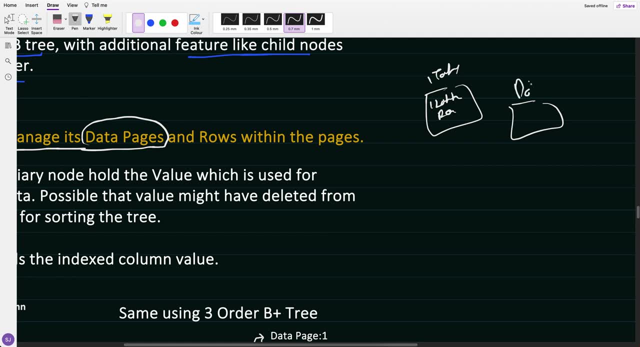 Because I told you that for one table, if it is a, let's say, 1 lakh rows, It can have so many data page: data page 1, data page 2, data page 100.. Let's say, and inside each data page There will be hundreds of rows. 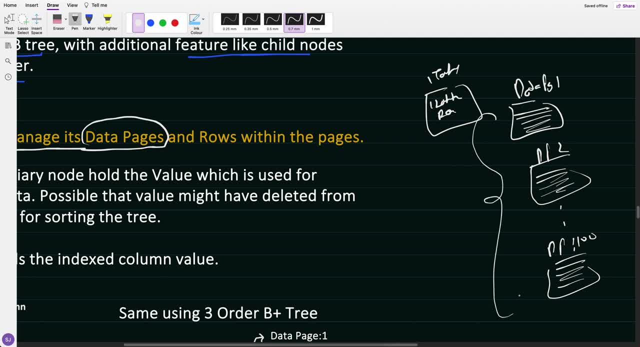 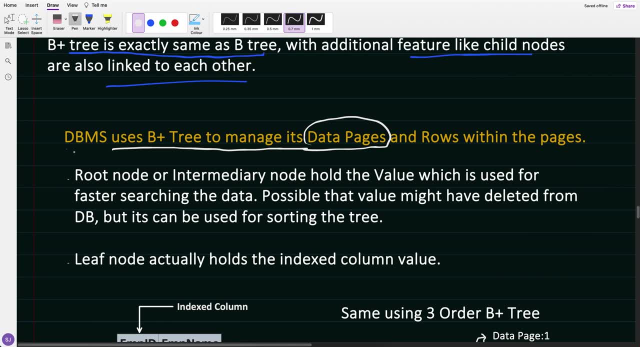 So there might be some kind of ordering right, how to order those right. So that's where we. that's where B plus 3 comes into the picture. DBMS uses B plus 3 to manage its data page and rows within that pages. How? 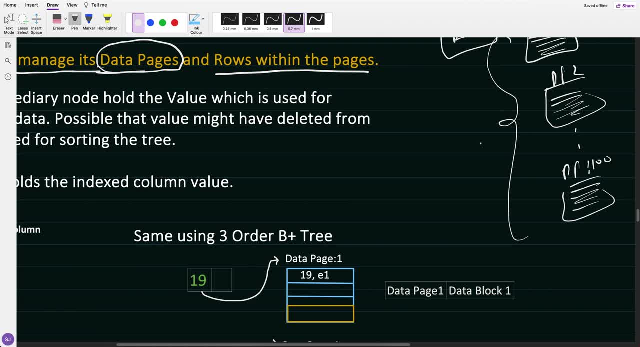 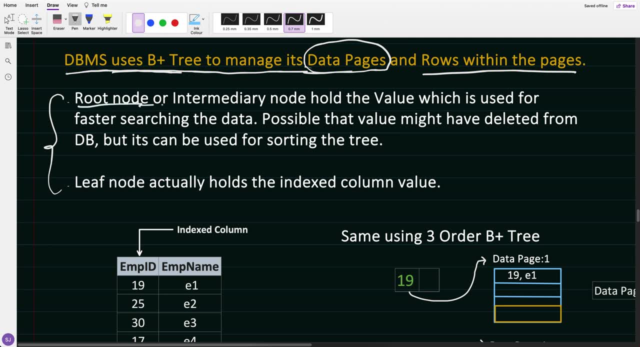 Okay, so just have this. like it is using the B tree, exactly the same, only with slight differences. The root node, or intermediate in node, holds the value, which is used for faster searching the data Possible. that value might be deleted from the DB, but it can be used for sorting the tree. 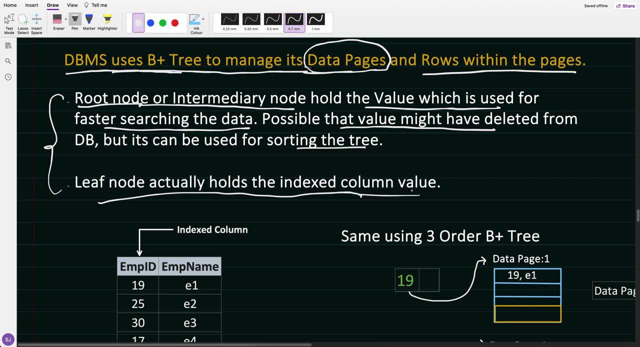 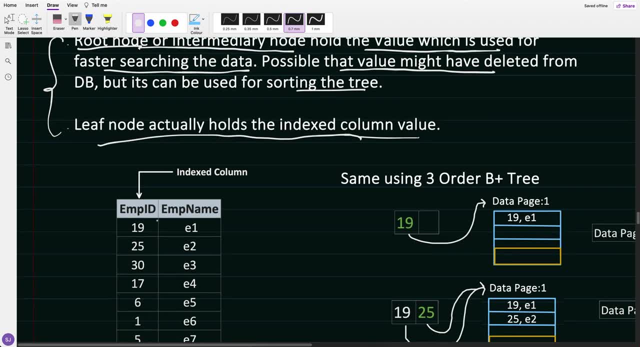 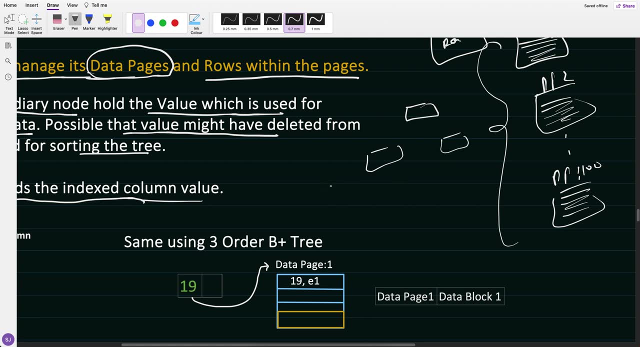 Right leaf node actually holds the index column value. Don't worry, I'll tell you what I mean to say, that how, what DBMS is do we will see that. So what I mean to say is that here is so, here, when we are maintaining the B plus tree. 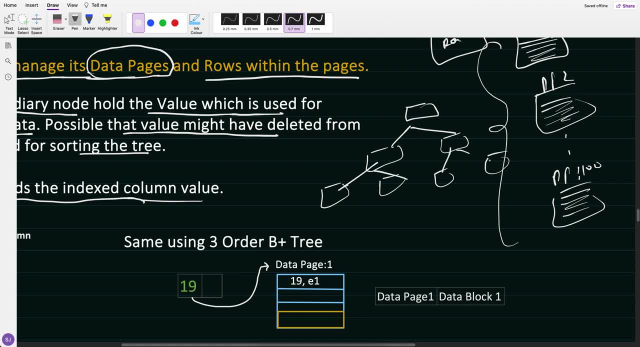 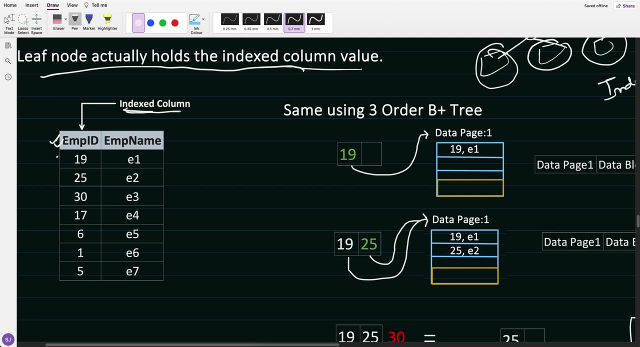 The ultimately the leaf node. This leaf nodes Actually holds the index values. So let's say, this is the column in this column I am, this is, I want to put an index, So this is the index column. So what is the index value? 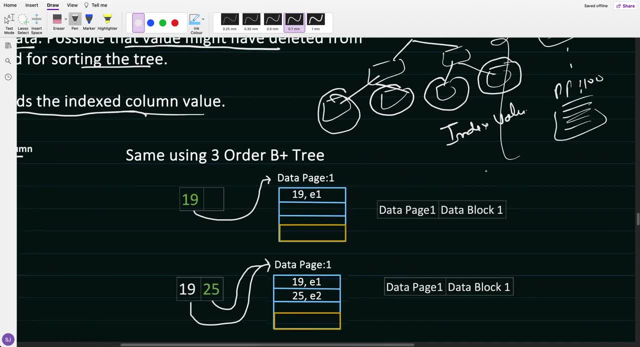 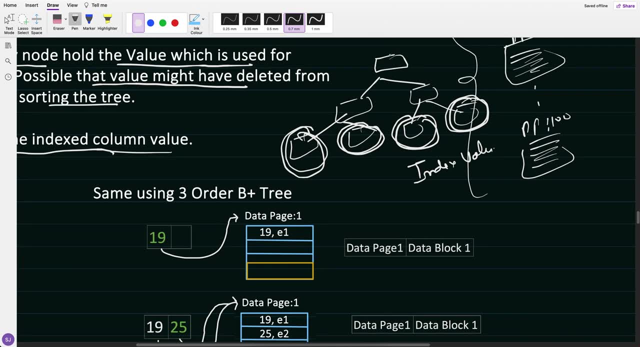 19, 25, 30, 17, 6, 1, 5.. So these leaf node are actually the one Which holds this index values: the root node and the intermediary node. this root node and intermediary node might restore some data. Let's say it. 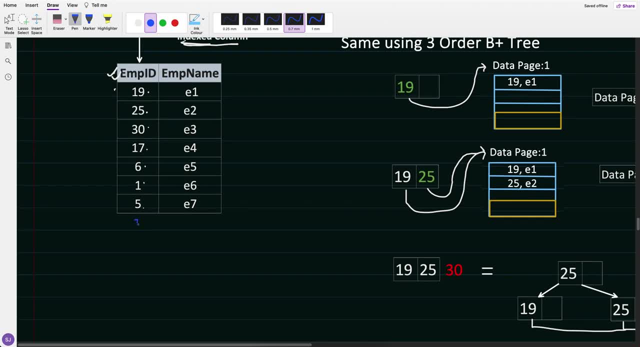 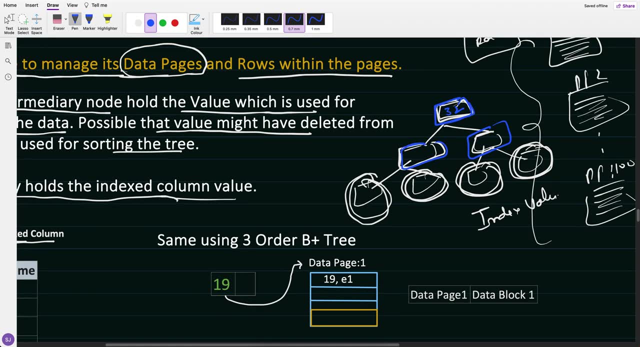 32, which might even not even there earlier. It was there but it might have deleted. It's not even there now. So it is possible that it might be present here into the root node or intermediary node, because they just help us to do a faster searching: go left, go right and all. 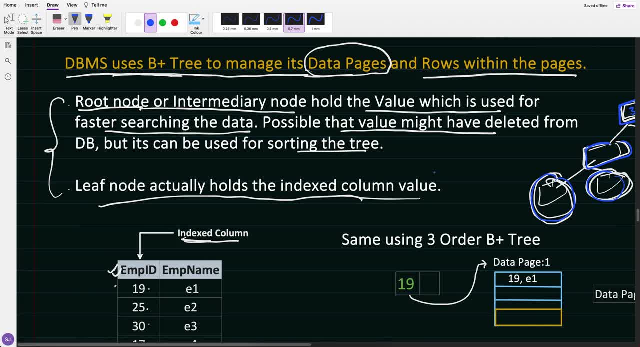 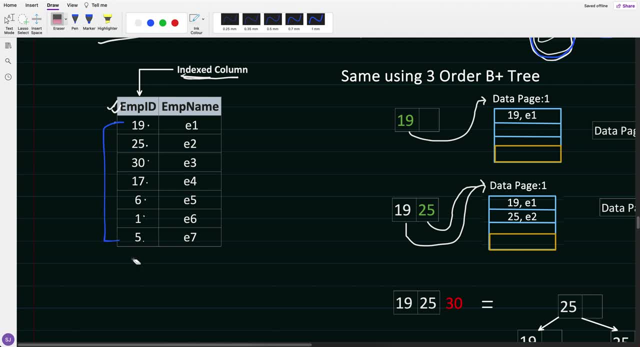 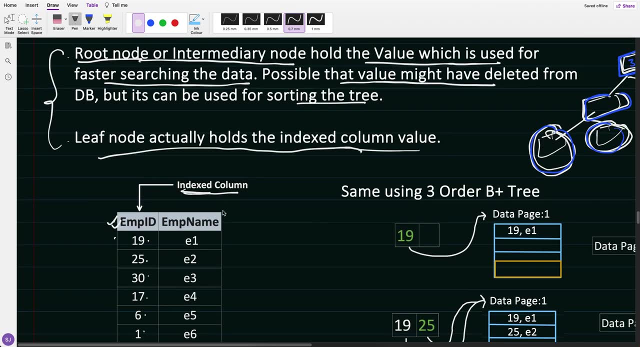 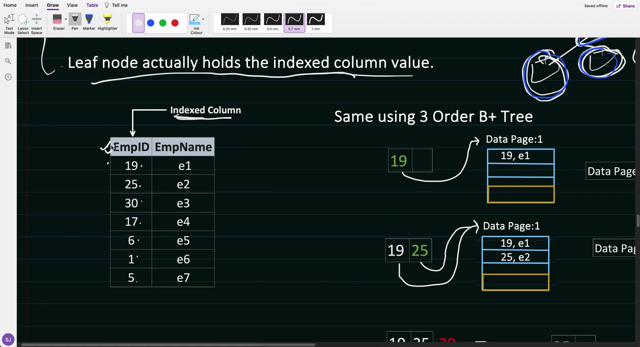 But this leaf node actually holds this current values of the column, which is index, and that's what I meant to say. Okay, So now let's see how DBMS is actually using B plus 3 to maintain the data pages and indexing. Now let's say: this is the table, very basic table, right. 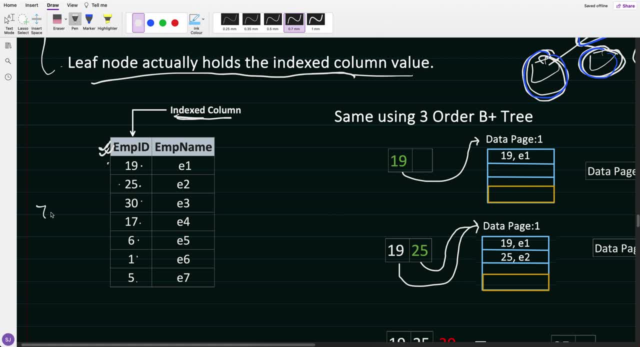 How many rows 1, 2, 3, 4, 5, 6, 7, 7 rows Are. let's say, our row 1, row 2 to row 7, right, and we have two column, column 1, column 2, very basic table. 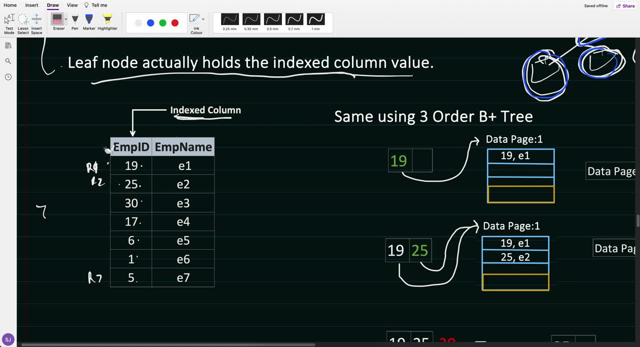 Now I have put an index on Employee ID. I have put an index on this employee ID so we know that whenever we are putting an index now, DBMS will Apply B plus 3 on it. Apply what B plus 3 on it to sort to manage. 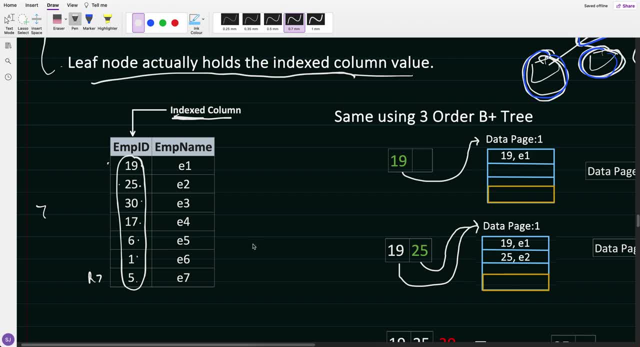 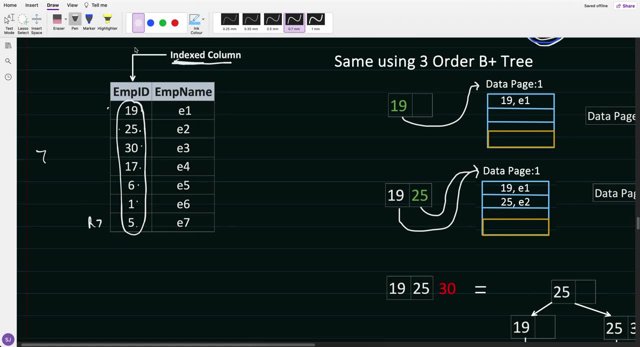 This data. How right. so exactly the same way which we. it has done, exactly the same way It will do this. So now, this is the column where I have put an index. now It will read this: 19, 25, 30.. 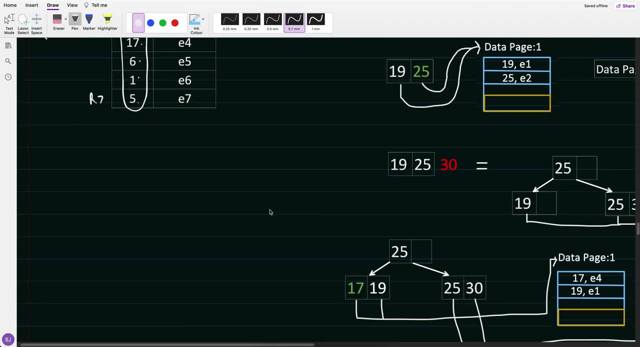 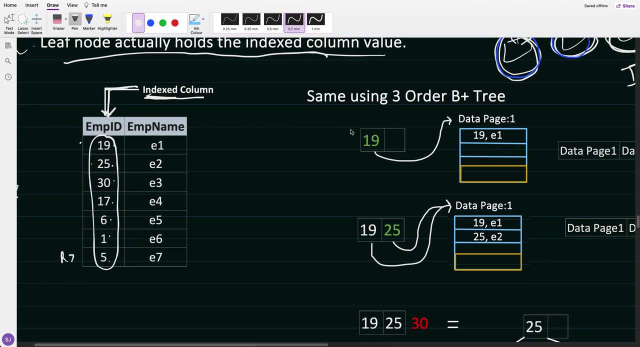 So now it will start creating a B tree out of it, right? So what before? even so, don't look at this pointer now, right, I will explain you, But now see this. first is 19.. So you know that I am still using the three order. 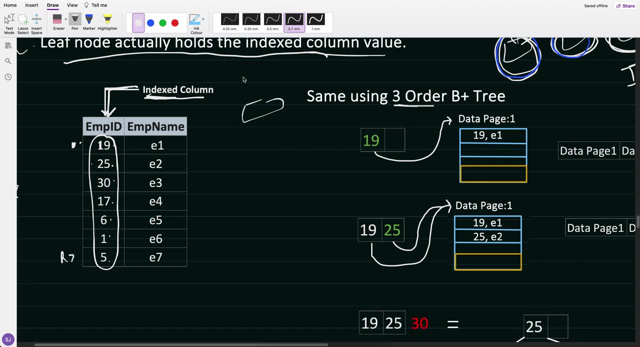 So in three. order means how many one node, how many keys you can store, and minus one, which is two right. So and there, how many pointers would be there? three pointers would be there and two keys I can restore, So 19.. So in the key one I have a store 19.. 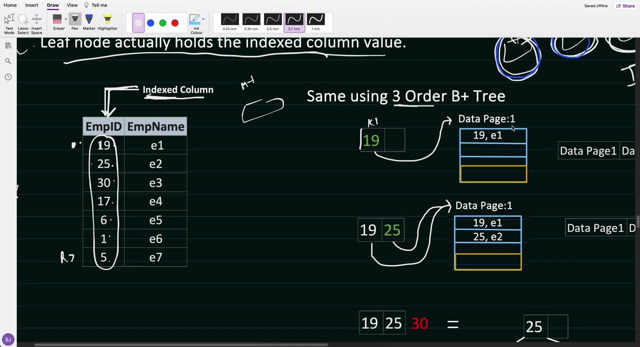 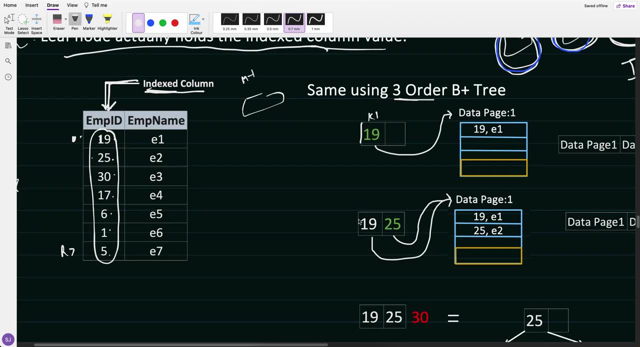 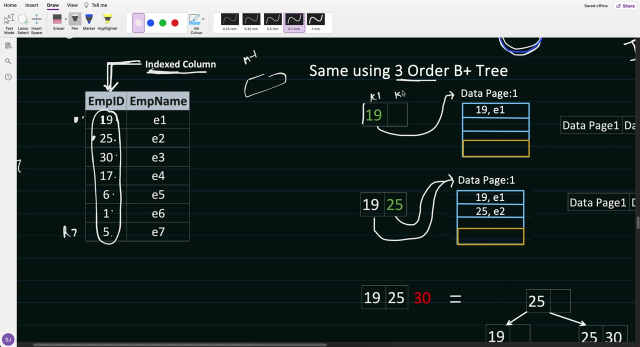 Okay, don't forget about this pointer Now, this pointing to the database, and I'll forget about this. Let's first focus on this: construction of a B tree. The second is 25.. So now the second row is coming, 25.. So the key to was empty. 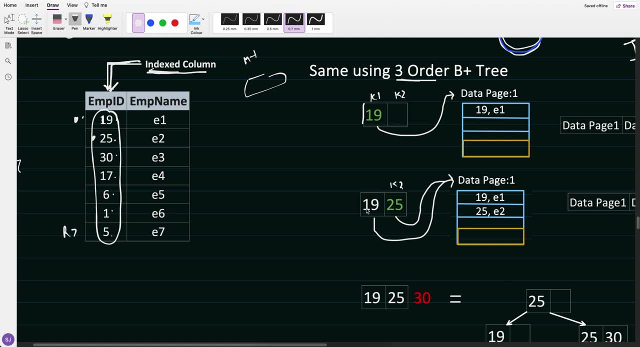 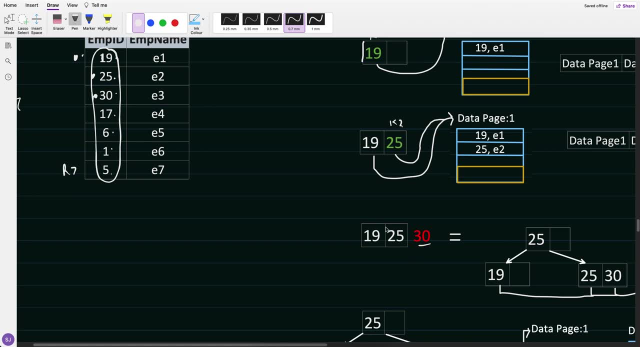 So I have put 25 into this part. Third one is 30. So now if I put 30 here, it will break, because it's a three order tree. in one node You can have only two keys, You can't put 30.. 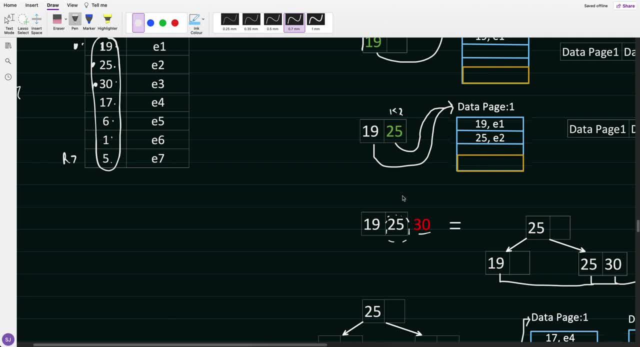 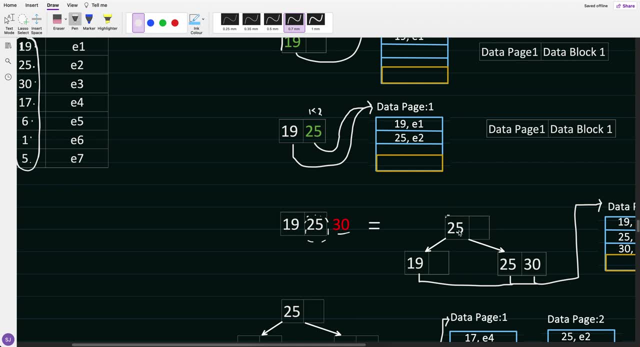 So you have, After sorting whatever the mid one is, you have to take it to it parent. So it would look like this: So there were no parents. So I created a new note. I put 25 there, 25. Now, left pointer will point to 19 and it's right pointer will point to this node, which holds: 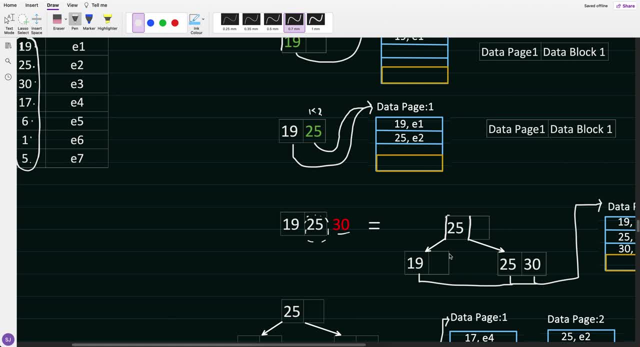 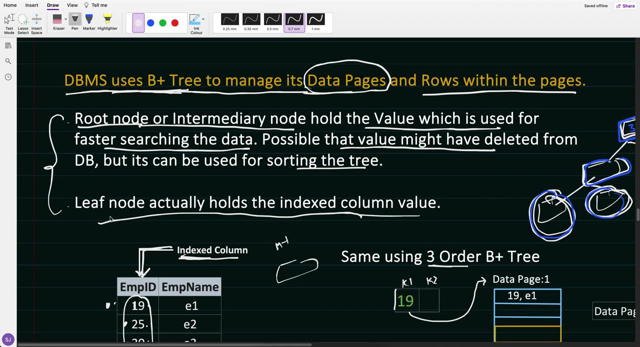 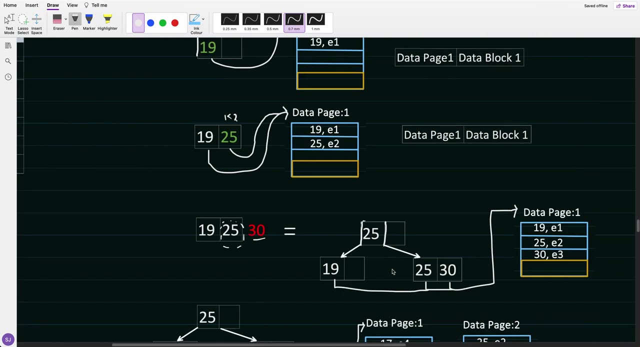 25, 30. So now this is the first different. you should notice I told you right in the DBMS, when it use B plus tree, Leaf node actually holds the index column value. These are the index column values, right? So leaf node is towards it. 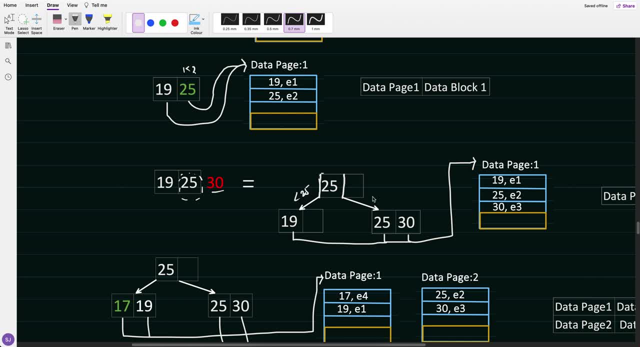 The left pointer hold less than 25. right pointer is told greater than equals to 25.. So here, if you see, I have put the 25 here also. I have put the 25 here also because in the leaf node itself we hold this value. 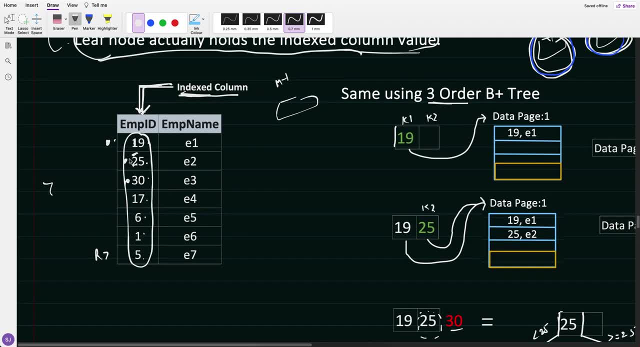 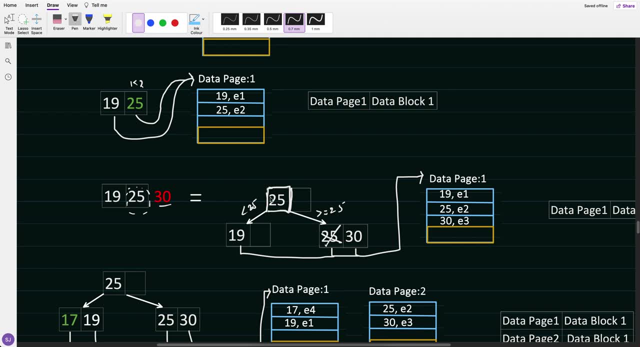 In future it is possible that 25 rows deleted, So I might delete this, but this could still be there. This is an intermediate, a node, This is just for faster searching. anything comes, He goes to write this right, You will find values greater than equals to 25.. 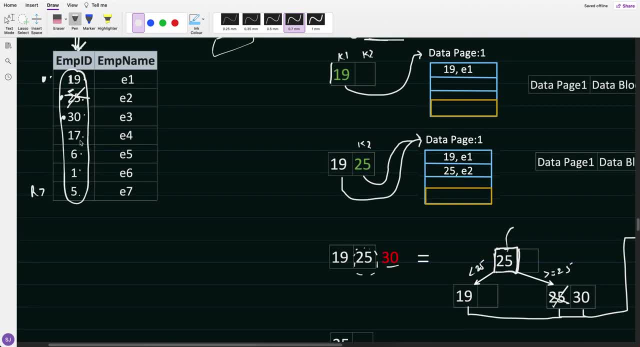 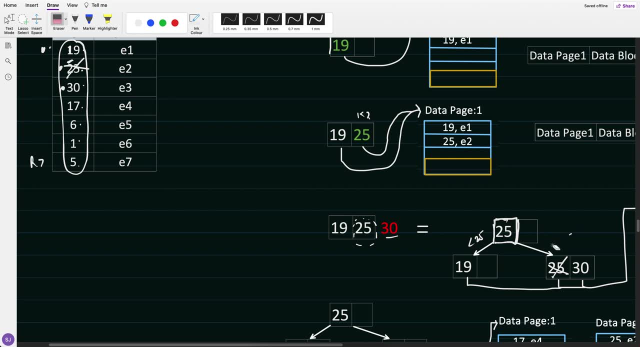 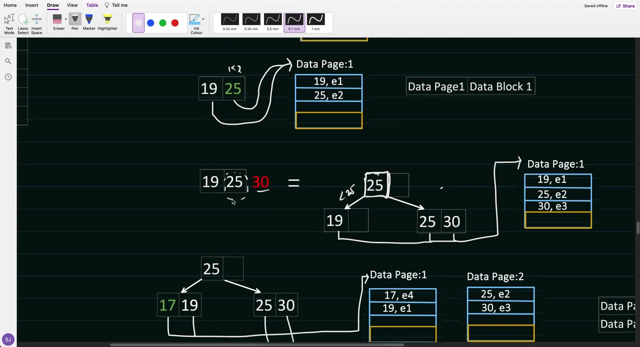 But this doesn't signify that this is the index column value in the DB which is stored. No, Okay, got it So. So this 25 right, we have to put greater than equals to 25.. So we are restoring the 25, right. 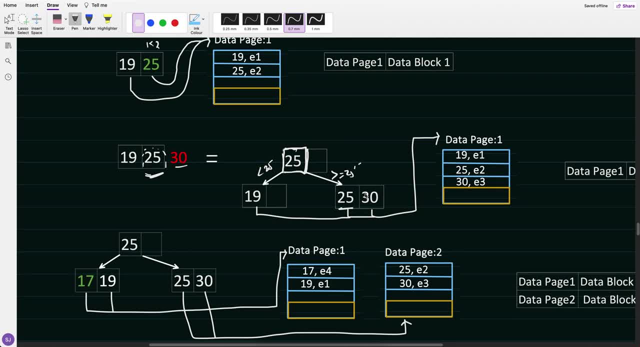 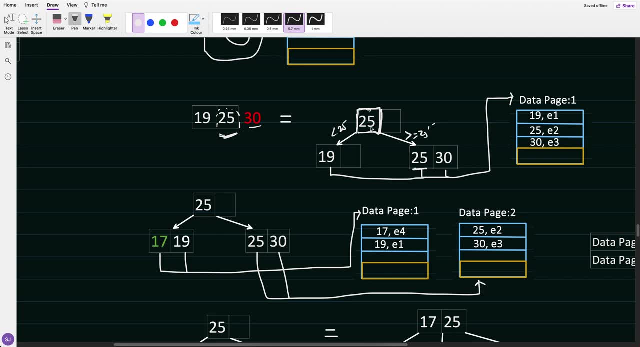 So 25 would be stored here and 30. So, in a sorted manner, Then, what we have to store, 17.. So in this 17, where it will go, it is lesser than 25.. It goes to the left side of it. 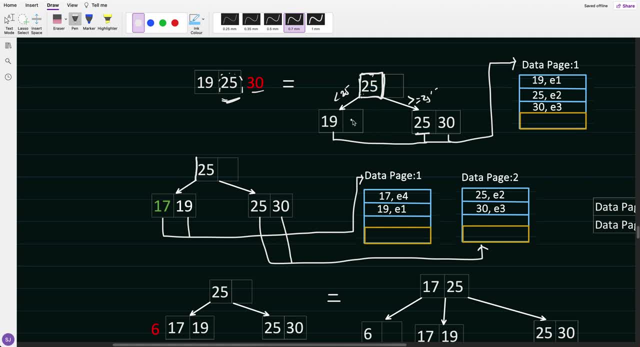 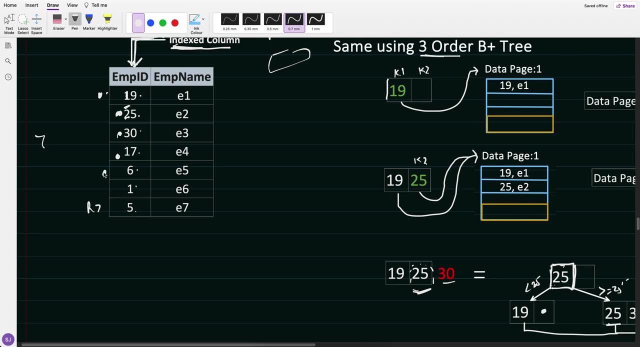 17 is lesser, So it will go to this. There is already one space present, So it will store in a sorted manner. So 17 first, 19, later, After that 6, where the 6 will go. So 6 is lesser than 25.. 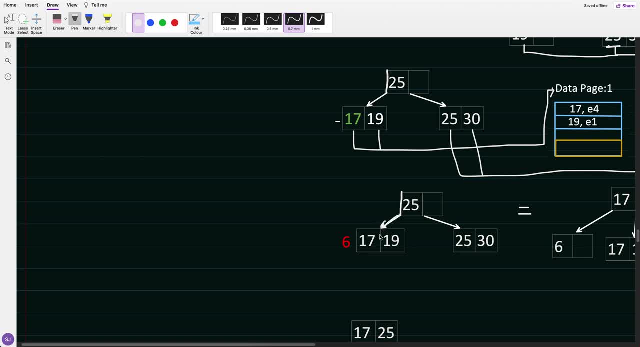 It will goes there. Now there is no child. So generally 6 would be in the first of 6, 17, 19 sorted manner. But again, three keys We can't stored over here. We have to now divide. Take a mid one. 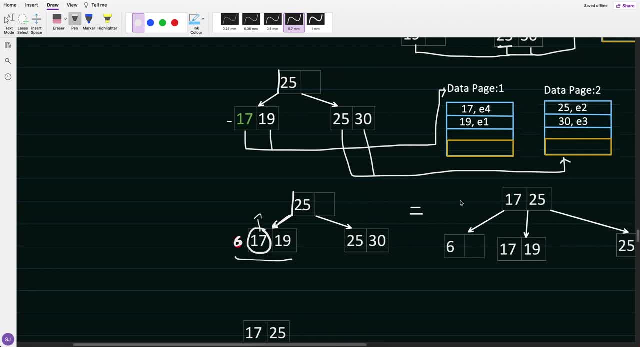 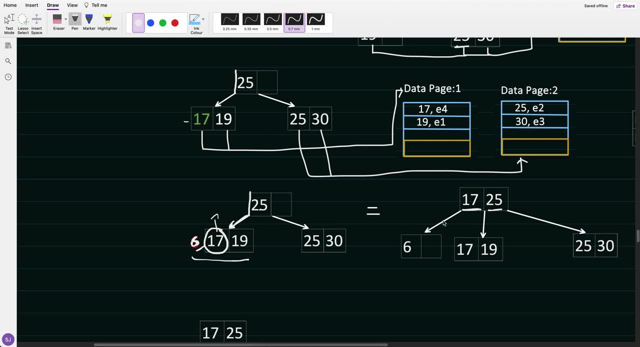 Take it to the parent who is the parent: 25.. So it will, in a sorted manner, 17, 25.. 17, left will point to 16.. 17, right, because this is a, still have the index value, right. So it will point to 17 and 19 greater than equals to 17, 17 and. 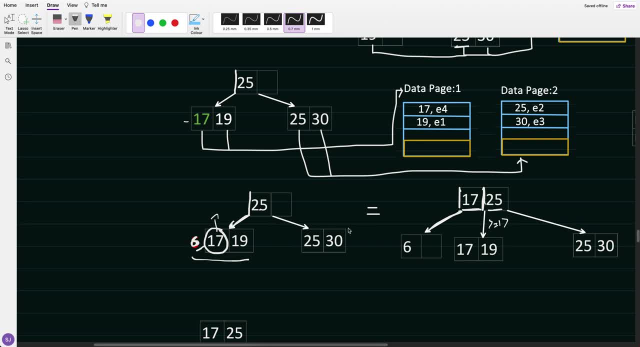 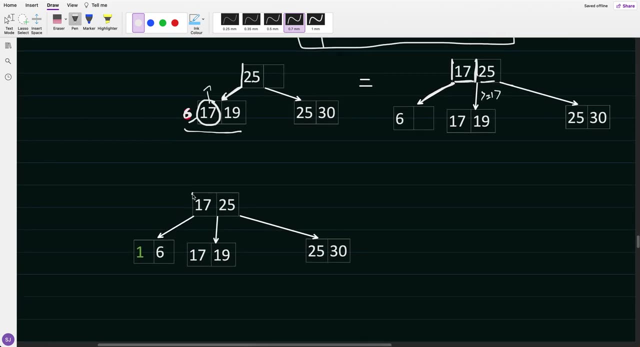 19. And 25 right will point to its 25- 30. So you see that three child It has currently each note. Then we want to store one, So one is less than 17.. It goes to the left, So there is one space. 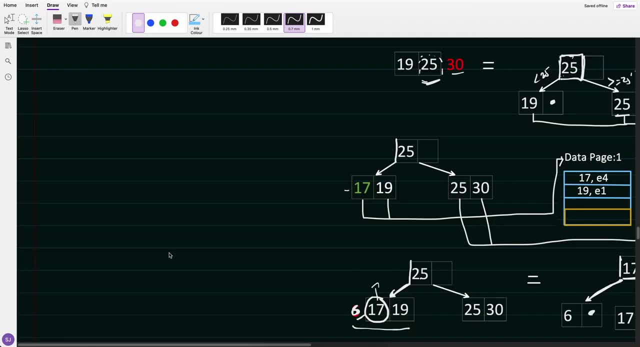 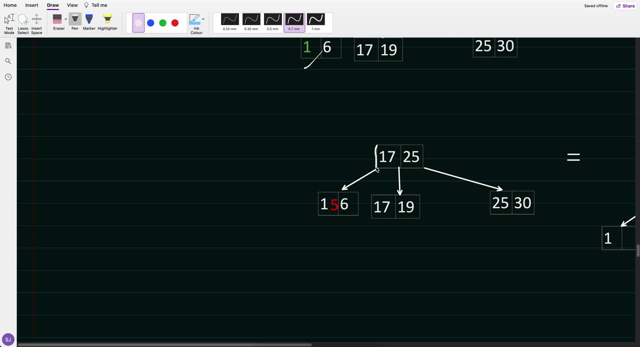 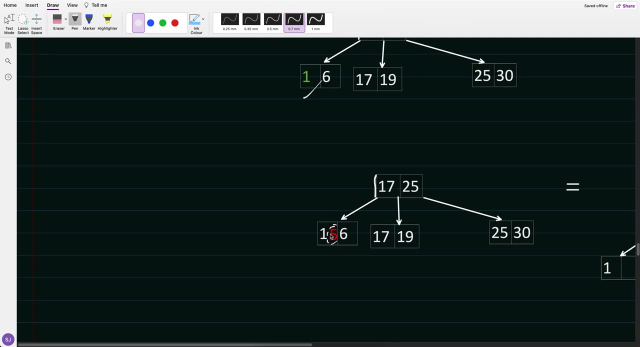 So it is stored in a sorted manner: 16. Similarly the five. so the five lesser than this it goes here. So generally the five should be here in between of one and six, But it will break. So three keys We can't have it. 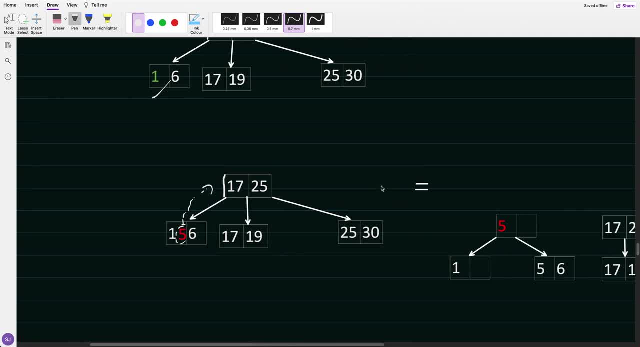 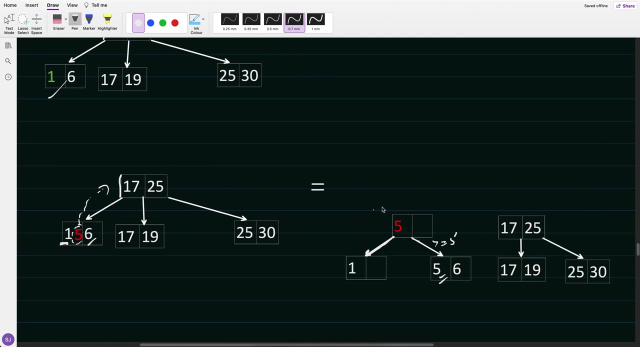 So it should goes to the parent right. If five goes to the parent, the five left would become one. Five right greater than equals to five when it's a key also. So five should also be there. five and six, But at the parent level you can't have three notes right. 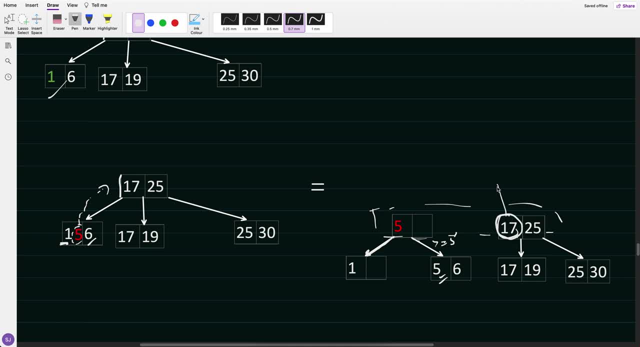 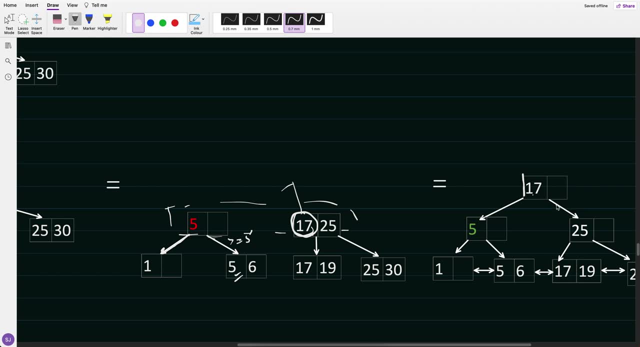 So again the mid one: 517, 25. again It has to go to the top. So it's: hold this five, It's right, hold 25.. Now here, if you see that I am not putting 1725 right, because this is just an intermediary node, intermediary node. 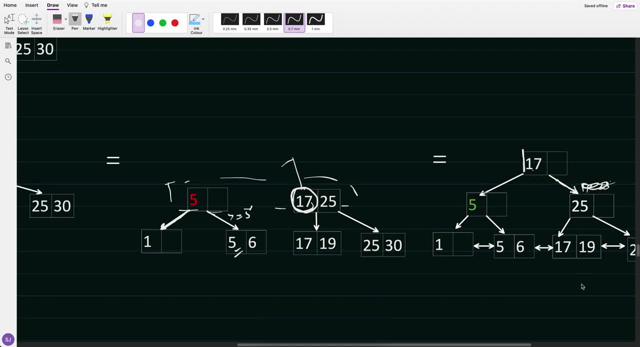 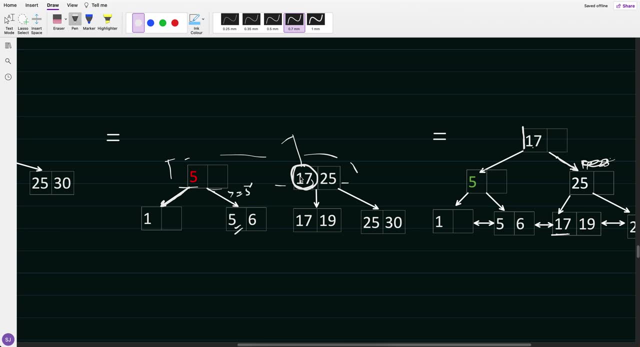 I told you that it is not index column index values. column index values are only the leaf Right, So I am only changing the intermediary node. It's going top. So that's why I don't have to put 17 here, because it's not index. 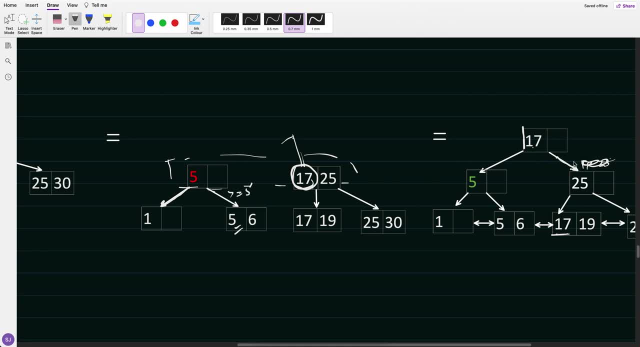 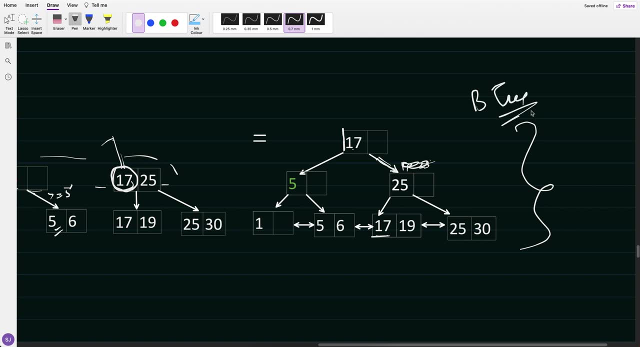 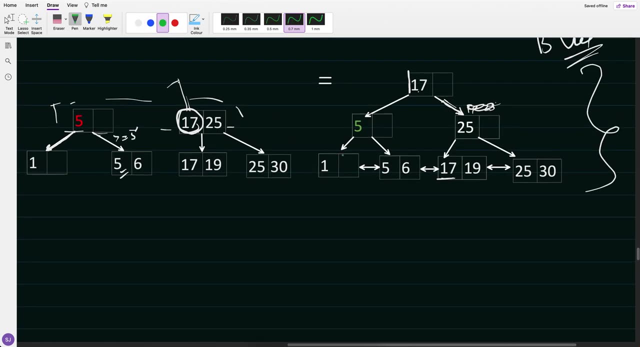 column index value, So 17 right, will point to 25 and this thing, so it's graph, will be: so this B tree is constructed. So now here, if you see that at the bottom, this bottom part, This bottom part, This is now sorted. 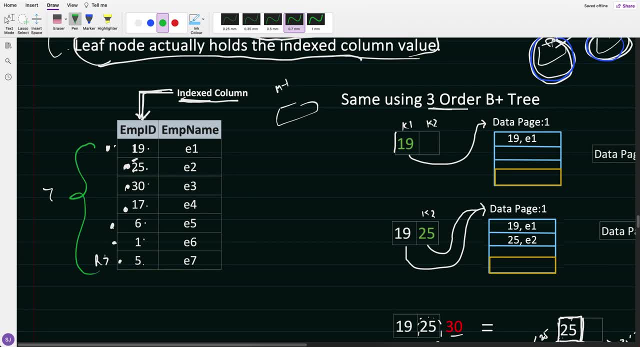 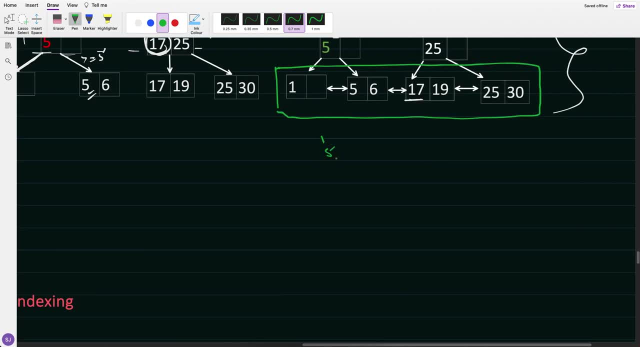 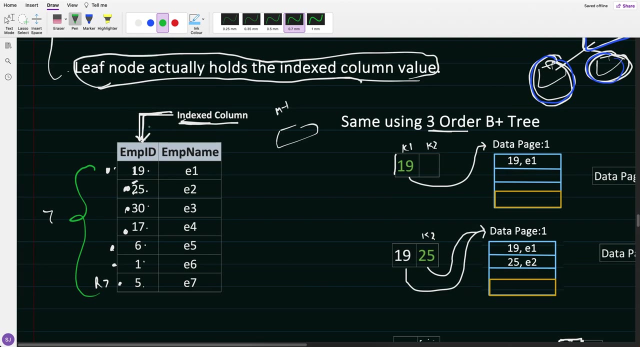 So here we have a mixed data but bottom what we have now of this B tree, This one, five, six, 17, 19, 25, 30, see sorted Right now. we understand that okay, how, whenever we make any column index, whenever we make any column index, DBMS do B plus 3 on it. 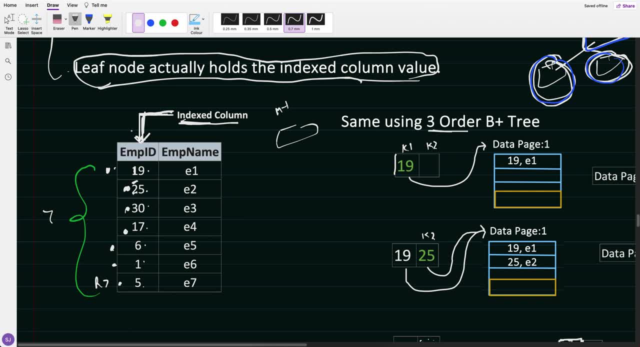 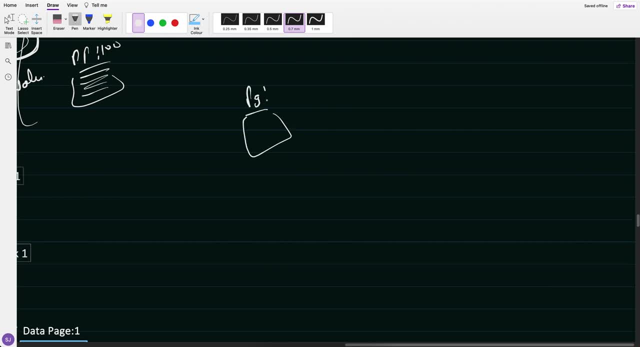 But strange How the data page Are created now, how it gonna link, because you told that one table can have hundred of data page. data page one data page 100.. How those gonna manage, Right? So, because these are actually has the row. 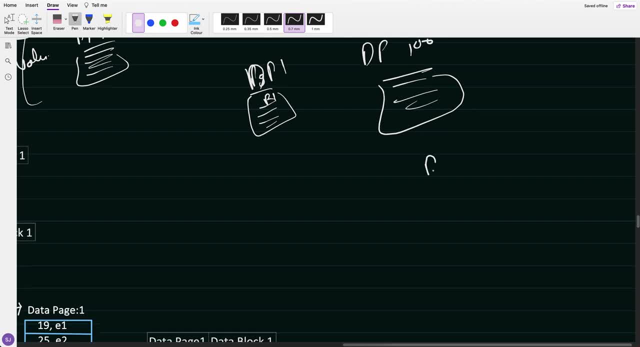 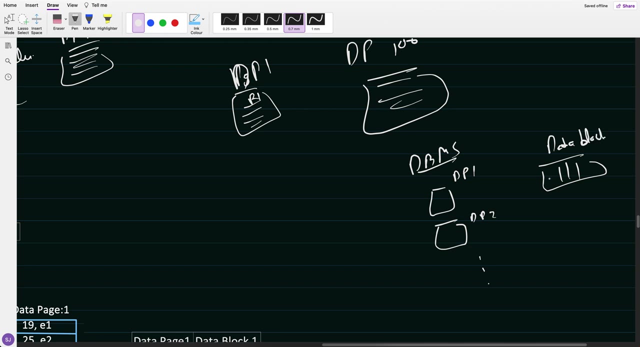 So what till now I have understood is okay. DBMS has so many data pages- Data page one, data page two, like this: Each data page is stored in a data block And one data block can have many pages, like page one, page two. data block can have certain. 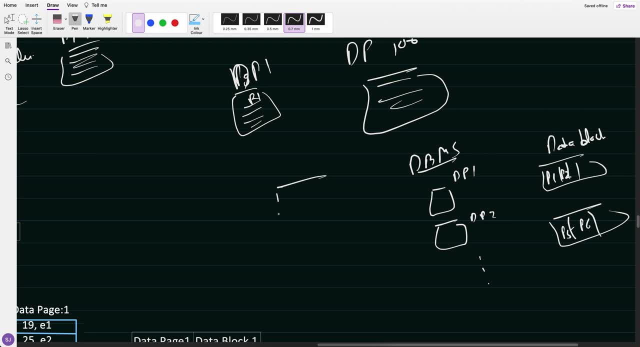 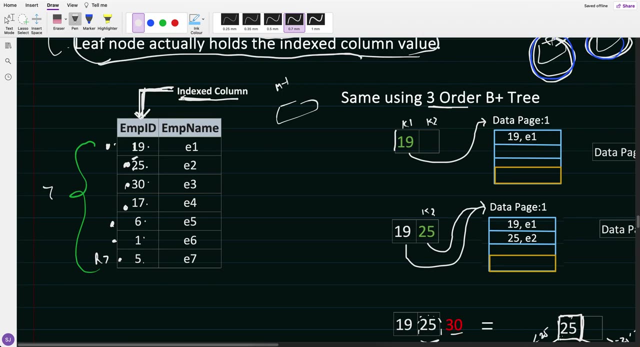 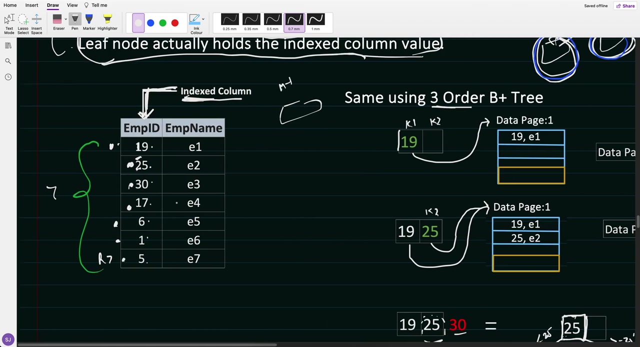 Let's say page five, page six, something. DBMS maintains the mapping of page page one, block one, page two, Let's say again, block one. like this: it mapping it does. I know that whenever any column Is indexed right, it maintains a B3. you will now understand how B3 is constructed so that the data of this column is now in the sorted manner. 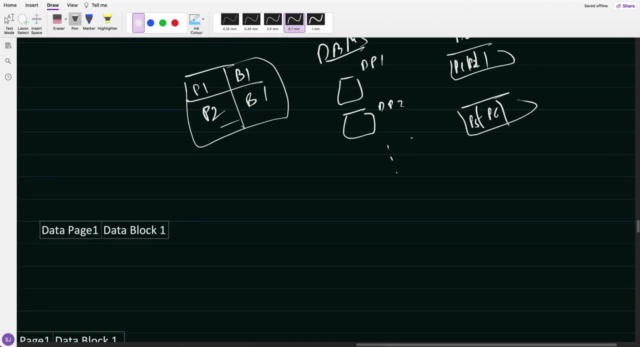 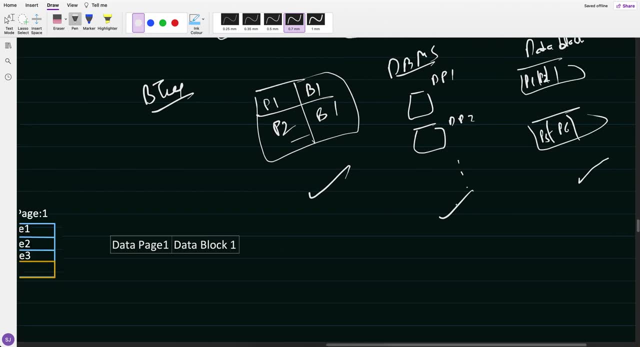 In a sorted manner, But now we need to connect the dots. So now, B3 exist, I understand this, I know data pages, I know data block, But what is the dots connecting to all of this? Now, let's understand this. 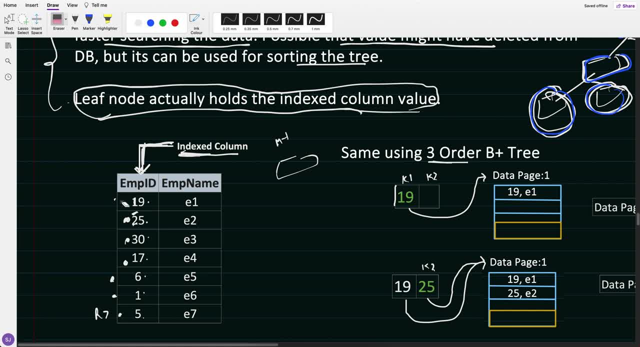 Okay, Now let's understand this: our table Has Empty And we are doing inserting the row from start, Right. So now let's say, we have make this column indexed and now only first row is inserted, 19 even. This is the row. 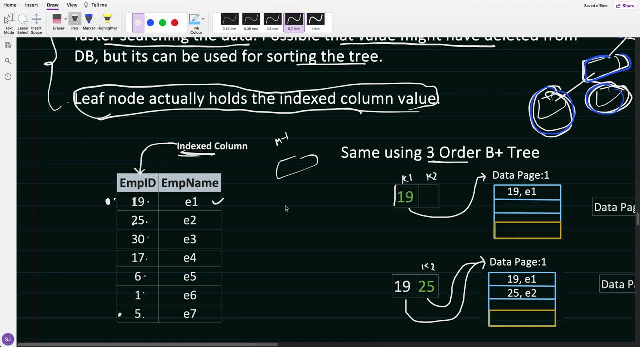 I told you now that first what DBMS is will do, it will create a B plus tree right for this data also, So it will put 19, now remember, in DBMS. with this key It will also hold one more pointer value, or you can say that the pointer with this key is which ultimately points that this belongs to which data page? 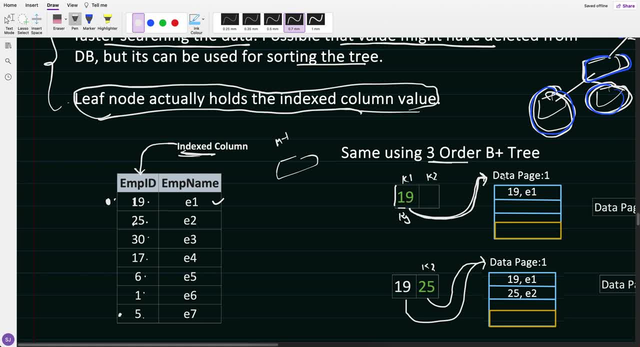 This 19 is stored in which data page? So now, let's say, I told you that this is the first time we are creating a table. This is the first row, So data page is currently empty. So I created a data page one and stored one row, 19 even, and stored, put a pointer here that, okay, this 19 is points to this data page one. 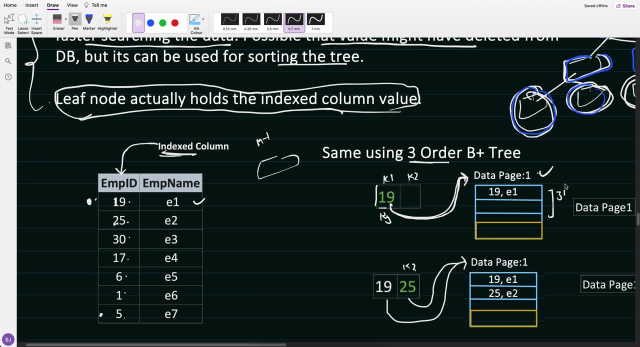 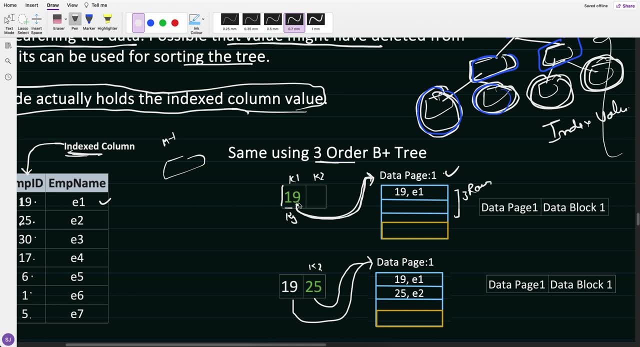 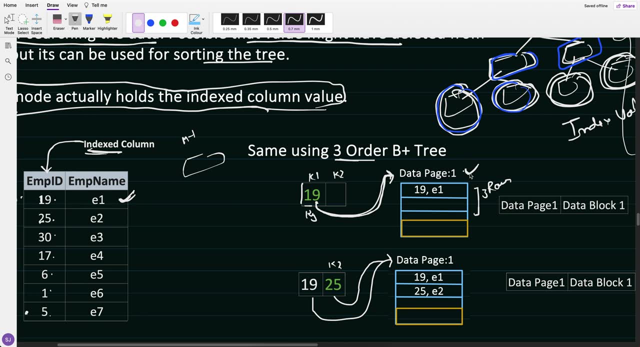 And let's say, this data page can only hold three rows. Can only hold three rows, Okay, so when I put 19.. So, DBMS, ultimately, actually, this is just our representation- DBMS, What ultimately has done is it created a data page, one is towards in this 19 even row. 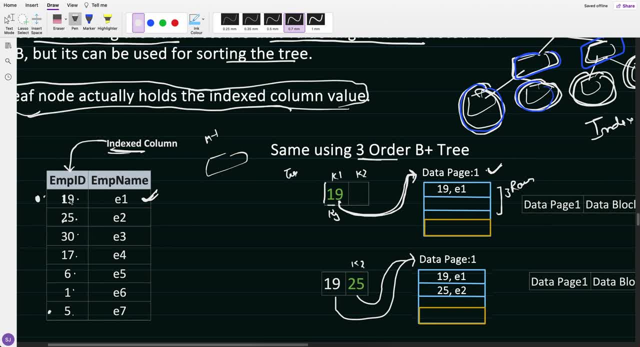 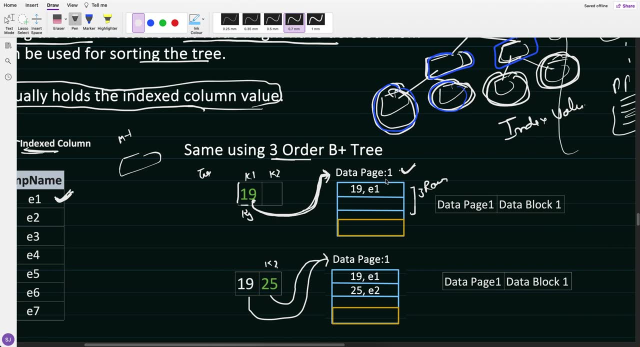 It created a B tree on this index column. It also, maintaining the index, put a 19 with this 19.. It also maintains one more pointer: that this 19 row belongs to this data page and also this data page ultimately has to be stored in some memory or data block. 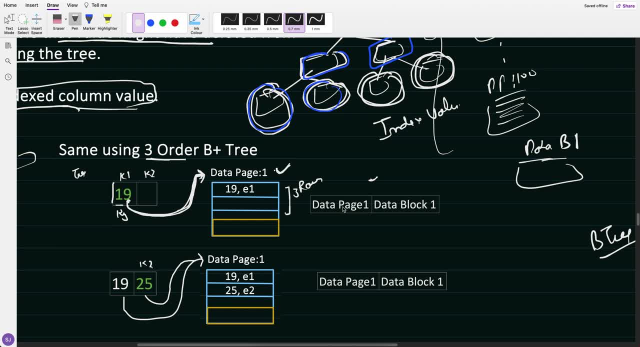 Let's say it is stored in one, So it is also now storing this data page one, data block stored in one. So this is the data page one in the disk. Okay, So now second row is inserted. So when second row is inserted, 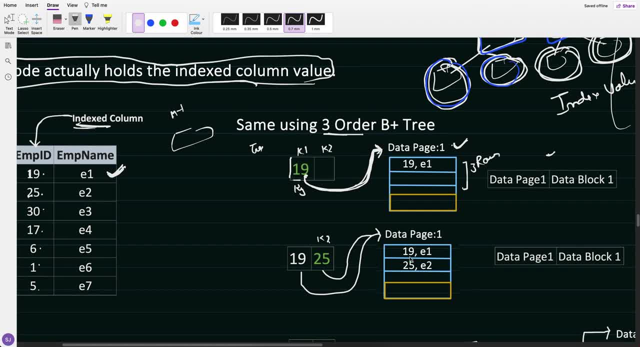 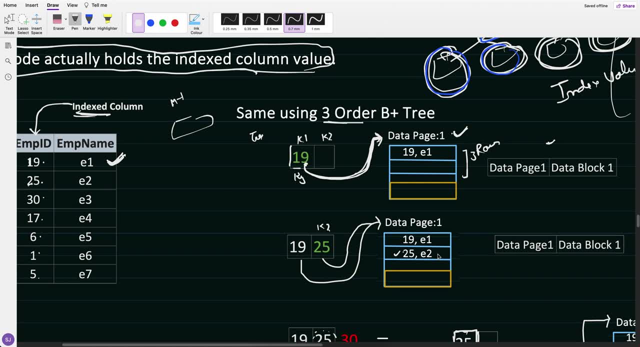 It is inserted where in the data page first. so data page second row is inserted because data page can hold three rows. It is only the second row. it inserted properly. Now it will update its indexing because new row is inserted right, it has to updated indexing. 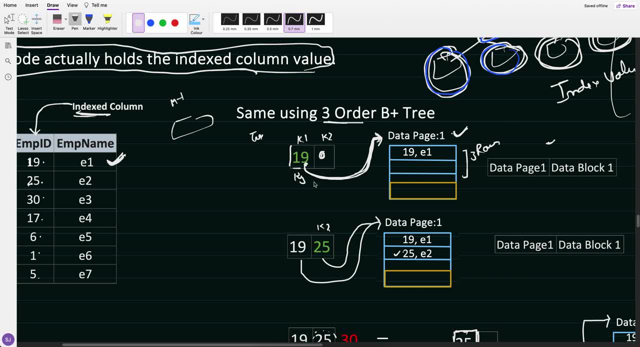 So it will check that. okay, one node is free, one key is free, So it will put 25 here And also manage one more pointer with it, And this pointer that 25 is stored in where data page one only. it put this pointer in which data page this 25 holds. this record holds: 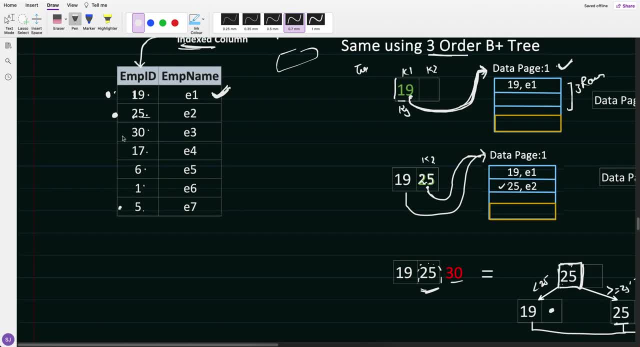 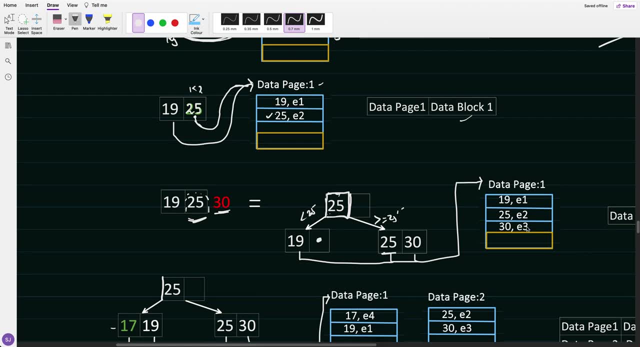 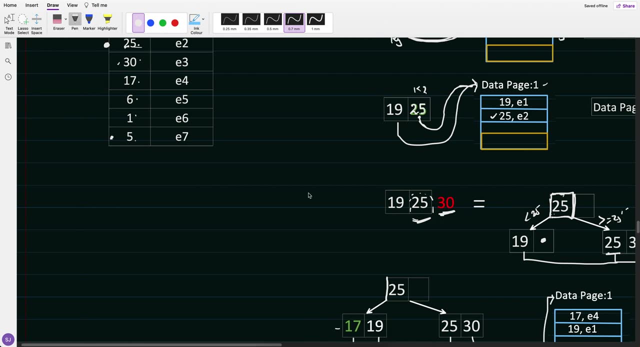 Right till now data pages in data block one only now 30. So when 30 is stored, so first it will be stored in the data page one only right. so because it has the space right, so you can or you can say that first. what it will do is it will try to see that. 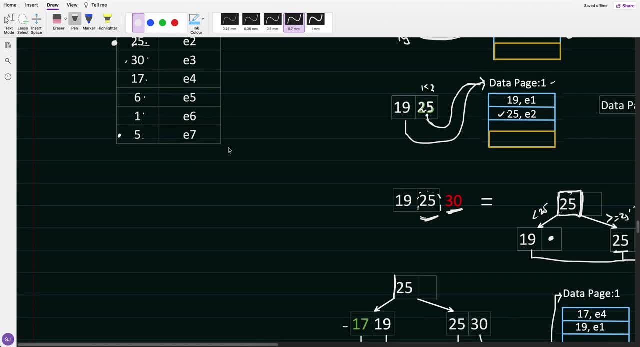 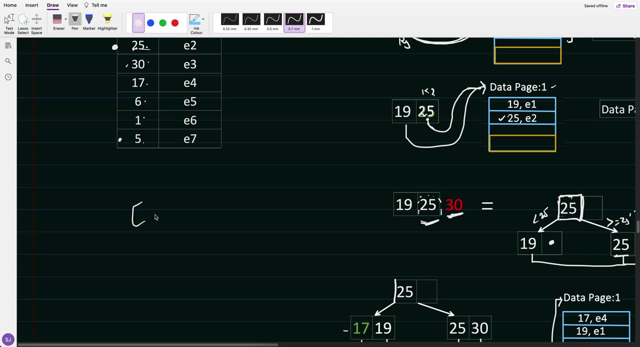 Which data page it has to pick, Right? So one more question: it has to comes to your mind that, hey, shansh, If there are so many data pages already exist, and when you inserting a new row, let's say we are inserting 30.. 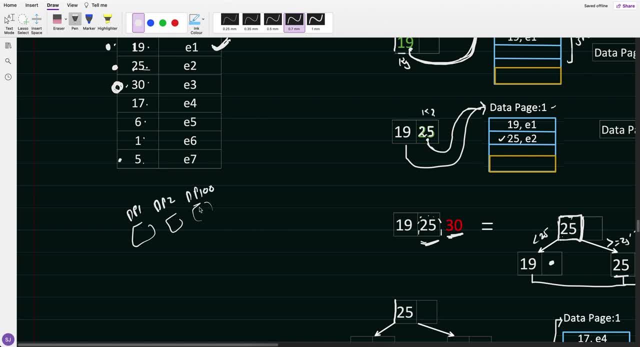 This is data page one. data page two. data page hundred: which data page to pick and insert? which data page? Right? This is a very interesting question that whenever you are insert a row, Which data page you will insert it? how DBMS knows it. 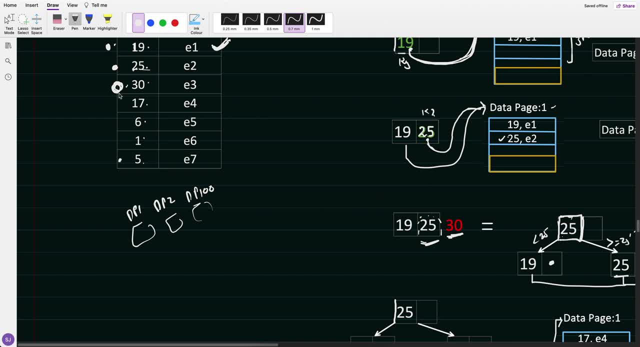 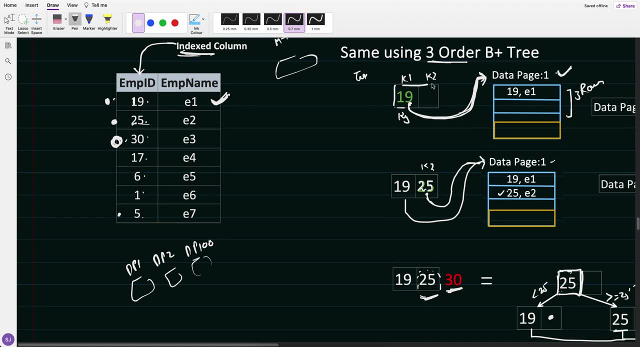 So this is how it knows this: through B tree only. So when I inserting a 30, so first it will goes that Tries to insert a 30 into the Tree B tree. So it will see that. okay, It will try to construct a tree. 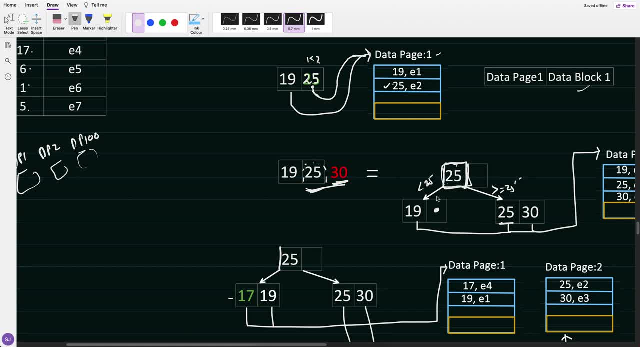 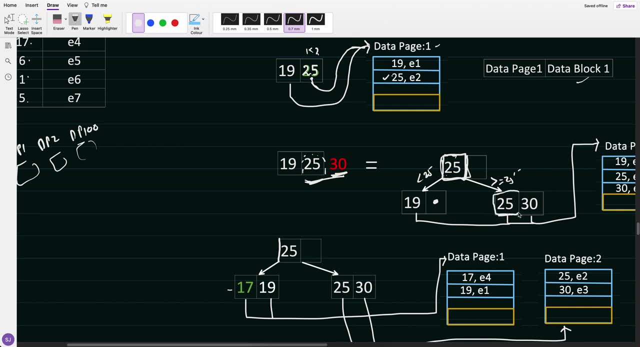 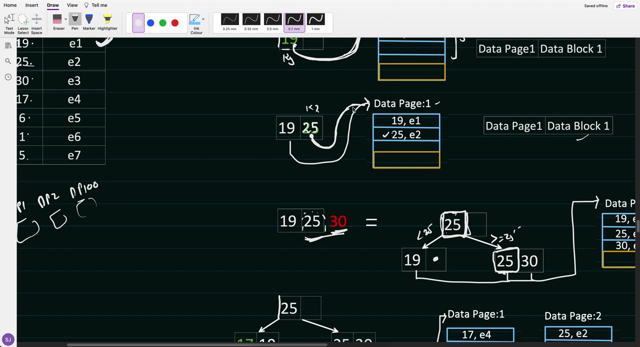 You already know that how we did it. So ultimately it gonna be look like 19 and here 25, 30. So what? it will see that, hey, my nearest Index is stored in which data page 25 was stored in Data page one. 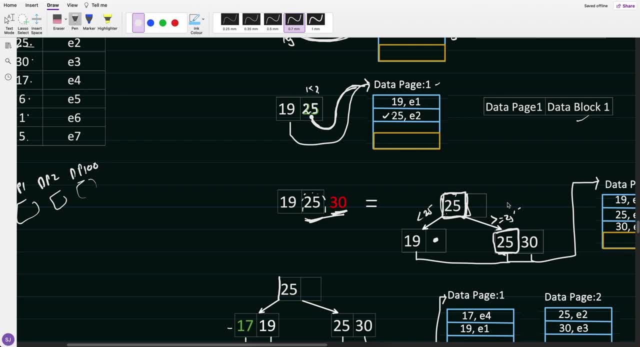 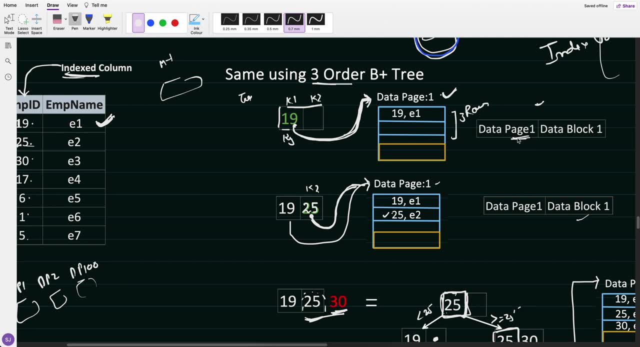 So what it will do is DBMS will try to load check the data page one right. So from its Data page one Memory it will check out its mapping database one. It is there in the data block one. It will load it. 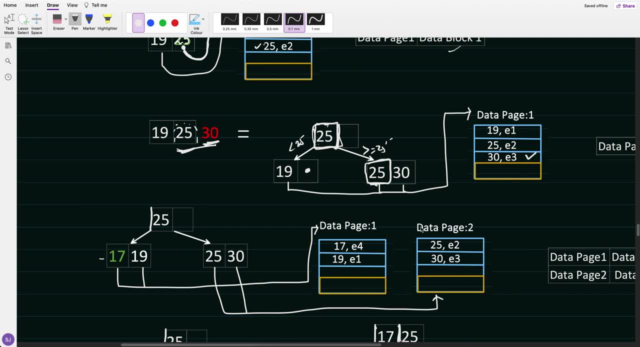 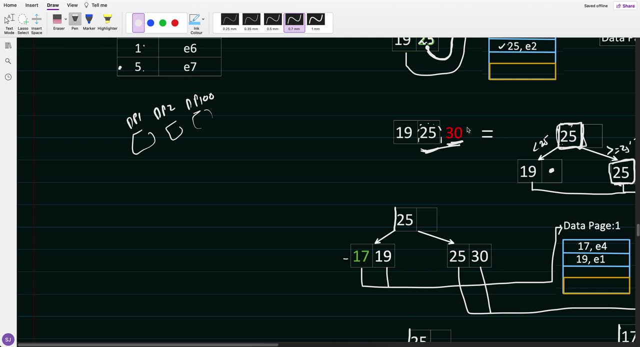 Right. and what it will put is This row and put it back into the data block. Right. and one more pointer it will store with 30 is that it is stored in Data page one. Got it. We will see one more example. 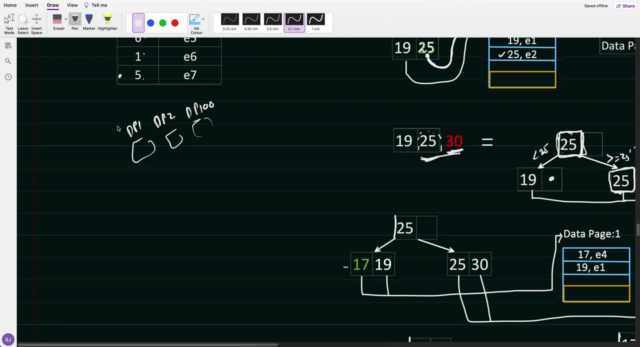 Now, let's say 17.. I want to store Now which data page. so let's say, if you have so many data pages with data page, It has to pick how it will determine. first It will go into This B tree. 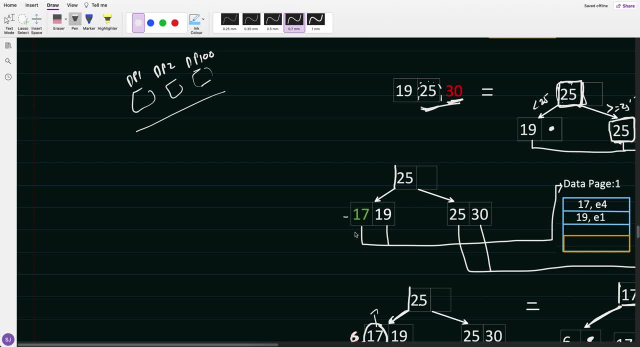 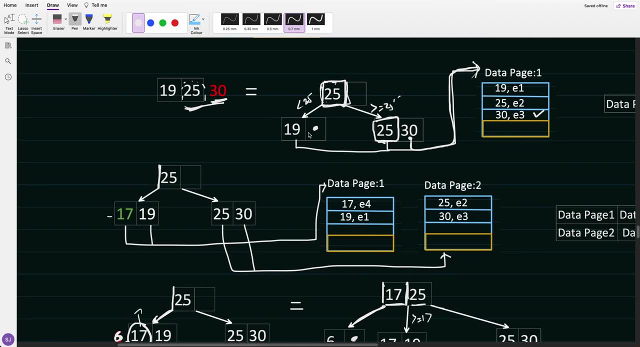 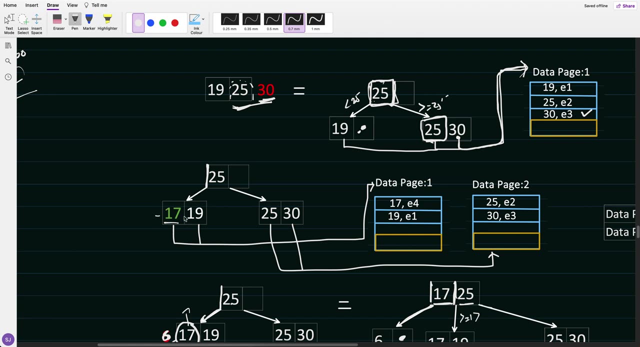 It will try to find out the correct logical Sequence of the 17.. So 17 is less than 25.. It goes here. There is a space available, So it will be stored here Now. it will check its neighbor index, that which data page it is stored, and it pick one of the very 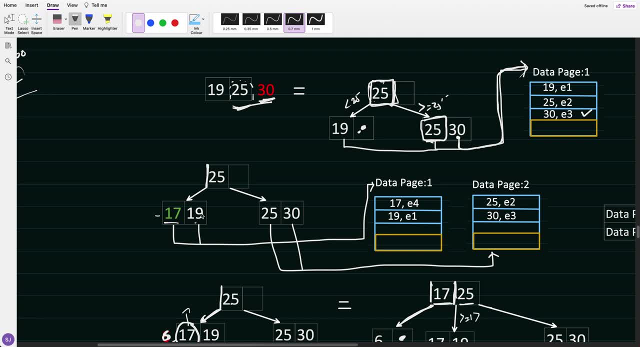 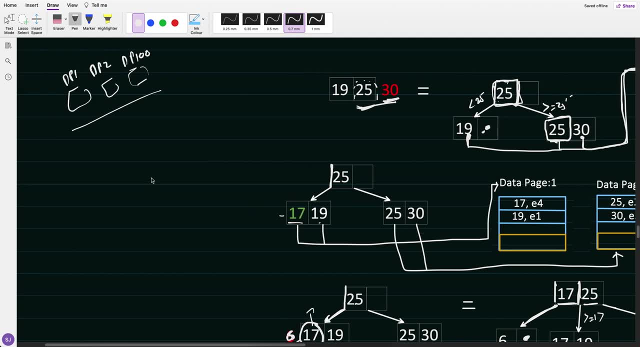 You can say that one of the data page, So 19, is stored where, so 19 is stored in data page one, right? So it will see that. Okay, Let me pick also data page one. So what it will do is DBMS will pick the data page one. 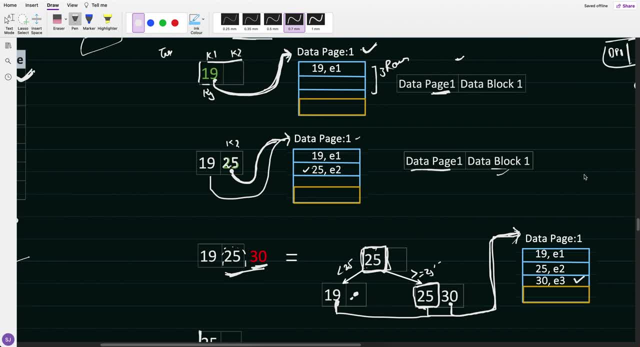 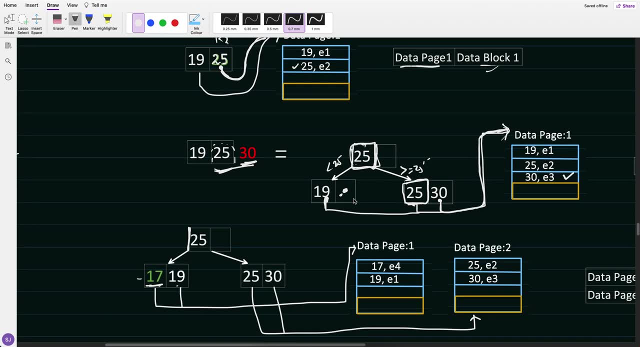 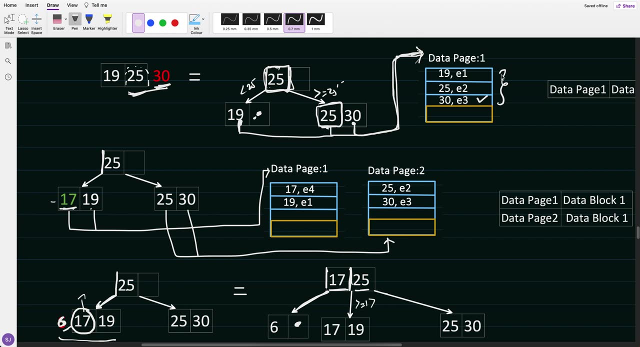 So data page one. It knows that it is stored in data block one. It will hit the goes to the memory loaded from the data block one. It loads the data page one now in the data page one. We already know that it is full three data. 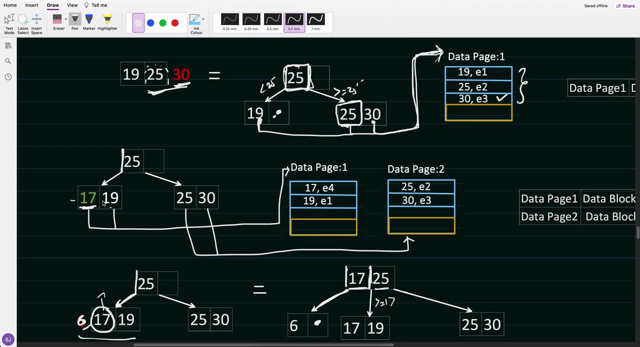 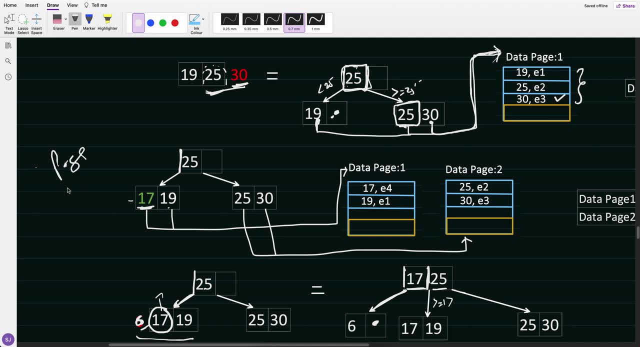 It already has. it cannot insert 17.. Now, what to do? Now, what it will do is DBMS will do page splitting. Page is splitting, So now, in the page is splitting, It will split. I create one more page, So it will create new page, page to right, and it will split the data. 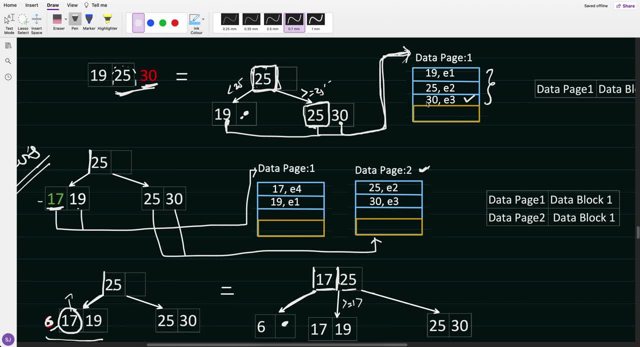 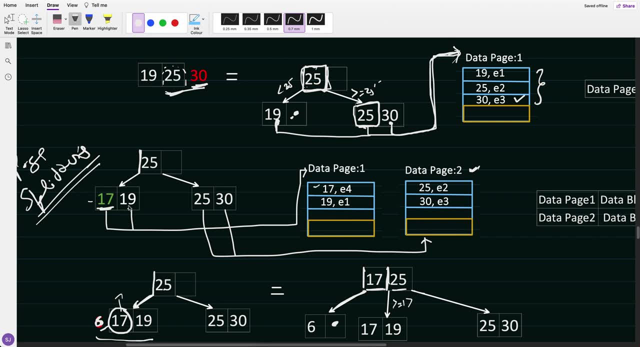 So earlier page one has 19, 25, 30, now 17 it has to store and now it will just split the data. So now let's say in page one It puts 17.. 19 rows data and in the page to it put rest of the data, whatever the page on. 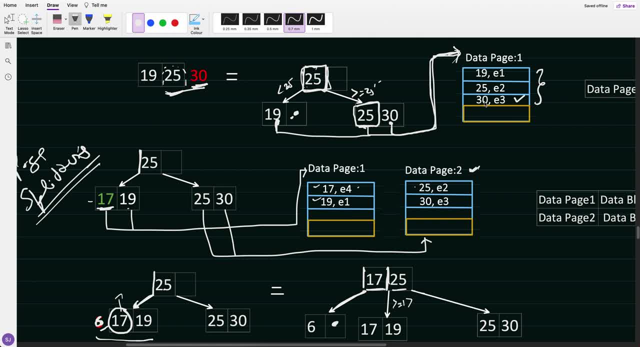 So page one has this three data right: 19, 25, 30. So whenever it pick a particular page, so it picked page one. page one has no space, So it now the page is splitting happen. So in the page is splitting, a new page is constructed and it divide the data of the page one plus this new data. 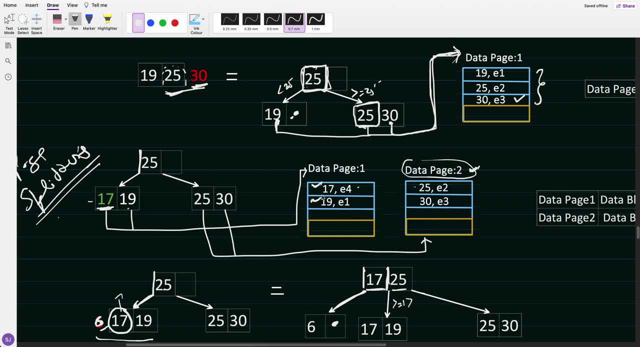 Right, So 17- 19. I have put into page one and 25- 30. I have put here in the page to right. It can be anything depending upon the DBMS and it will update the pointer. So now 17 will point to that. 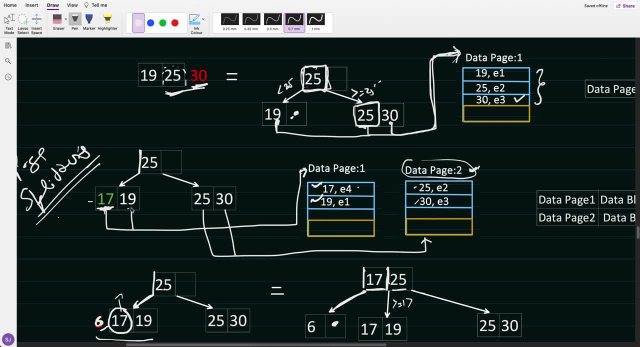 It is in page one 19. it will update its pointer that it is also in page one. Now it will update the pointer. 25 is present into page to 30. It updated that. it now it present into page to earlier. 30 was present into page one. 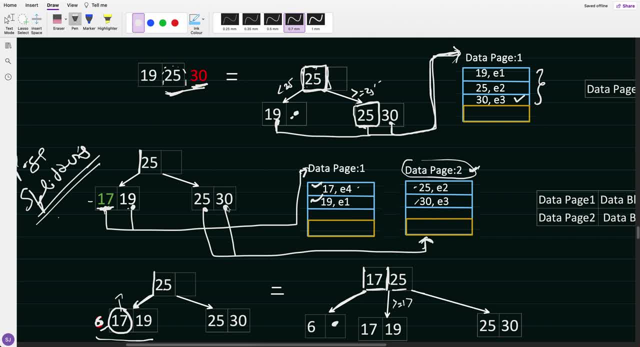 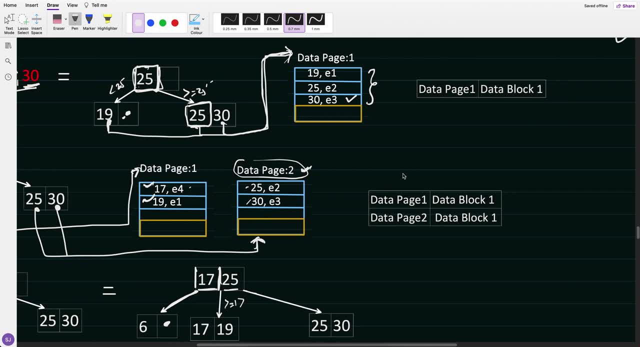 So it has to update the pointer. So it will update the pointer that this index value 30. It's all corresponding data is present into page two And also it will maintain a mapping that, hey, this page two is stored in, Let's say, data block one itself. 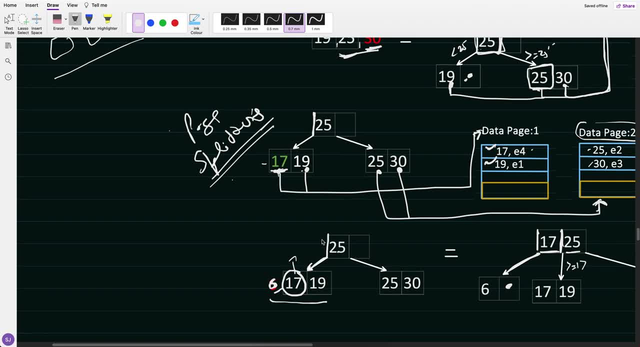 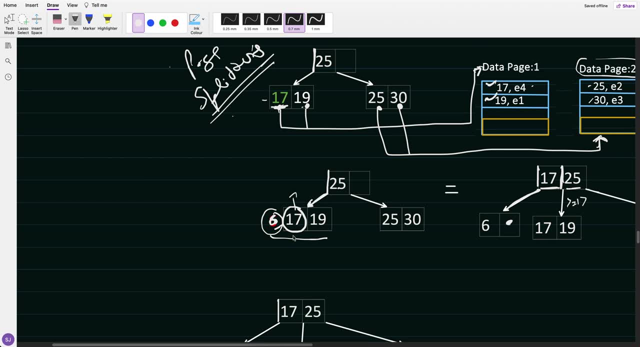 Okay now What data we have to store After 17,. let's say six. So it will try to insert a six. six will go here, Okay, So first it will try to identify its correct logical location. Okay, so it will find out. 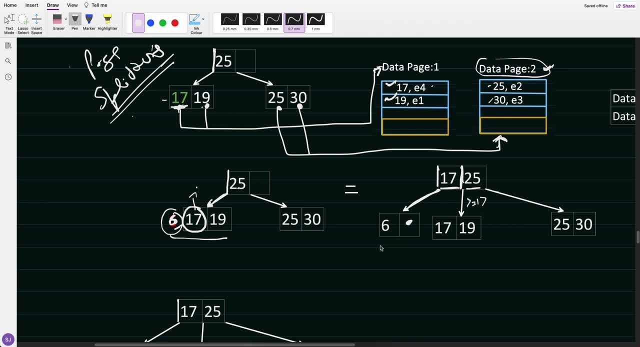 It's that okay. 17 has to be go up it find out its correct location. Now it will check its nearest neighbors nearest index in which database it has. So nearest is. all are linked in B plus three, I told you right, So it will check that. 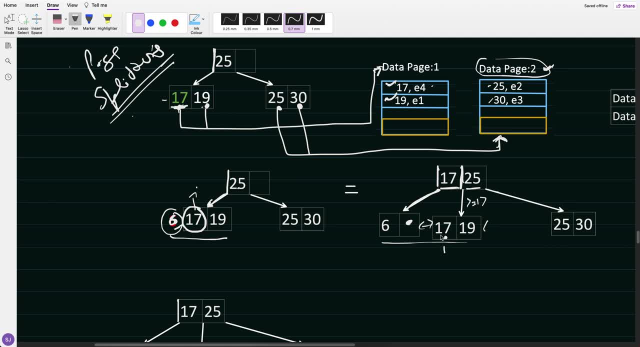 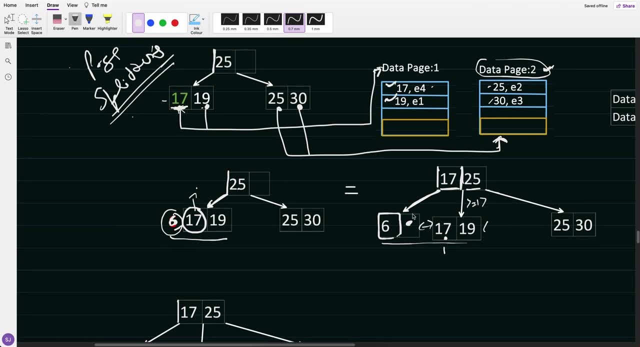 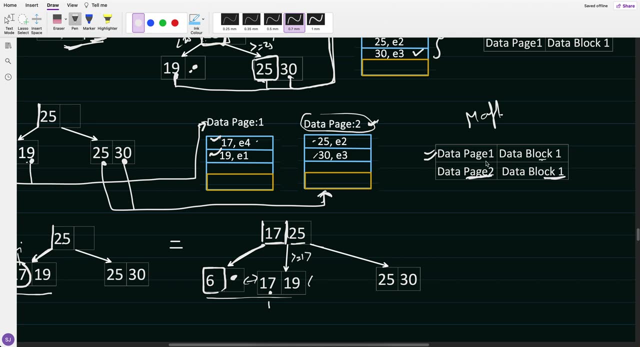 Okay, this 17. this 17 is stored in Page one. So it what it will try. it will try to insert the six into page one. So DBMS will load the page one. So from the physical memory it goes to a data block. one loads the page one. page one has now this two records: 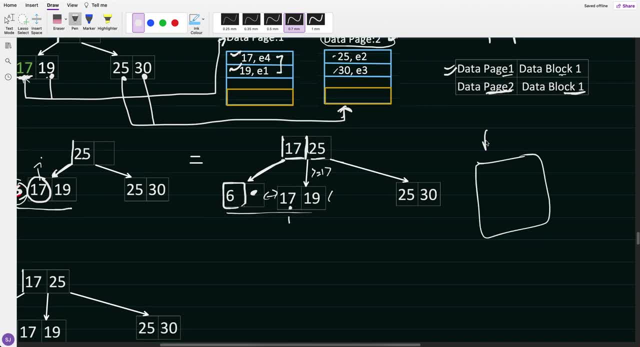 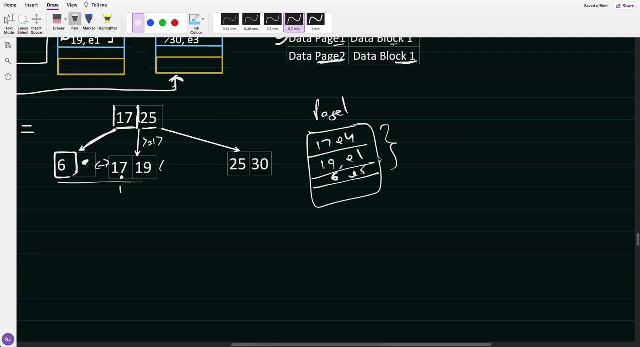 It will insert The page one. already has 17 e4.. 19 e1. it will restore the six also, because three we can store. so it will restore six and six data is e5.. E5. Right, and it will update the pointer of this to that it is stored in page one. 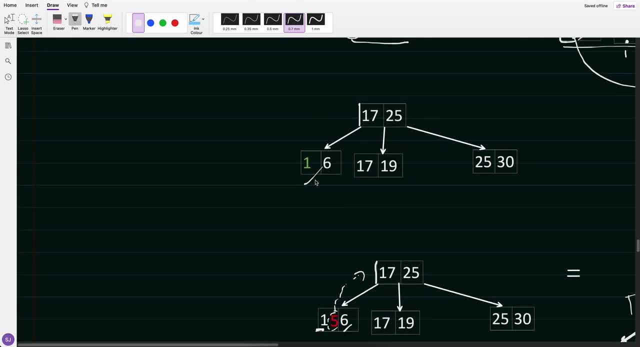 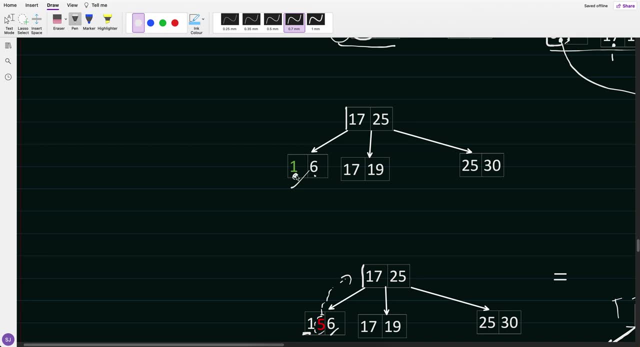 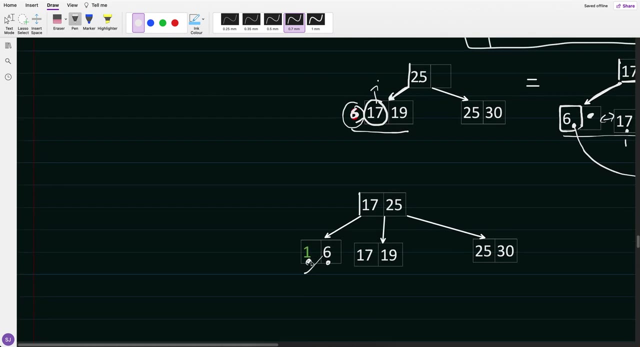 Similarly for one also. So ultimately, Once goes here, now here, Can you tell me one. When it goes to the one, one will see it's to his neighbor. He, which database you are stored in six, will say that he, I am stored in data page one. 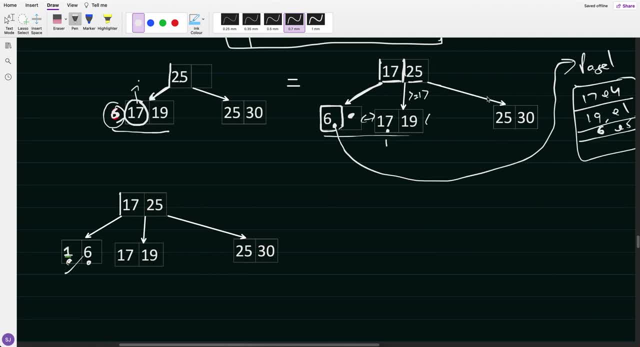 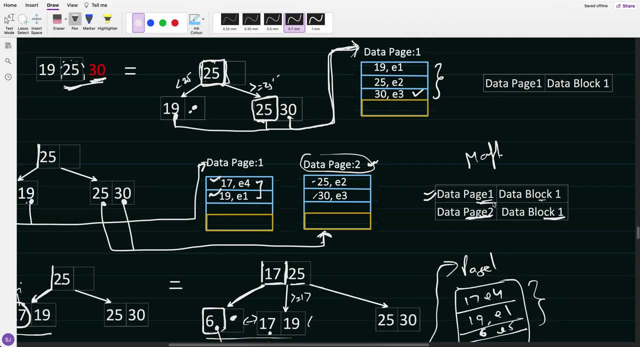 So DBMS will try to insert the one into also into the data page one, So it will load the data page one. It can easily load it that it has. the data page one is stored in block one, So now it will restore page one. 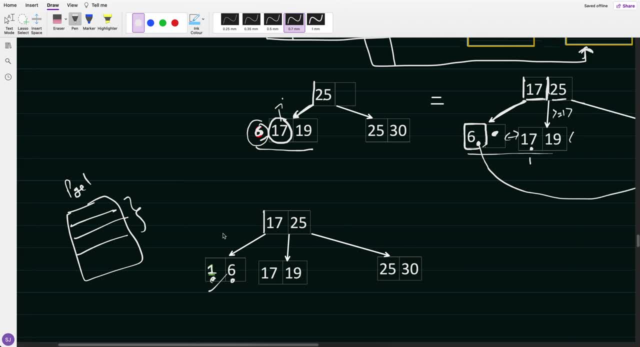 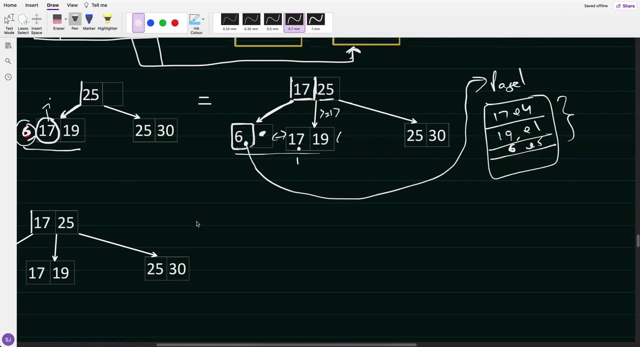 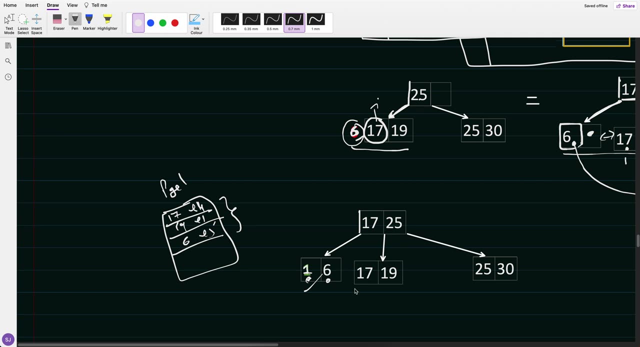 Page one already has three rows. It is totally full now: 17 19 6, 17 19 6 and it's data E4, E1, E5, E4, E1, E5. some data is already there. Now it try to insert one, but you can't insert one, right. 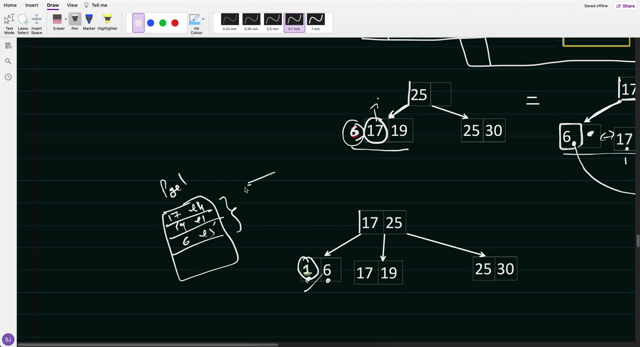 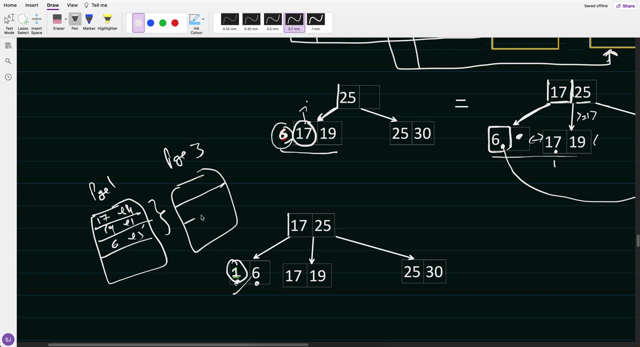 It's already full. So what will happen now? page is splitting, So it will create a new page. So page two was already there, So it will create, let's say, page three. It will now split the data, So let's say it 17, 19.. 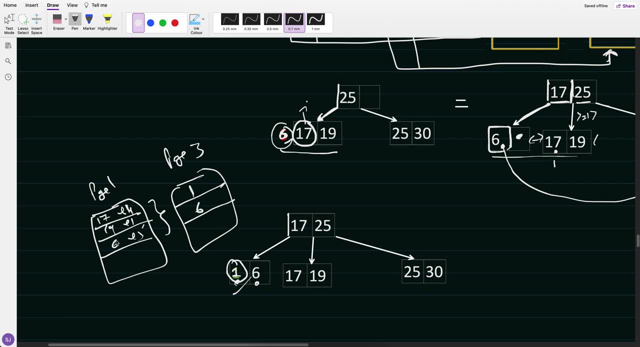 It will keep here and it will put, let's say, one and six here, One and six here, Right, and it will update the pointer. So one is now pointing to page three. Six is also now pointing to page three. It has to update the pointer. earlier six was pointing to page one now. 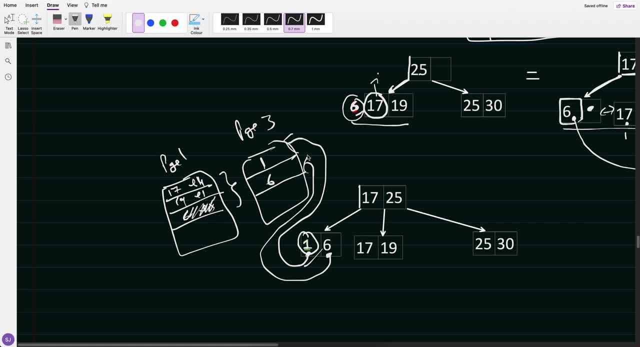 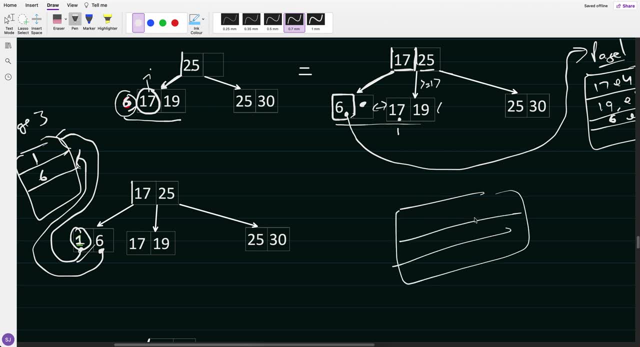 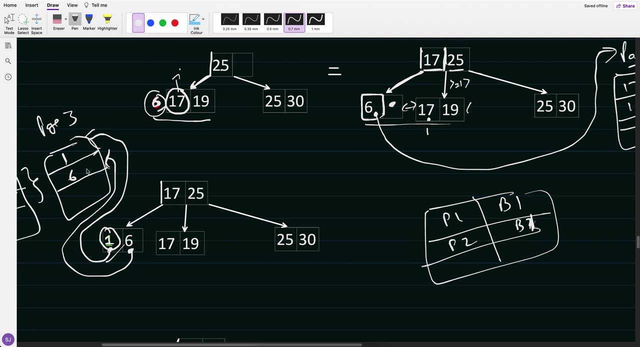 It has After splitting six has to points to page three Right and also it will add a new mapping also that Page one is there in block one, page two was there in block two, block one Now it will have. then let's say, page three goes into, let's say block two somewhere, while 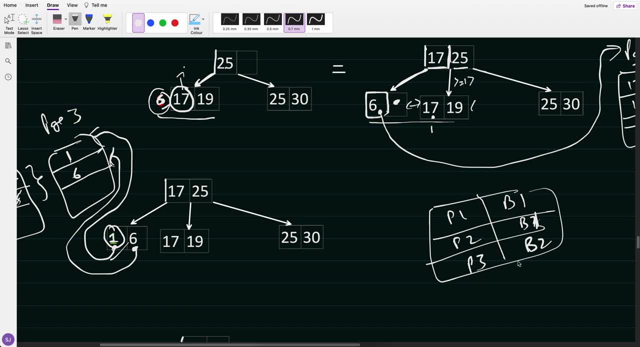 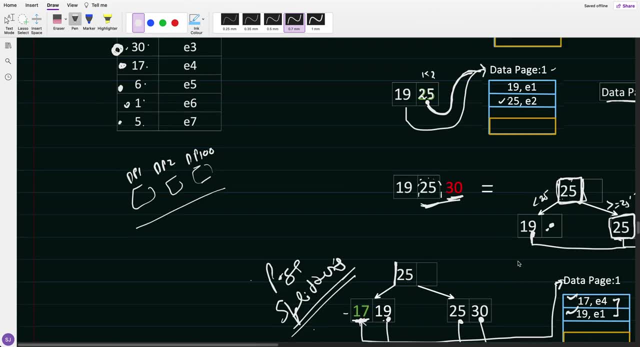 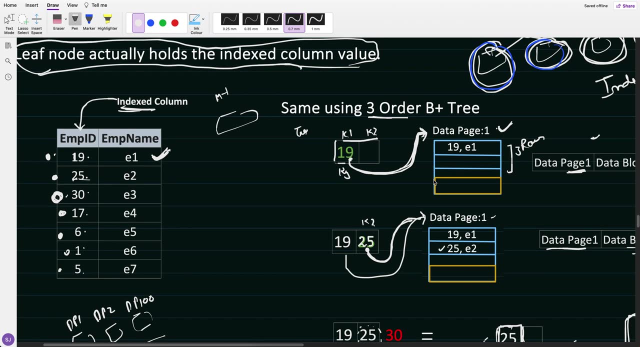 you're storing into the memory, It knows that in which block it goes. So it does the mapping. Now does everything Making sense to you that how everything is linked Right? one thing I still haven't tell you about this offset array. 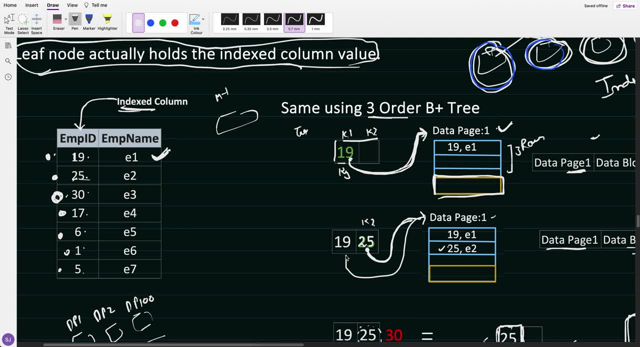 How this offset array is used. I will tell you when I tell you about clustered, non-clustered, but till now, tell me that in the comment section. Is it clear to you? I'm going very slow. You know right How the table data is actually stored in a 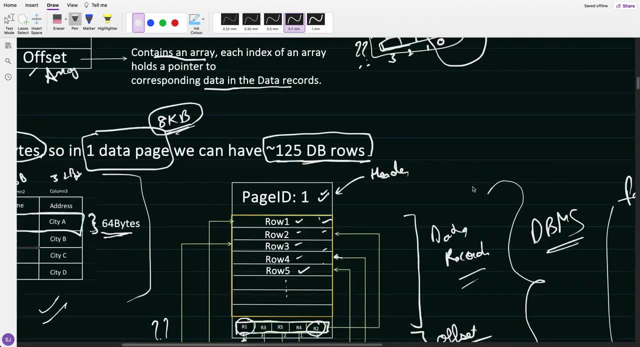 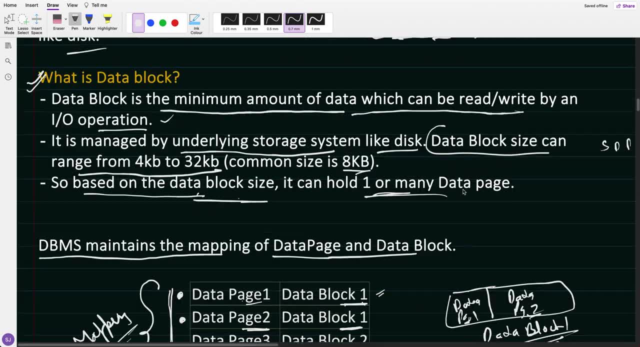 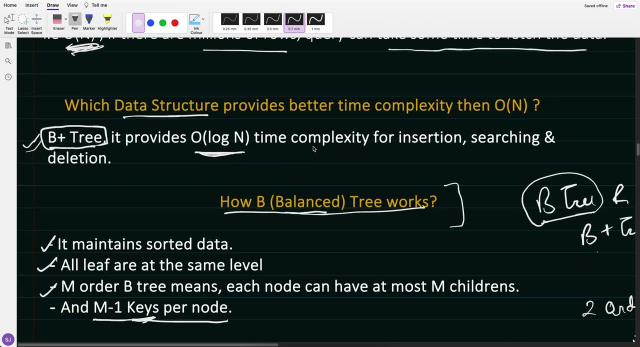 Page There can be. this page ultimately get stored into data blocks, So DBMS has to maintain The mapping Page versus block Right. Then For indexing B plus three. I think it should be clear to you. We have seen with an example. 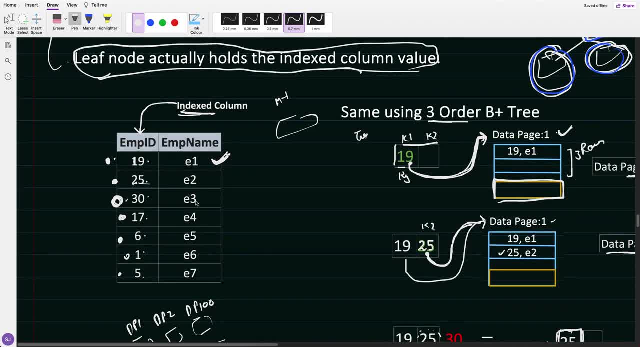 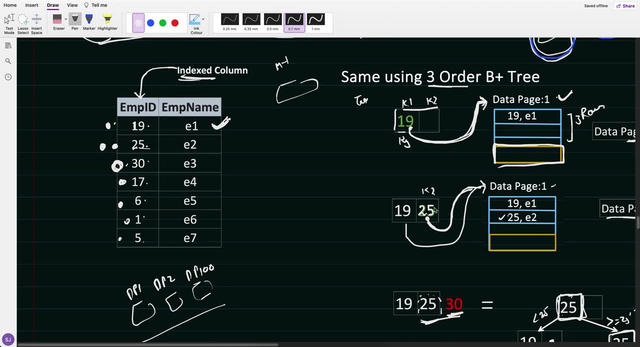 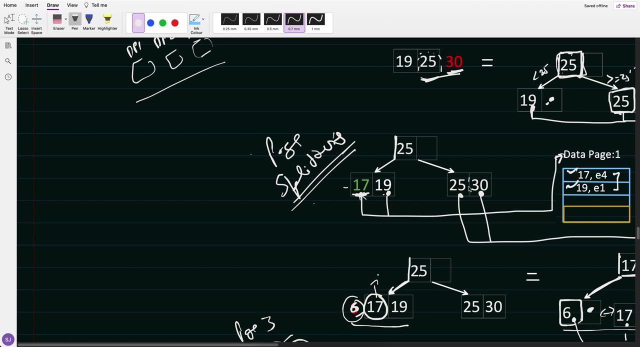 So whenever we insert a row, It first put its logical ordering into the B tree. Determine the best page It has to be stored, because there can be so many pages. determine the best page where this data has to be stored, Right. So we have seen an example that where the logical ordering is, it check. 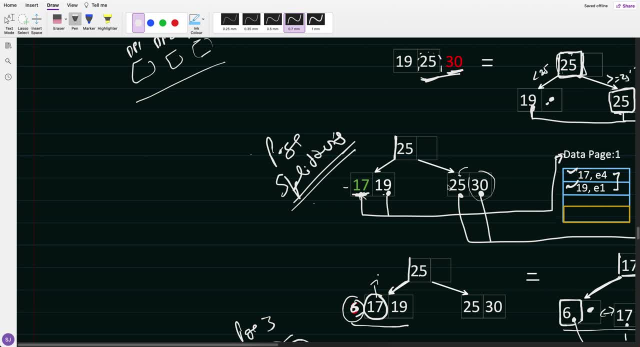 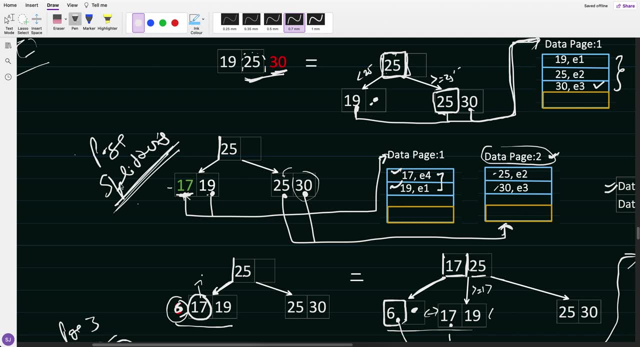 its neighbor. It tried to load that page and see if I can, if that can be accommodated in that page. If not, page splitting happen Whenever page is putting happen. a new page is created And it just split the data Right And it has to update the pointers. 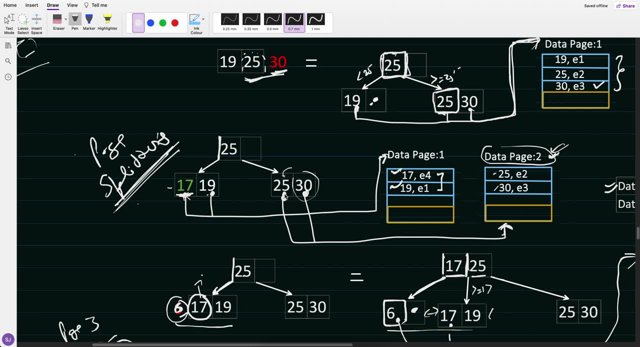 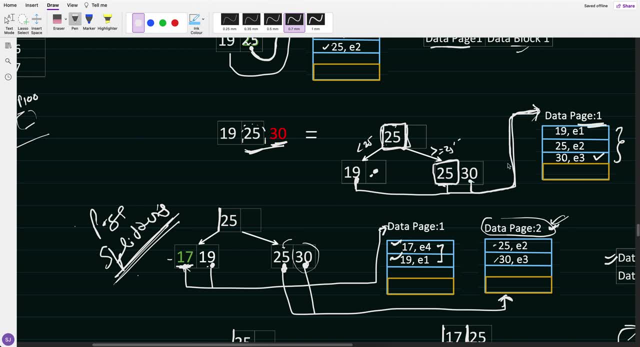 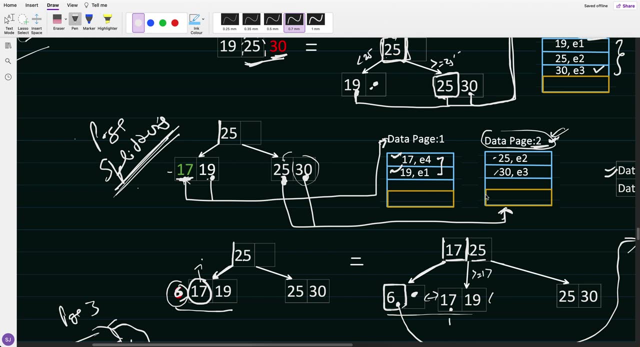 Also, It might be possible that earlier this Neighbor node 25.. Let's say it was a storing into Page one, but after the splitting 25 goes into page two. So this pointer has to be updated And whenever any new pages. 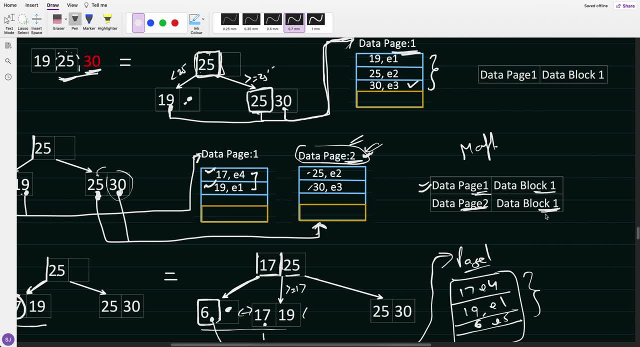 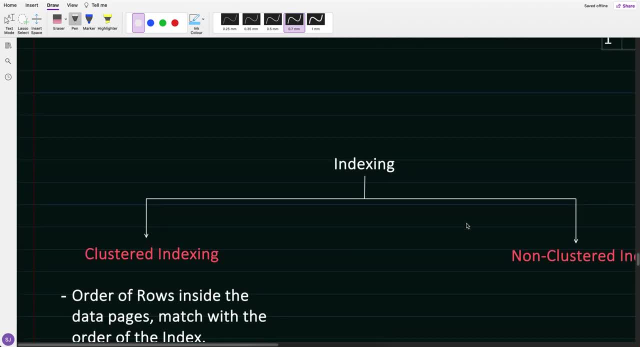 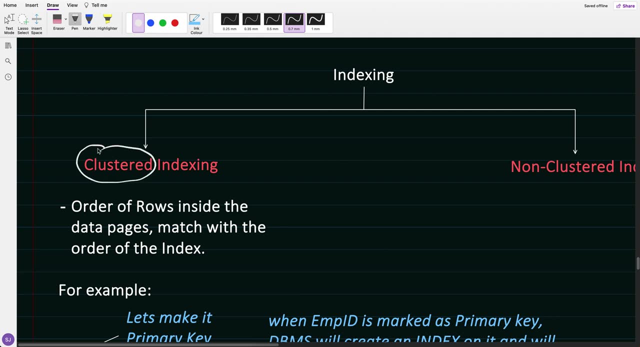 Is the stored When water. whatever the data block, it's ultimately inserted. DBMS has to maintain the mapping Clear till now. Cool, Now let's come back to the indexing part. Hey, what is the two type of indexing? clustered and non-cluster. 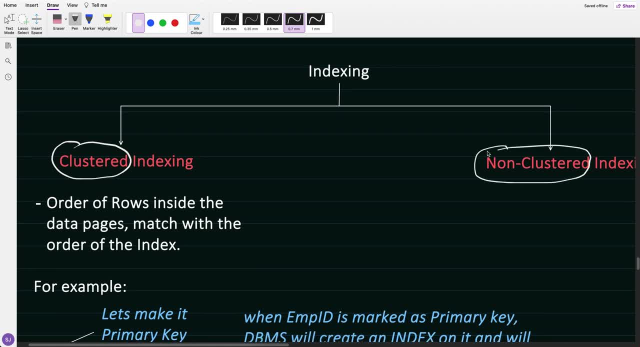 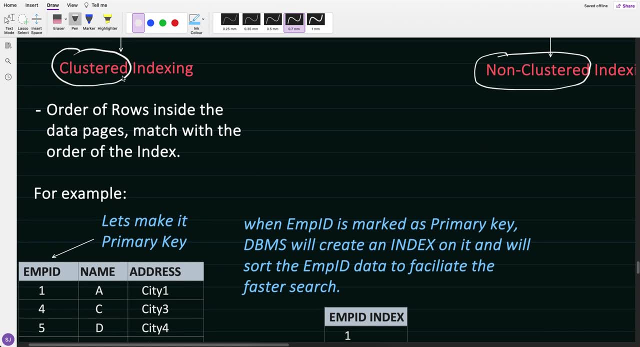 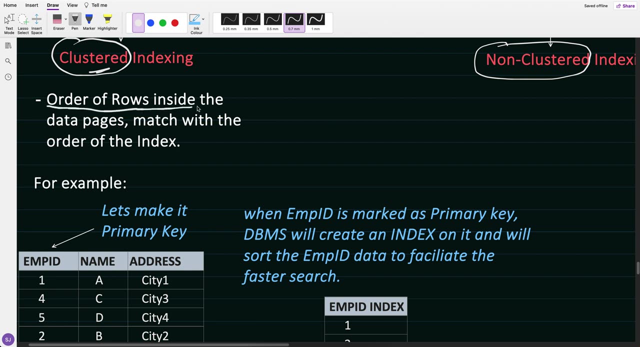 Now I know that what is how indexing, how DBMS actually does the indexing, but what are these two type of indexing? So see first, less understand the cluster indexing. cluster indexing says that order of rows inside the data page match with the order of the index. order of rows inside the data page match with the 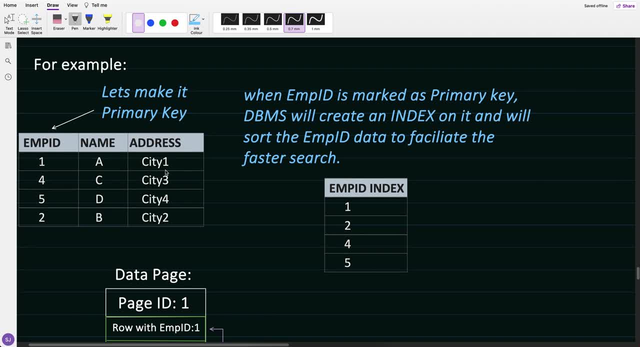 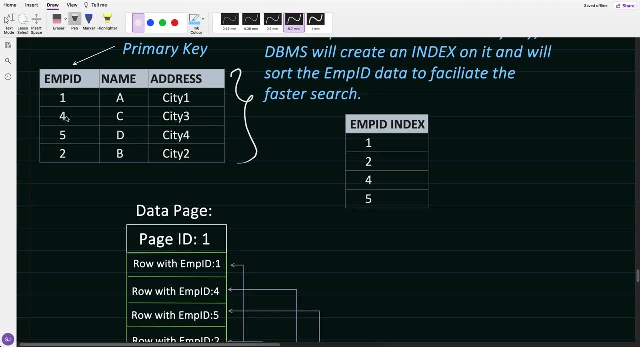 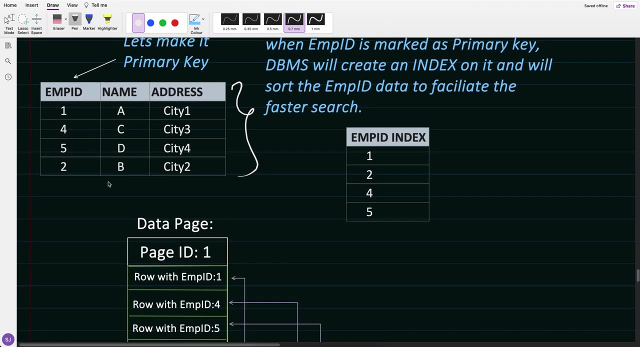 order of the index. Let's see with an example what I'm trying to say. So what But chance? so let's say: this is the table 1452, a CBD, and this is the address. Okay, so I told you at first that in the data page 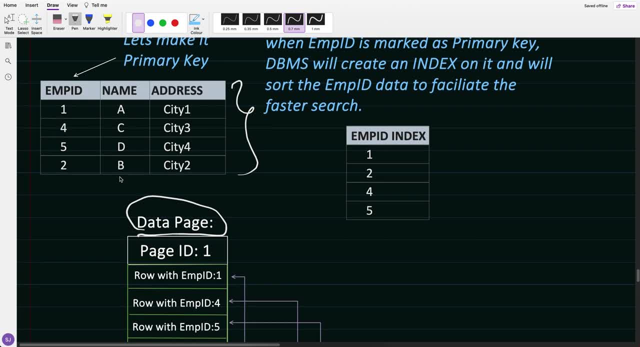 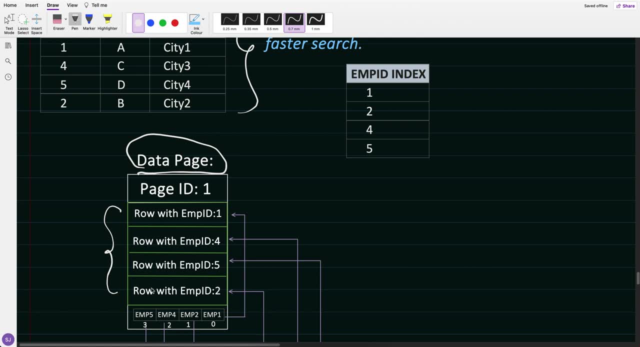 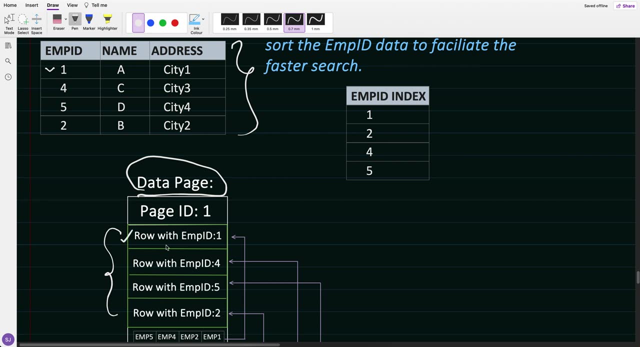 Whatever the sequence in which the rows are inserted into a table, generally in that order, only the rows are inserted into a page, only right. So if you are creating our employee ID one, so here in the data page, The, this row will come first. 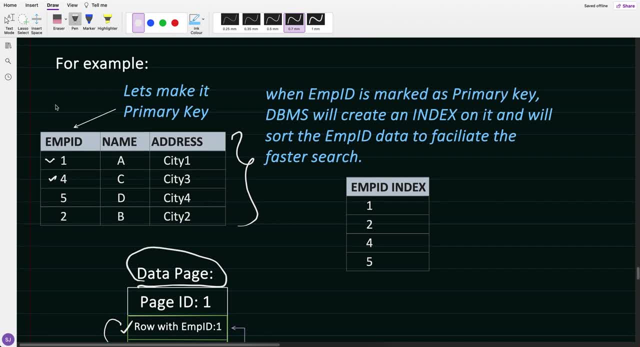 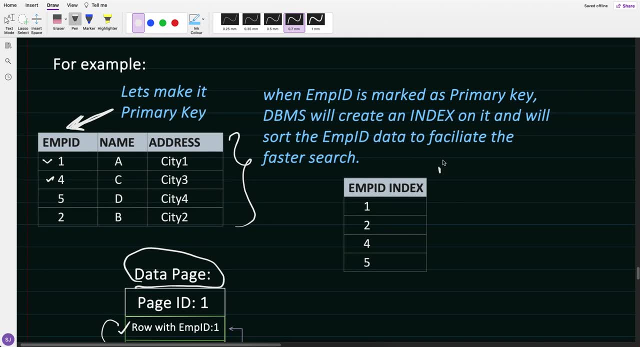 After 4, then 5, then 2. now, let's say I have put an index over here. Now you know that when you put an index, DBMS will do B tree On this index and it will have this sorted: 1, 2, 4, 5.. 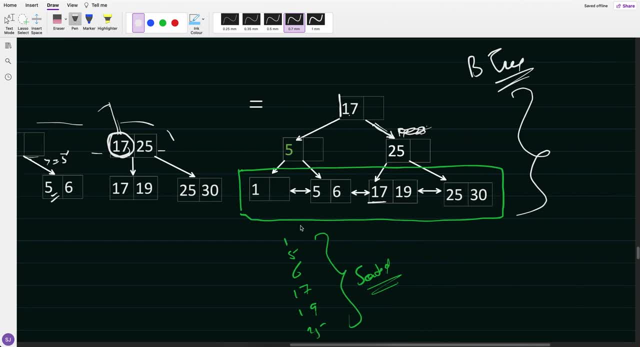 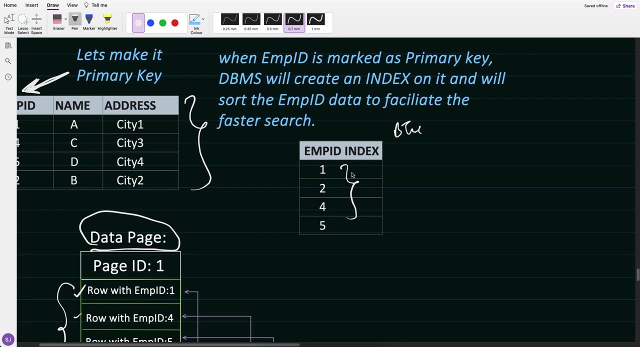 Now you know that right how: 1, 2, 4, 5, this at the base, It would be in sorted only and one will also hold a pointer to this. So when we say that right, one will hold a pointer to this one row. 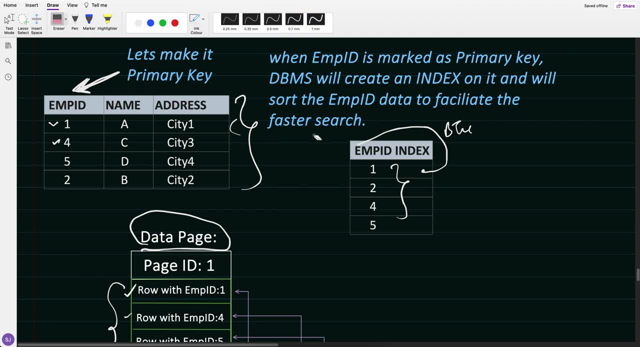 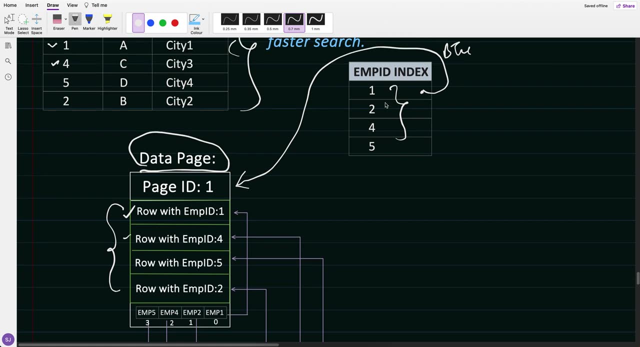 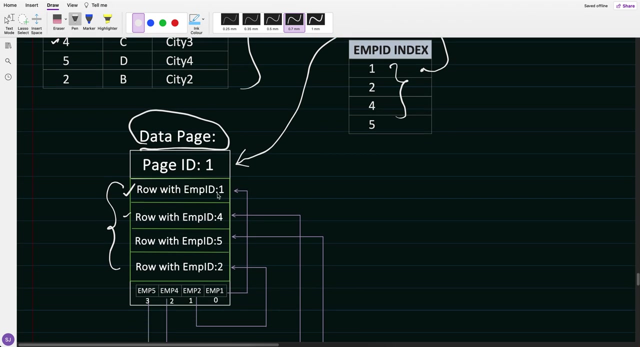 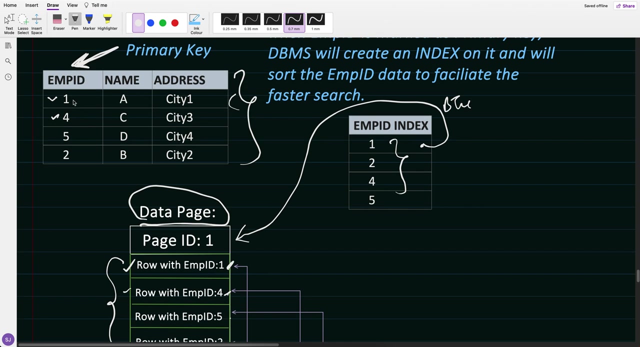 How ultimately actually this one will hold. point to Pointer to this page In which this row is present Right now. Here, the sequence, indexing sequence says that 1, 2, 4, 5.. And in the page Order is 1452. the way it is inserted, rows are inserted: 1452.. 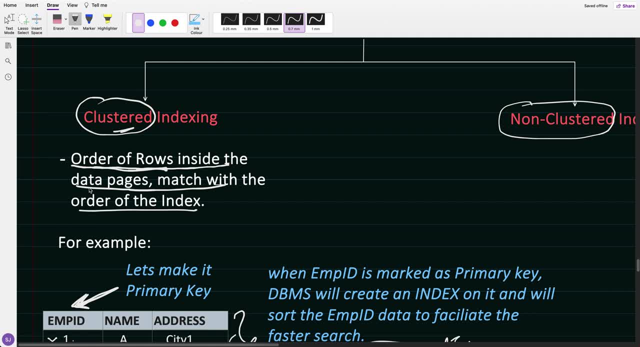 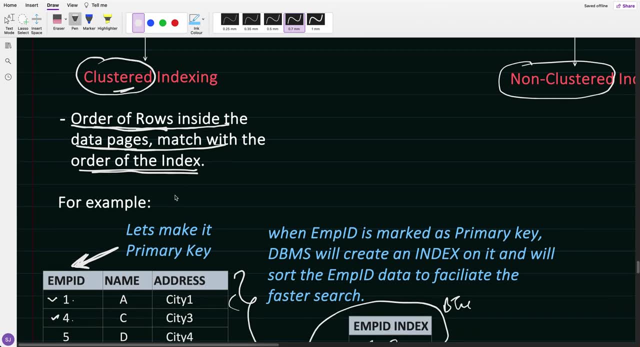 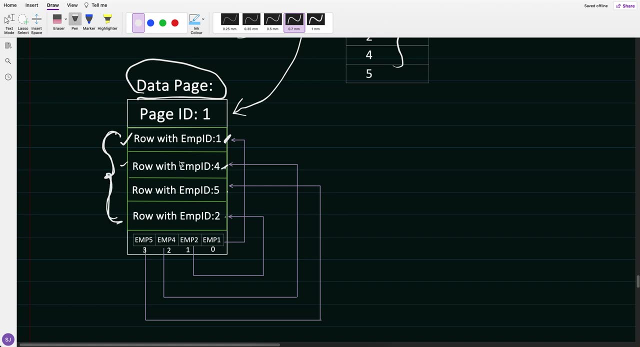 But hey, you are saying that the order of rows inside the data page match with the order of the index. That's what clustered indexing says: how we maintain the order. because you are saying that the order Of the rows which are inserted in a data page is depend upon how we insert. 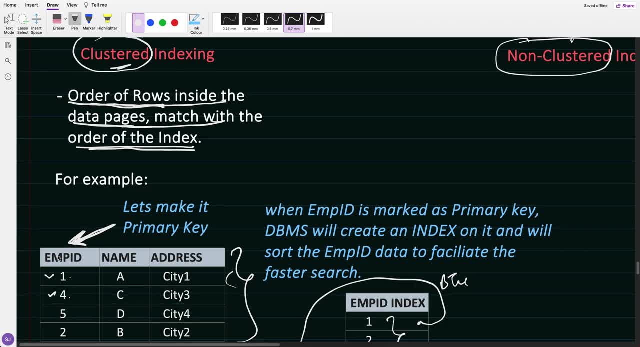 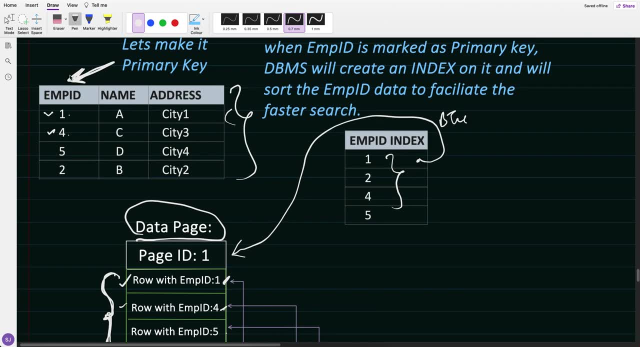 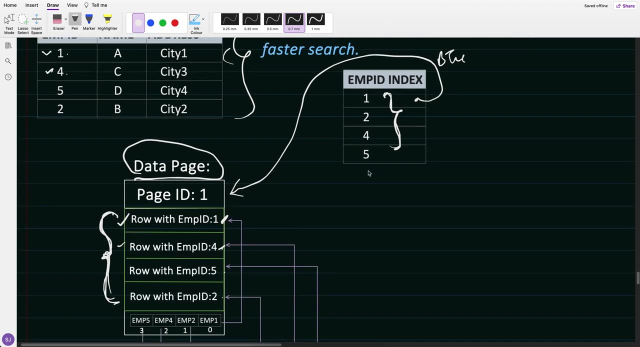 Inserted. actually Right, So we inserted 1452.. So it is stored like this: 1452.. But indexing on this column: indexing is in sorted order, So it should be 1, 2, 4, 5.. So the order of the rows should be 1, 2, 4, 5.. 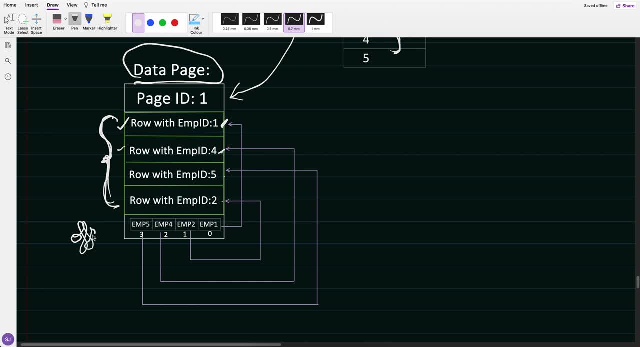 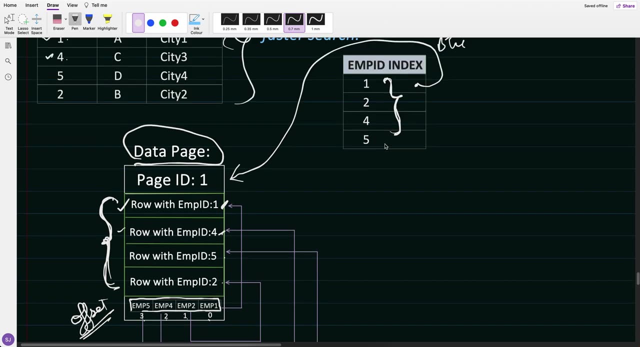 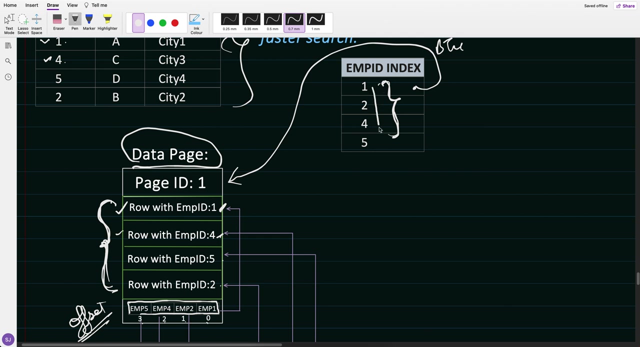 How. That's where the offset comes into the picture. I told you that in offset it maintain an array Right And it has an array like 0, 1, 2, 3.. So, whatever the index, Whatever the indexing Are you ordering is so indexing ordering is 1, 2, 4, 5, sequential. 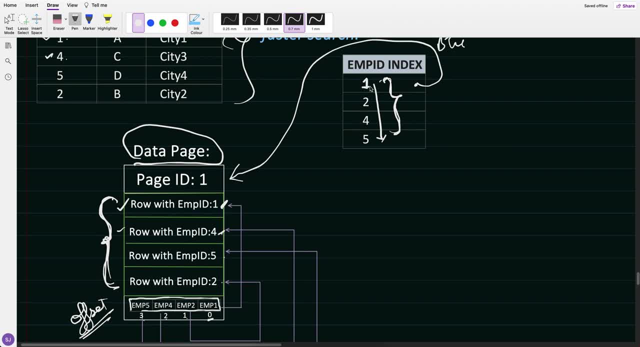 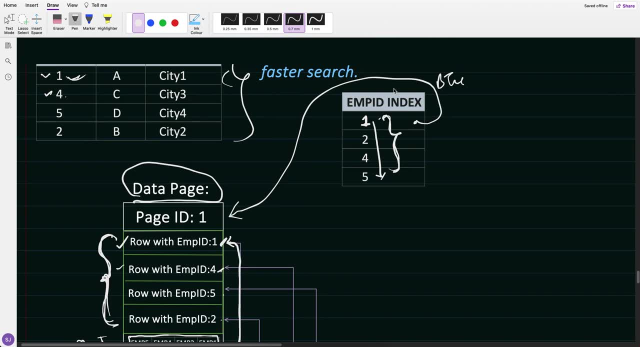 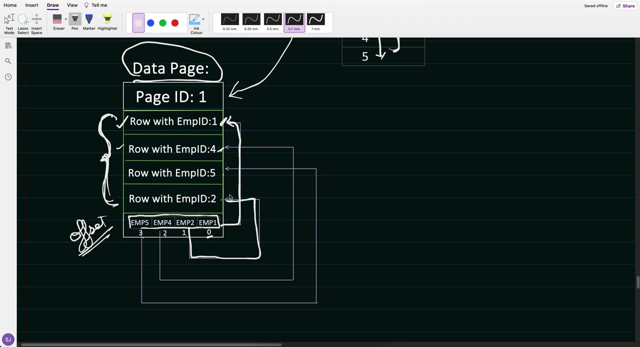 So at index 0 it would be, it would point to Employee ID 1 data, So it will point to employee ID 1 data, And then after the 2, so index 1, it will point to employee 2 data, 2 data. 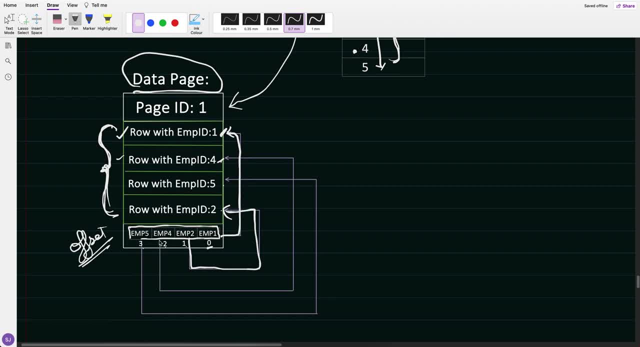 So third would be 4.. So and the next in the sequence of the array would be 4.. So now you see that, even though the data pages, the rows inside the data pages, are jumbled or depend upon how the user, I might have inserted mix mode. 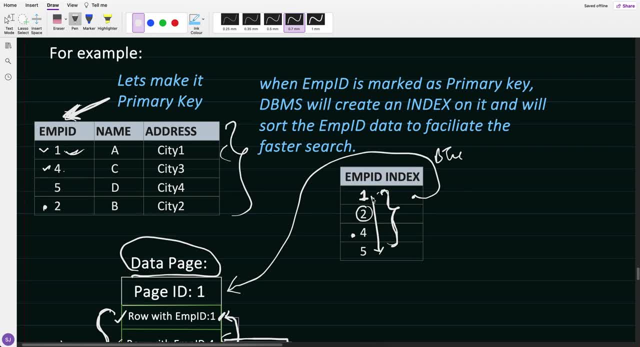 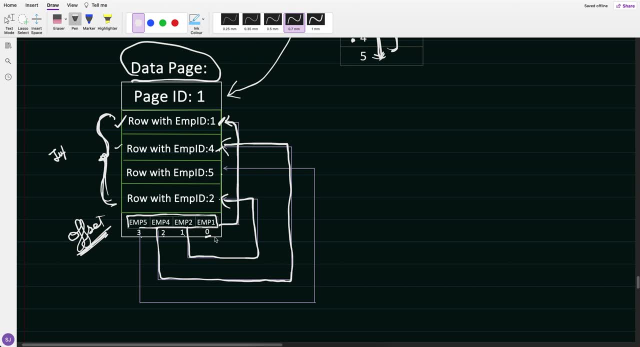 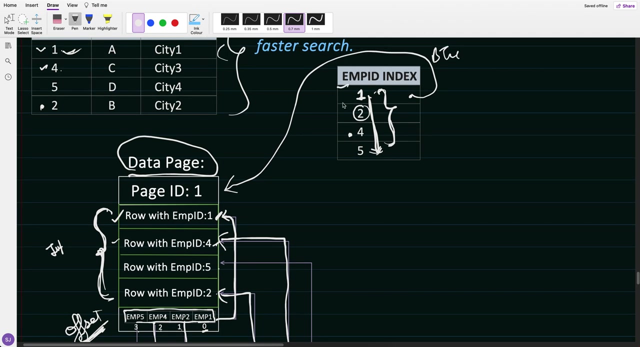 After indexing, Whatever the sequence comes out, The order is generally given by the offset. So whenever the you will Towers this pages, you will traverse in this sequence of this offset: So employee. so at 0 slot it is employee 1, then 2, then 4, then 5. 1, 2, 4, 5, like sequencing. 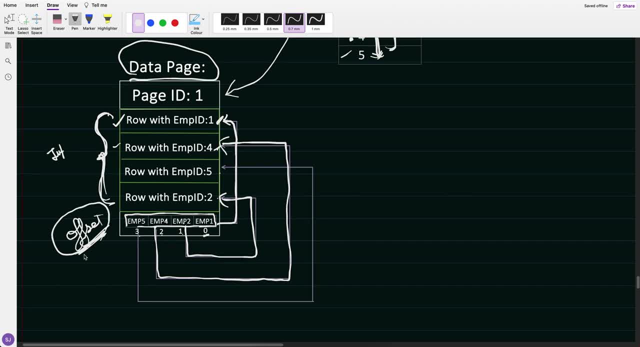 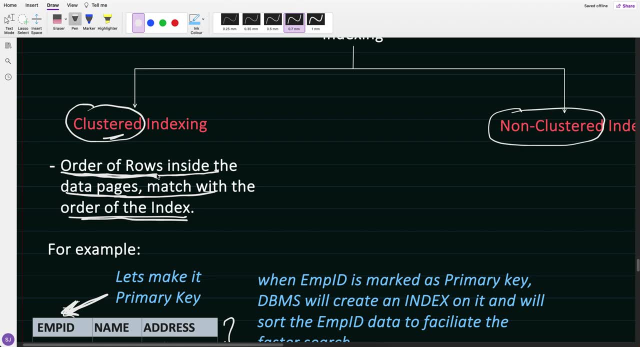 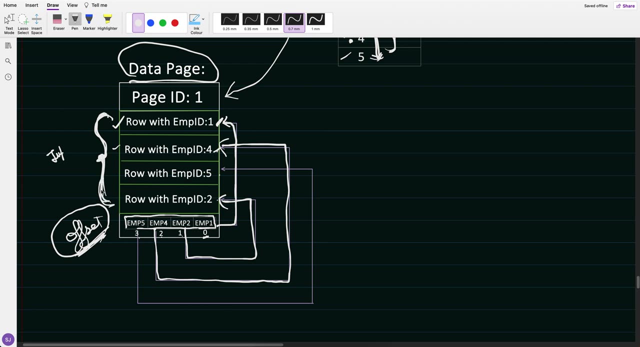 Understood that the Useness of this offset. it holds a pointer, And that's where cluster indexing is, that the order of rows inside the data pages match with the order of the indexing. So it doesn't mean that this rows are sequencing is changed. 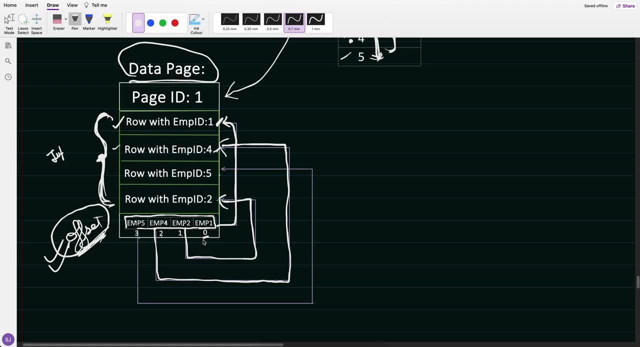 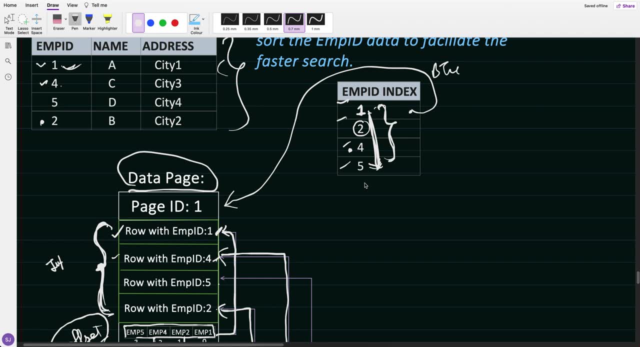 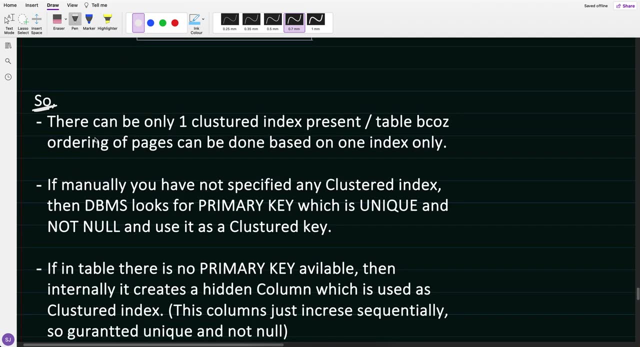 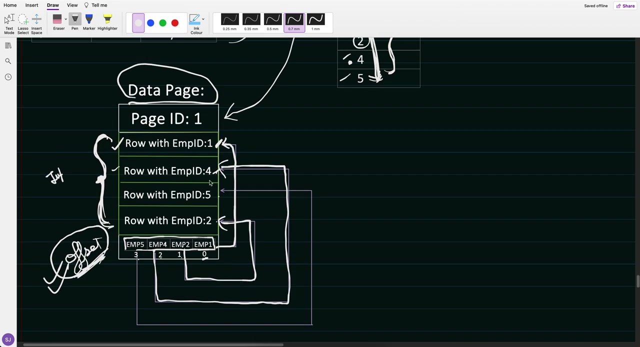 This offset is changed. This offset array holds the data in this manner so that it maintain the indexing sequencing. Okay, So There can be only one clustered index per table. Why? because you can create an order of a rows based on one index only, right. 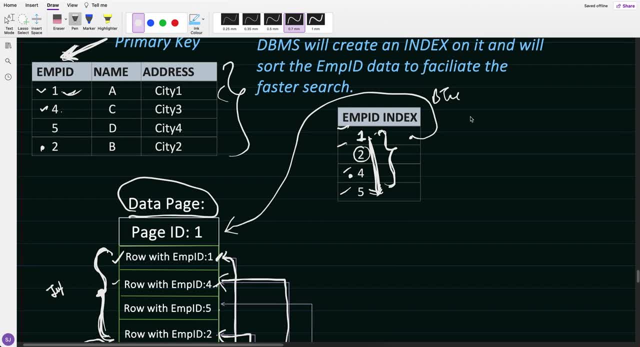 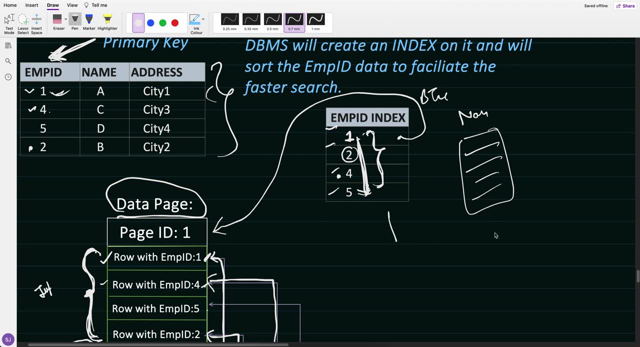 So now let's say this is employer, This is employee ID. Let's say name: Can a cluster index can be made on to employee ID and name: A, C, D, B. Let's say indexes. Let's say for this: A, B, C, D. 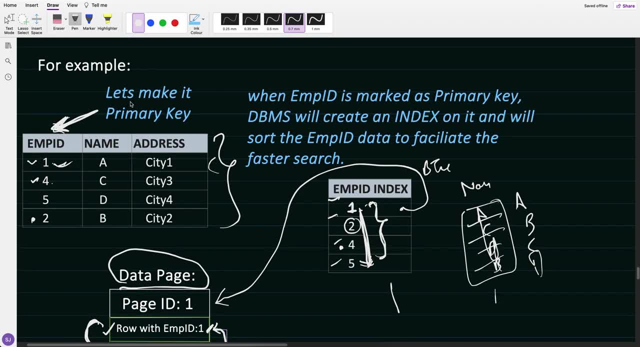 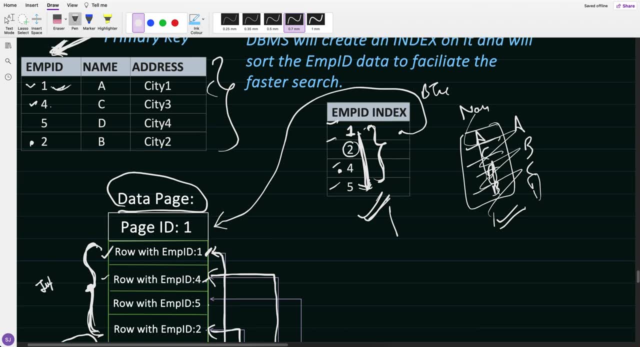 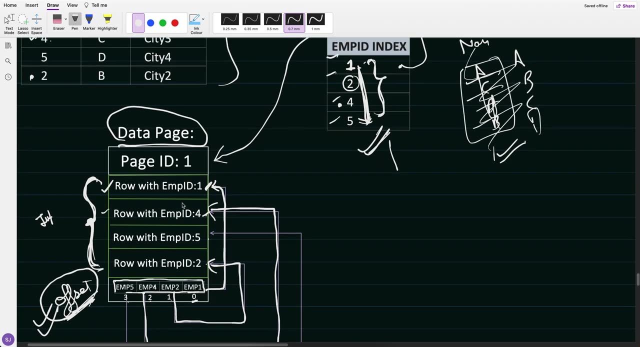 Right, but In the cluster index the order has to be maintained. So order can be maintained either through this or through this. So that's why they're in a DB. in a one table There can be only one clustered index. So what column can be a clustered index? 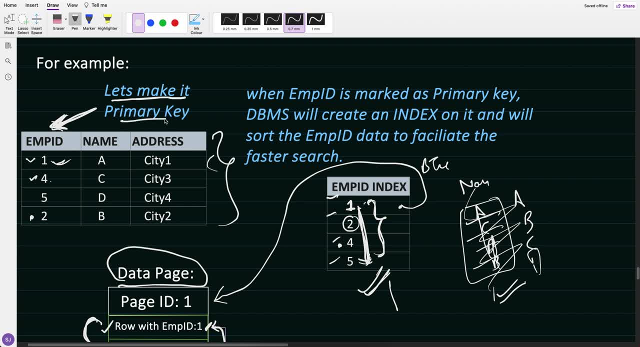 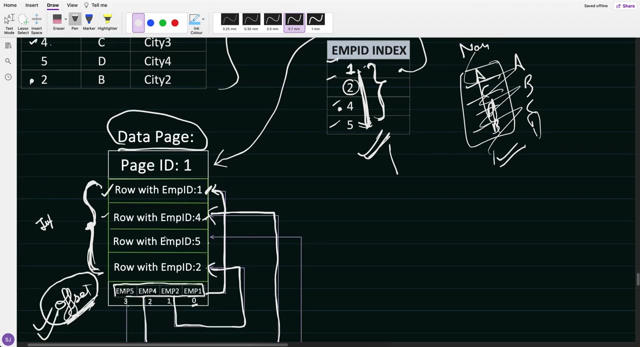 So the it give a prime, first priority to the primary key. So in this table, let's say, if I have created an employee ID as a primary Key, DBMS used is as a clustered key And whenever it use it as a clustered key it will sort the data pages based on that one. 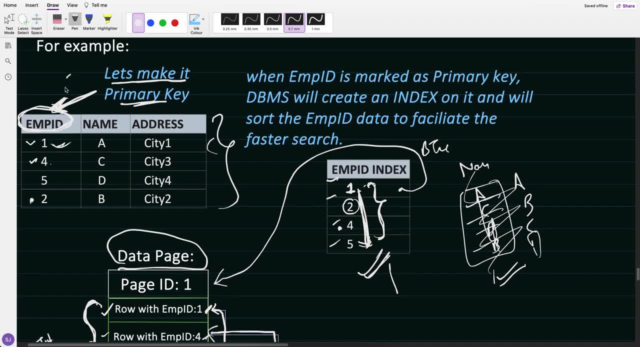 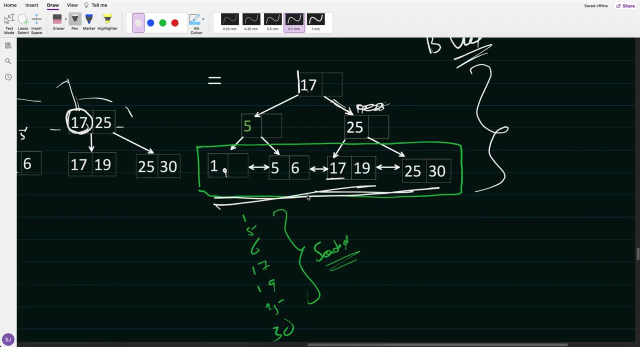 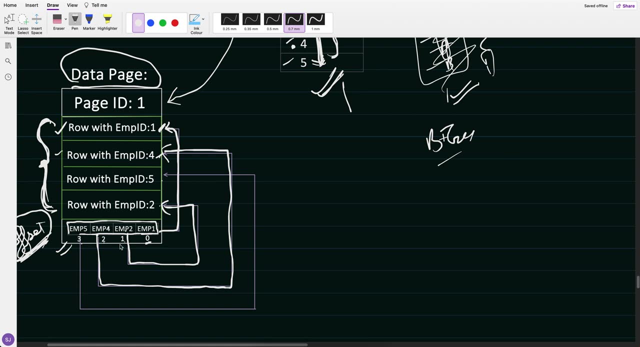 Whatever the index comes. So based on this clustered key, it creates a B tree, B plus 3 and whatever the B plus 3, ultimately the index sequence comes, The data pages also. it will insert in the same manner Like: Do not this offset the offset. 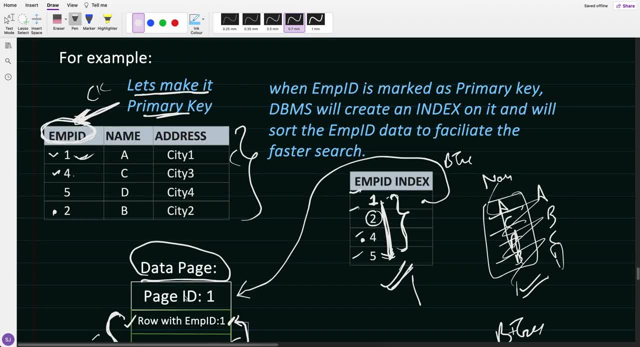 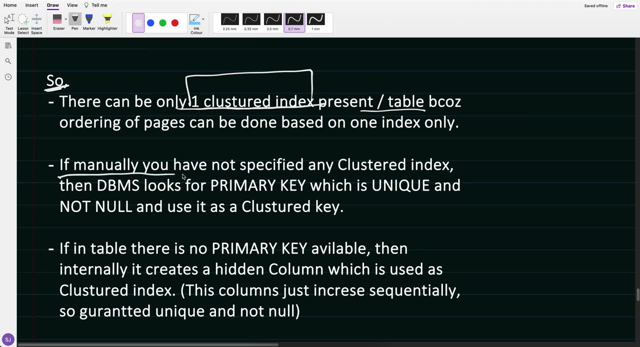 It will maintain in the same manner, Right? So first priority it will go to the primary key. If manually you have not specified any clustered key, then DBMS look for primary key, which is unique and not null, and it is used as clustered key. 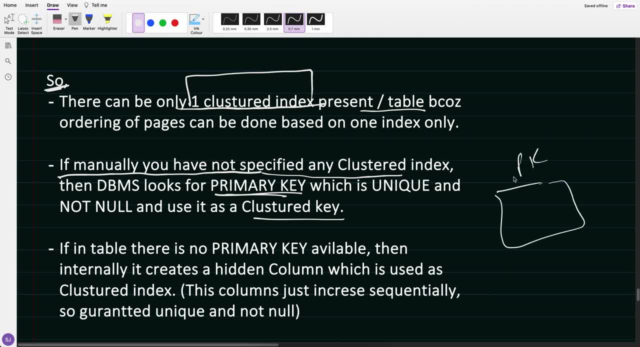 But let's say your table doesn't have primary key, Then what? what will happen? How? DBMS will create a B plus 3 out of it. when you don't have the primary key internally, which is not visible to you, DBMS create a new column and it is generally sequential, incremental: 1, 2, 3, 4, 5, 6, 7, right with every row you insert. 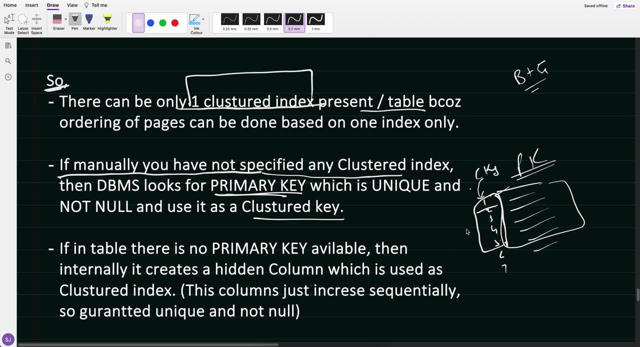 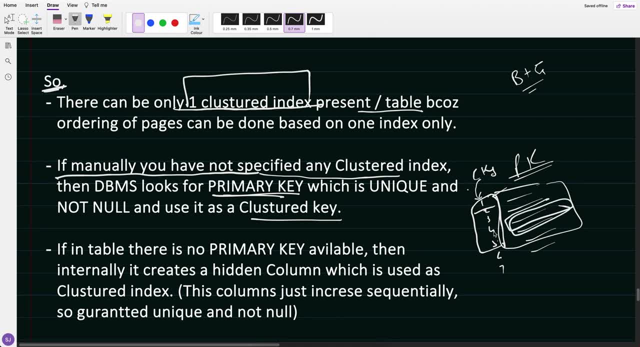 So it created as a clustered key And store the data pages based on this. So any, any new row You will insert, it will add. So this is auto increment column It insert which is not visible to you. It is used as a clustered key. 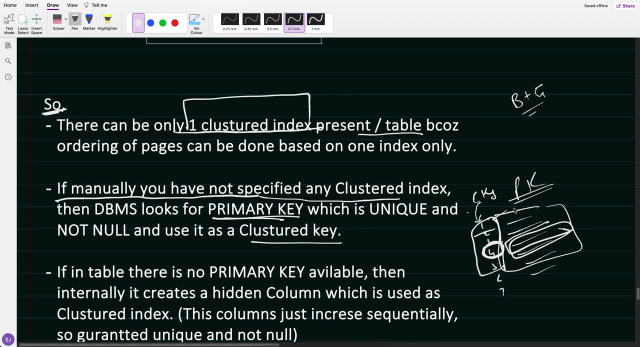 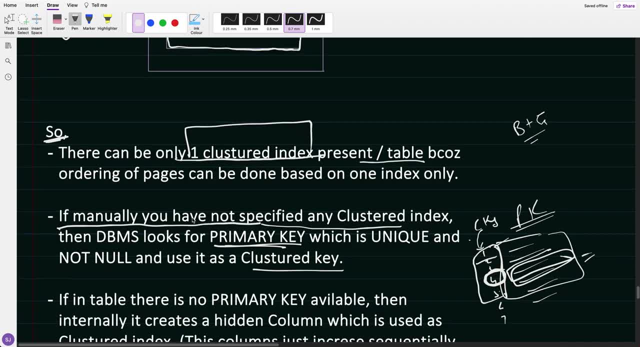 So it use that value in a B plus 3 to determine which data page to pick, where to put, what would be the offset sequence for that page and all. Now you can ask that, Hey, what if, let's say, I have a big table? 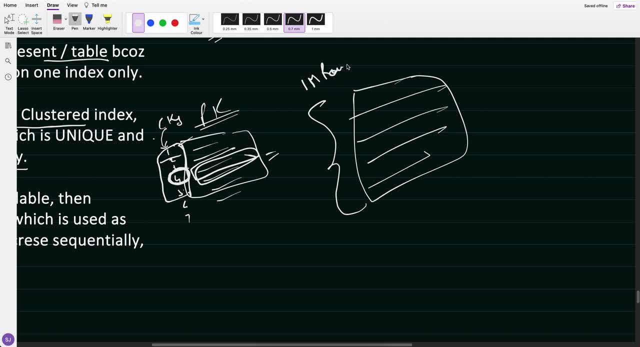 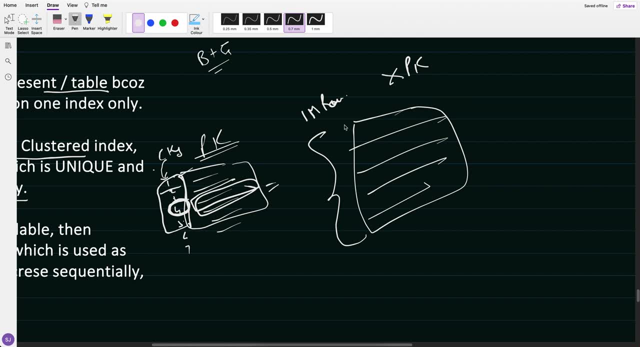 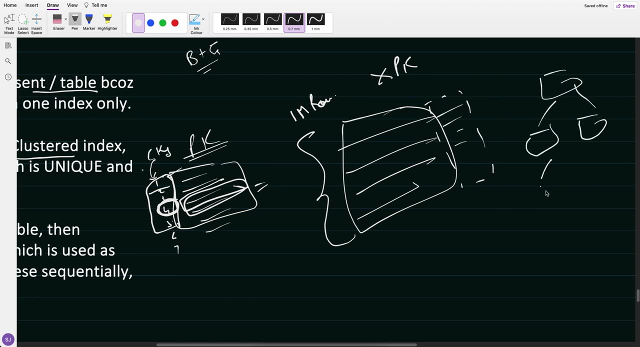 I have, let's say, 1 million rows, But I haven't defined the primary key. There is no primary key. So what happened would be: DBMS internally creates a new auto increment column and does a B tree out of it And Maintains everything. it maintains: page 1, page 2.. 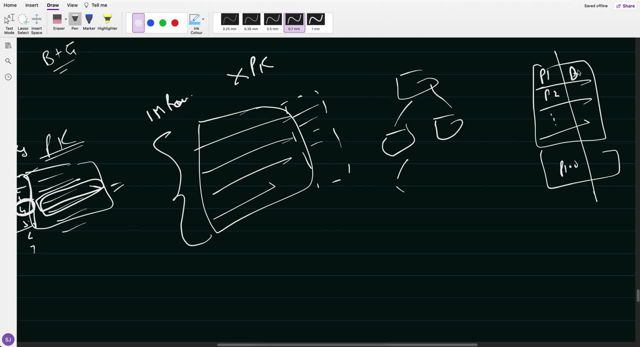 Page thousand: Data block: 1 data block to anything. Whatever the mapping it has been doing, it is doing. even the rows ordering also it is doing. But now you can ask that: Hey, what if after now I added a primary, can make one column as a primary key? 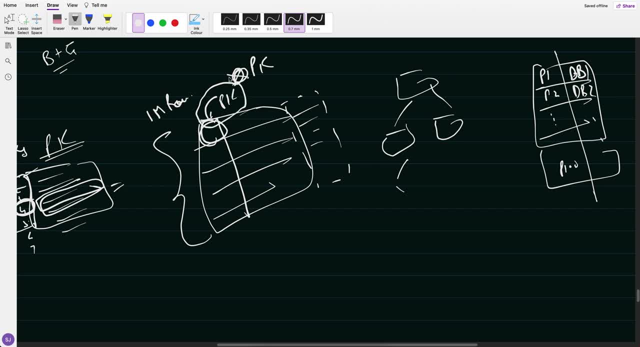 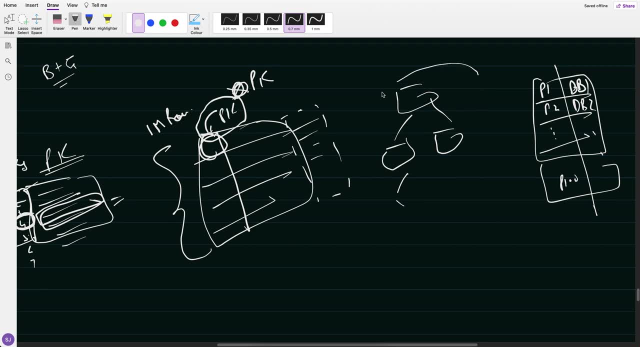 So now, as soon as you make a primary key, I told you, this will get priority. So now DBMS has to do a lot of work. It has to do regenerate this B plus 3. It has to update all the pointers now based on this. 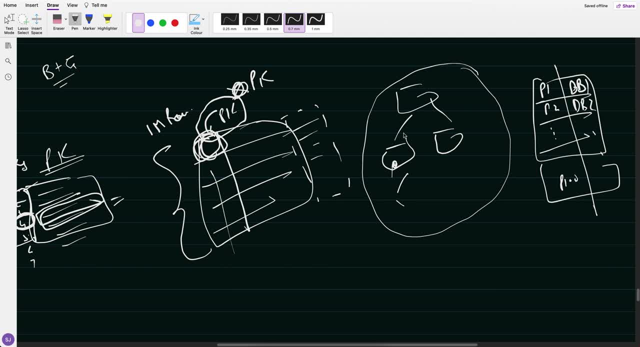 New index column. It has to update the B plus 3 pointers. It might have to load so many data pages out of the block, reshuffle the rows Right. So lot of work DBMS has to do, but everything has to be changed now based on this column indexing. 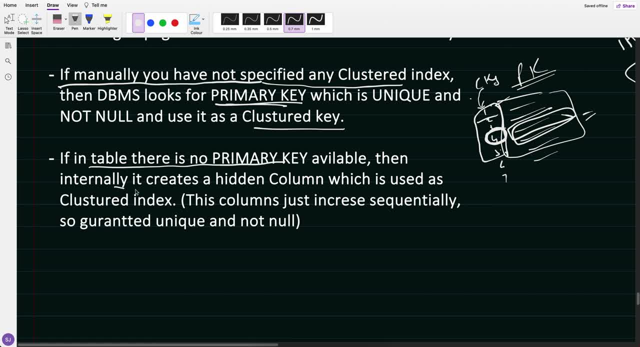 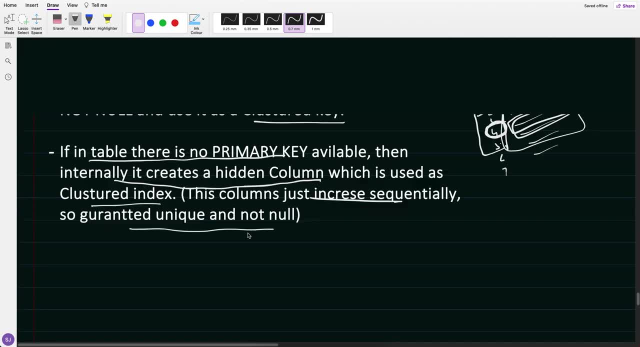 Okay, so that's what I did. If a table there is no primary key, then internally it creates a hidden column which is used as a cluster index. This column Just increase sequentially and guaranteed unique and not null. So cluster index, you already got it right. 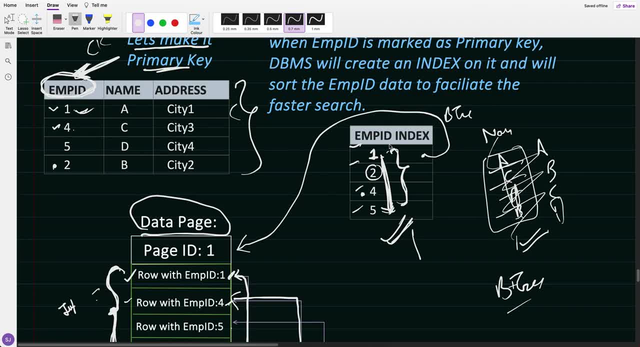 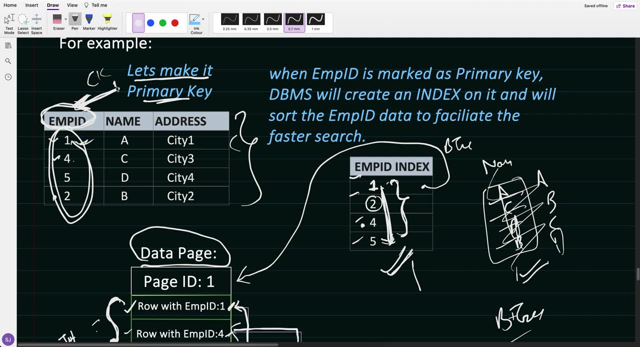 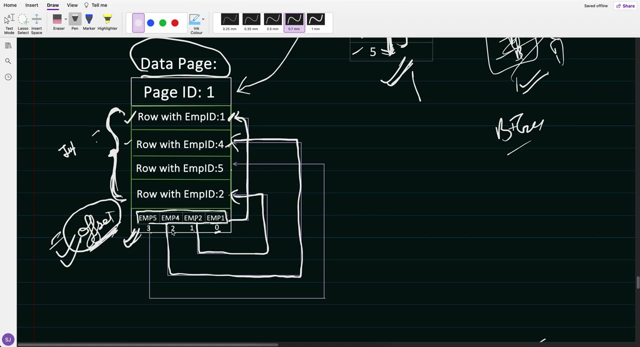 It actually Based upon this column, which is: you can say that the primary key column- the primary key column, which is always generally considered as a cluster key- It orders your rows and pages based on that. Then you can say that, hey, what is non-cluster key? 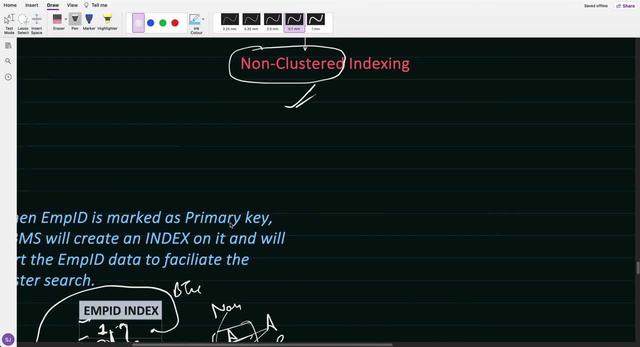 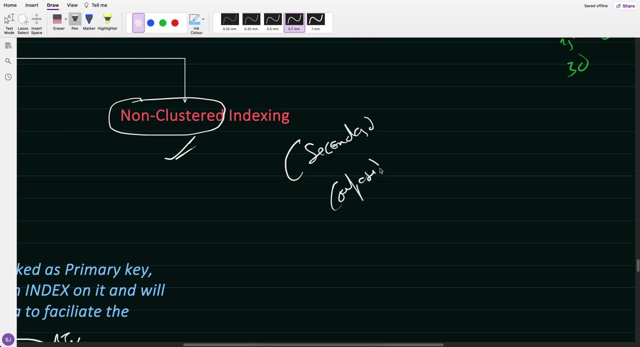 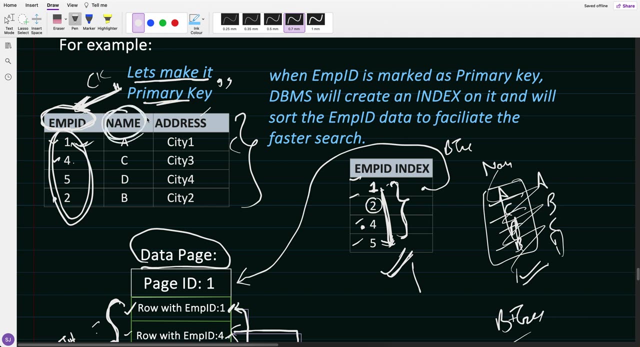 Okay, cluster key, take care of primary key, but you remember we have so many other keys also: secondary key, Composite key- What about those? also, all let's say that I have a scenario where this name can be used a lot to query, So it is better to put the indexing on it also. 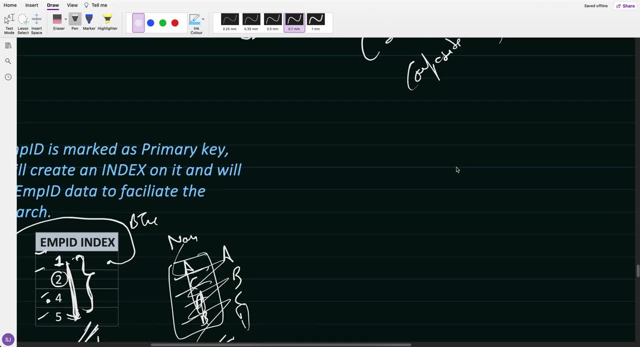 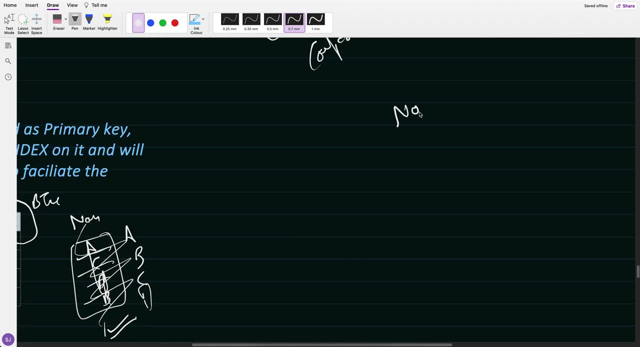 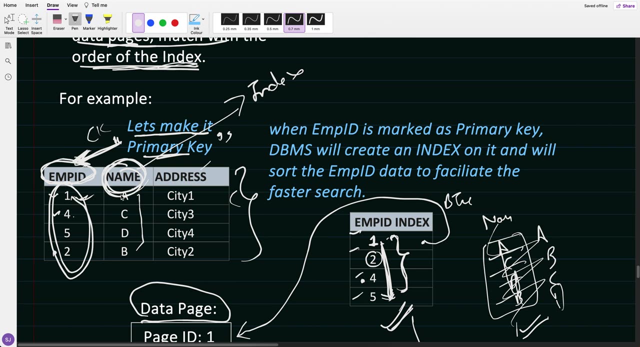 So non-clustered is like I can put indexing, or you can say that Non-cluster indexing I can put on this name secondary index, So on the name also I can put an index. Let's say I'm putting an index on name also, but now this name would not be considered as a primary key or it's a secondary key. 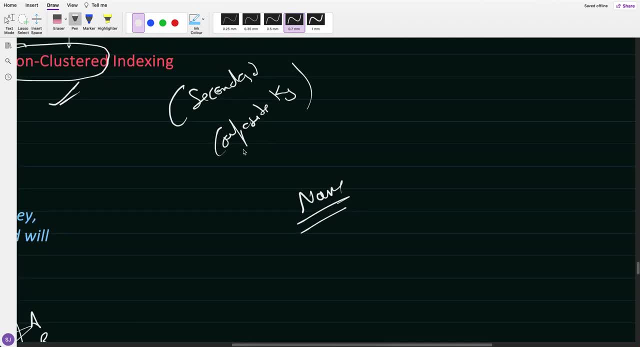 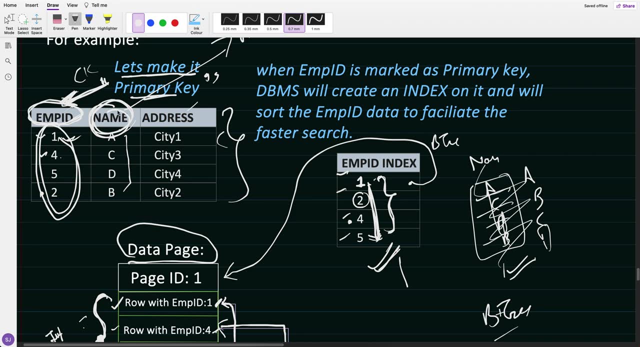 Let's say so whenever you are creating a secondary key, composite key, right, Ultimately it is doing non-cluster indexing. So what does it means that? so now let's say I'm doing name. So, based on that, B plus 3 on the name, 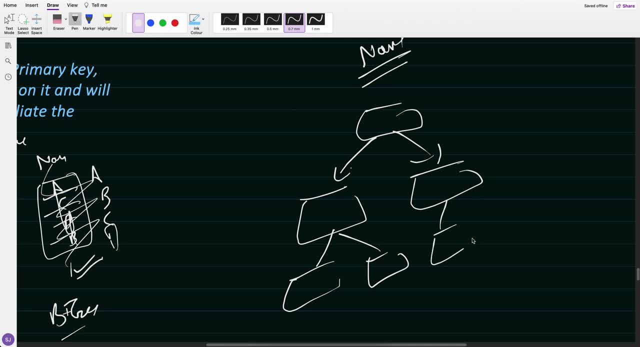 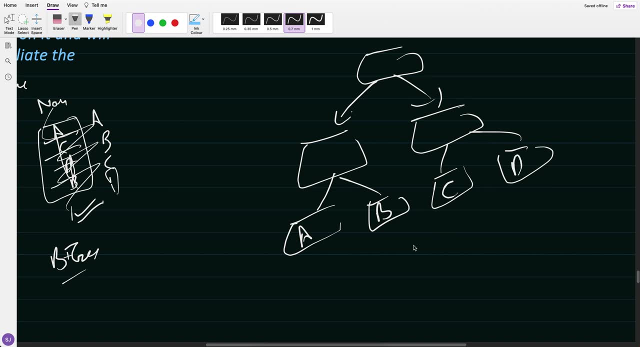 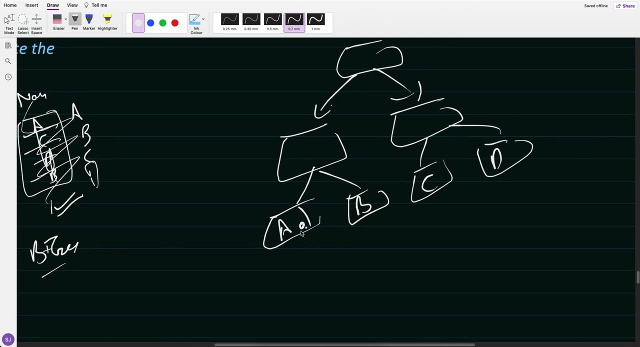 Let's say, it is able to maintain certain Sequence: that this is a, this is B. Let's say this is D, This is D, Okay, this a, now, What? So? now, two things. so it will again this: a data is stored in where 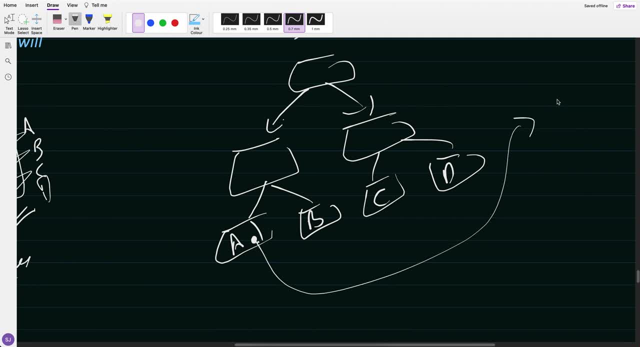 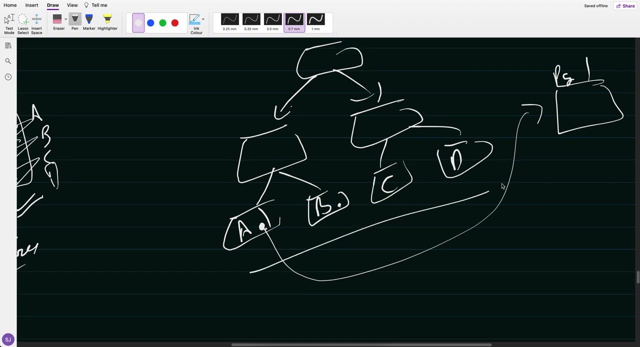 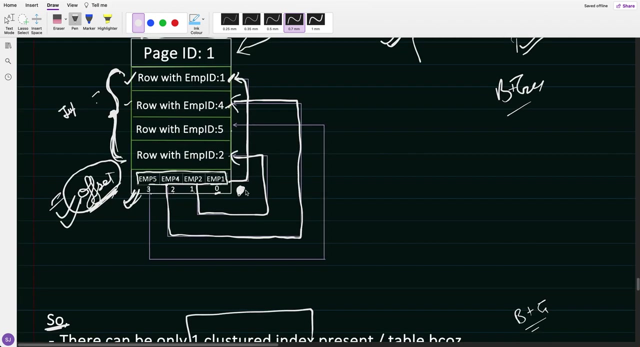 Let's say in page one, so it will point to the Page one. This B is stored in somewhere, So but here, if you see that the ordering of this offsets are not based on this, first correct The ordering of this. I would say that the ordering of the rows doesn't depend upon this secondary index. 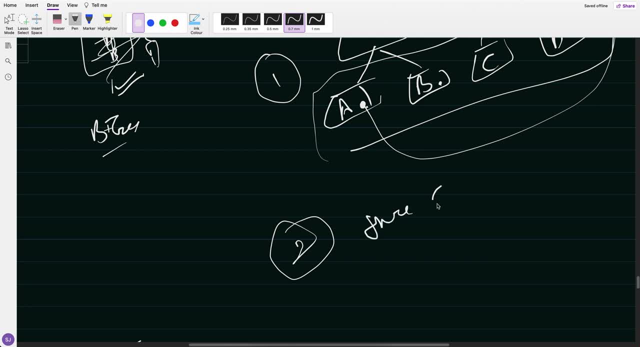 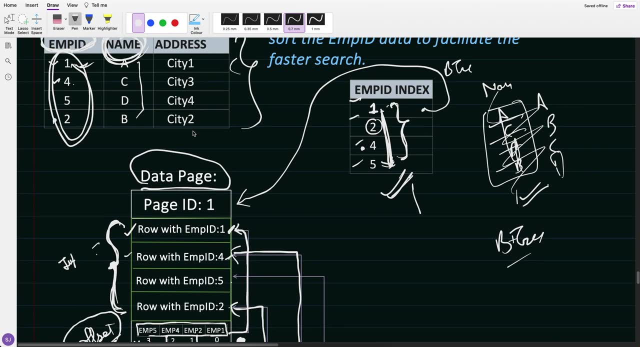 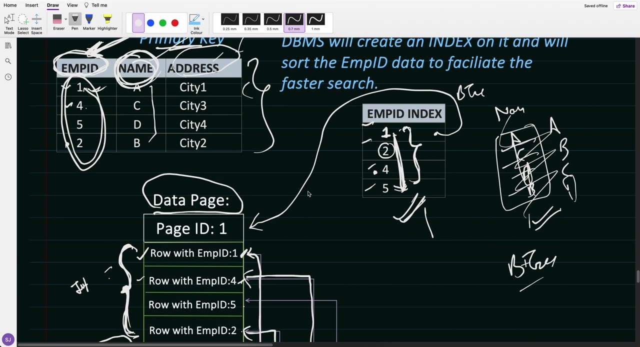 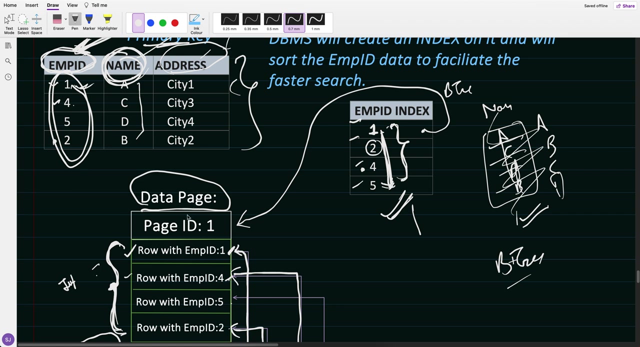 Second, There can be Many Secondary index or composite index. So I can have address also as an index. So it will create one more B tree and stores the data and just maintain the pointer to the database, Right, So we have only one clustered index. this cluster index actually drives this ordering of this row. 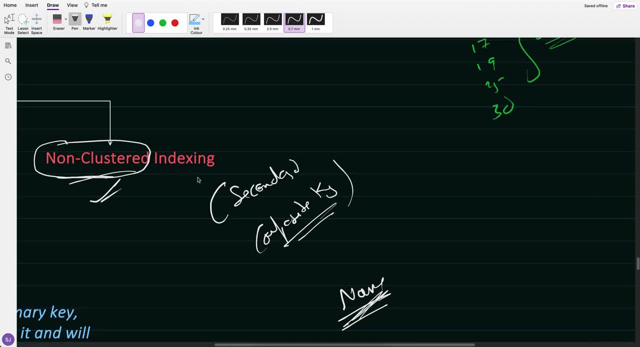 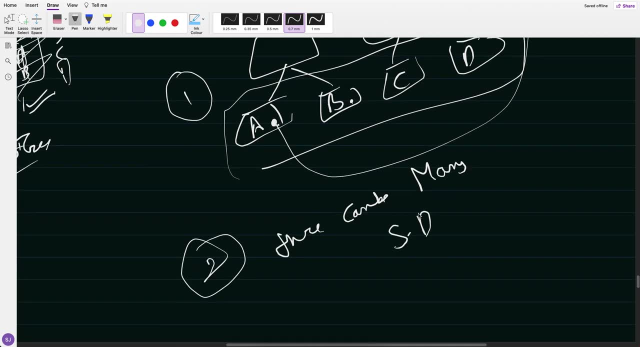 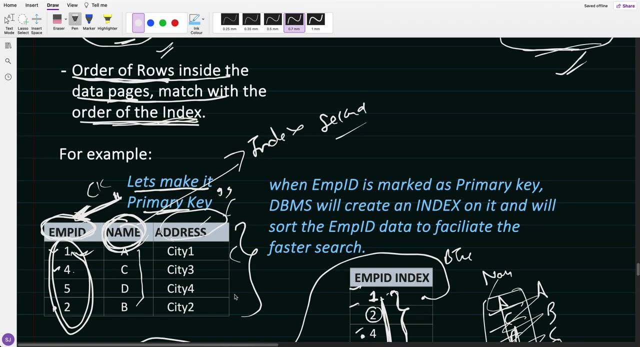 And we can have many secondary index or the non Clustered index, as your name say, that cluster. you are not clustering the rows and pages, right. So we can have many Non-cluster index or secondary index, Right, And that's one of the reason when somebody asked like you should always create index. 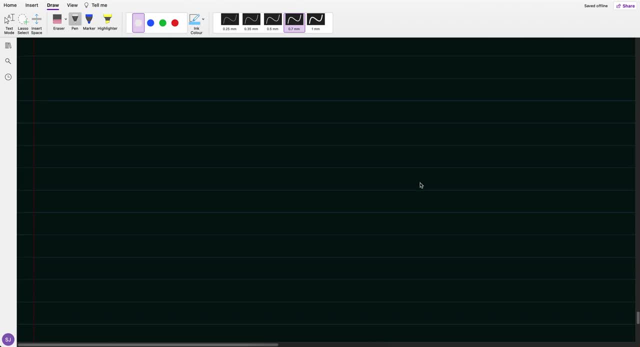 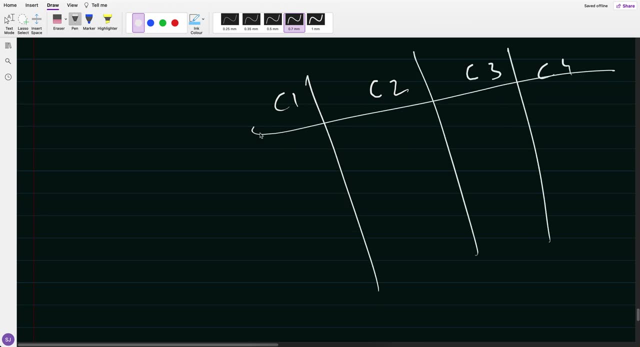 You can say that we should not like. I have 10 columns, Let's say column 1, column 2, column 3, column 4.. You might be asking that, hey, shansh, Why can't? so? this is primary key. Why can't I put this? 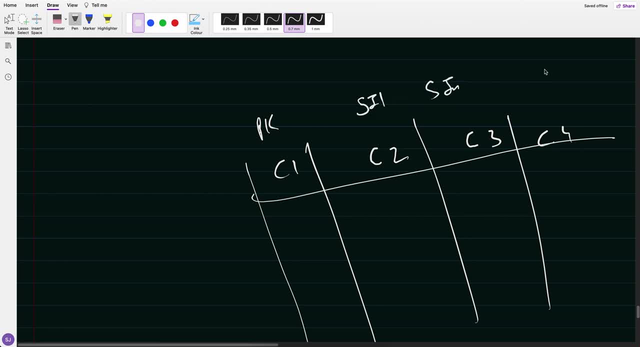 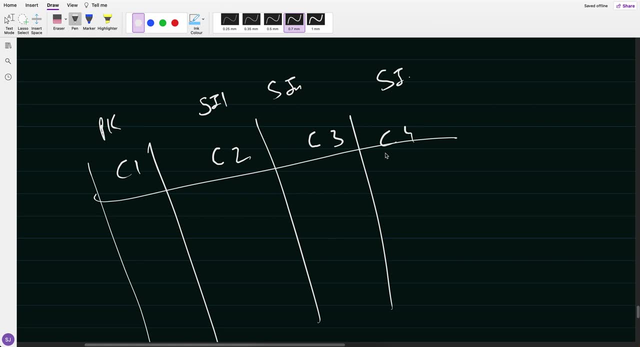 I this. I will also make secondary index. This is also. I will make secondary index. This is also. I will make secondary index Over like whatever the query will come, It would be faster. Now you understand, at least grab that there is a overhead. 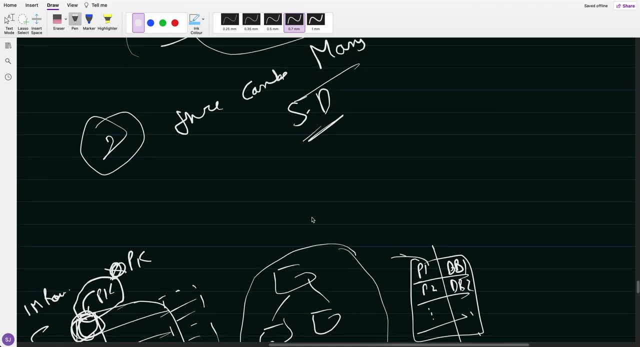 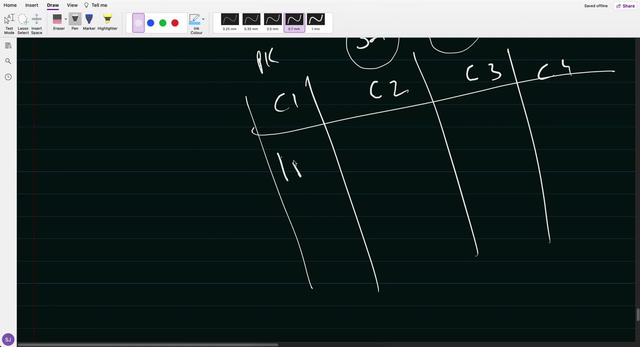 So for each secondary index you have to maintain a B plus 3 for it. Now, if there are 1 million rows in this table, let's say 1 million rows means in a B plus 3.. You are creating so many keys here, right? 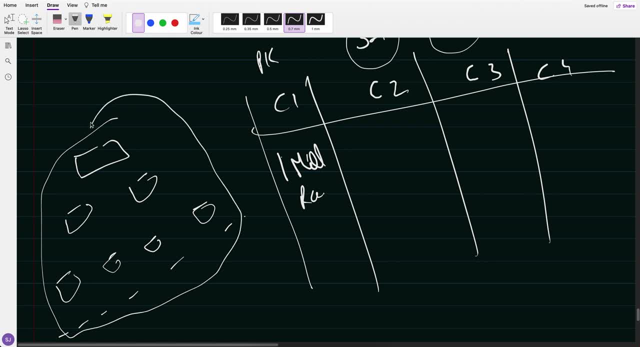 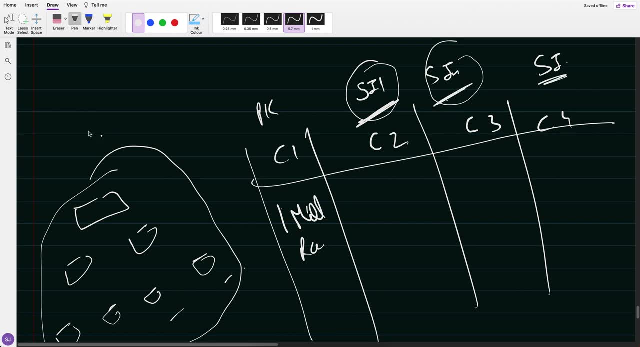 You can just consider the amount of memory It also required, Right? Let's say, if you have three secondary index, so means you are creating three B plus 3. Like a non-clustered index: one for this secondary index, for this column 2.. 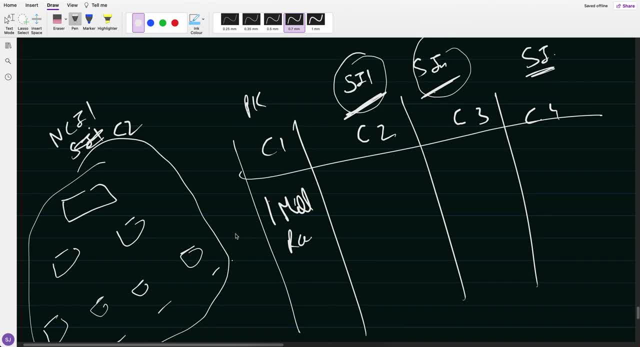 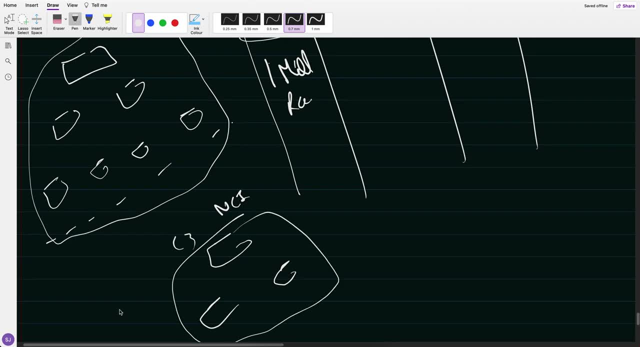 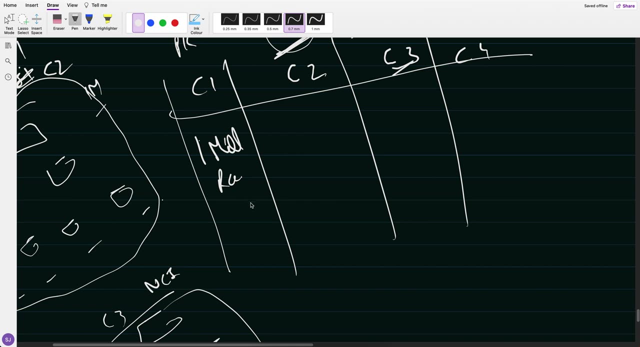 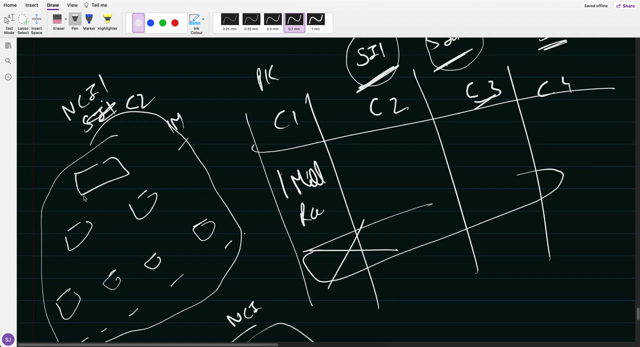 You might be creating another B plus 3.. For non-clustered index indexing You might be doing for column 3 for again 1 million record Like this: now, Assume that any row, particular row, is deleted, You have to update the pointers also of this. 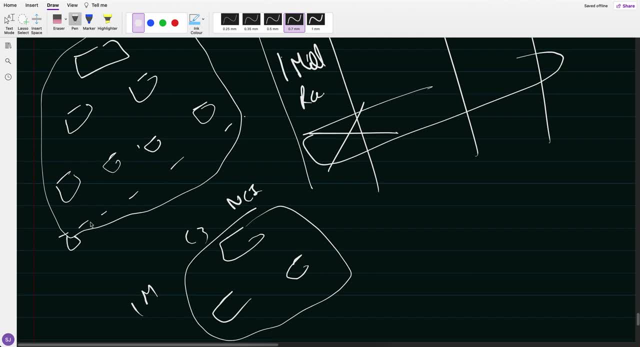 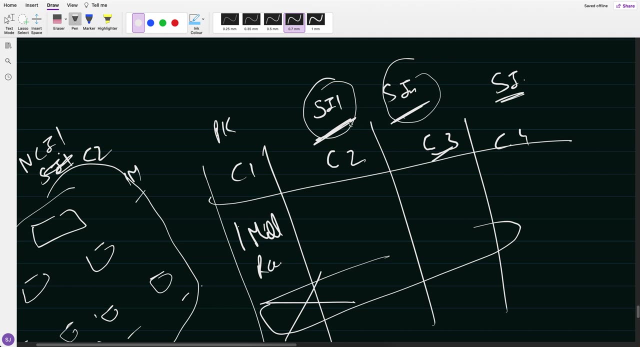 You have to delete that row, or because this is the leaf node has the index value, You have to delete that node also, And when you delete it, you might have, it might be possible that you have to update the pointer also. So that's why it is always say that create an indexing carefully. 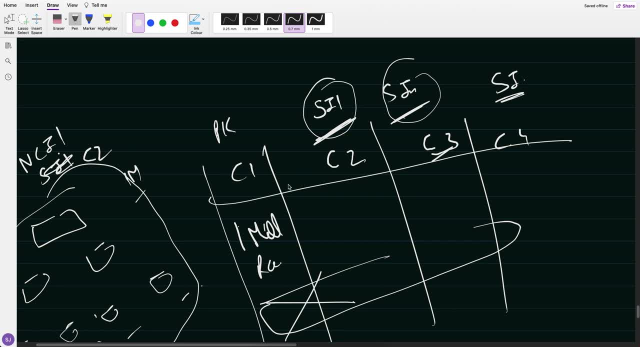 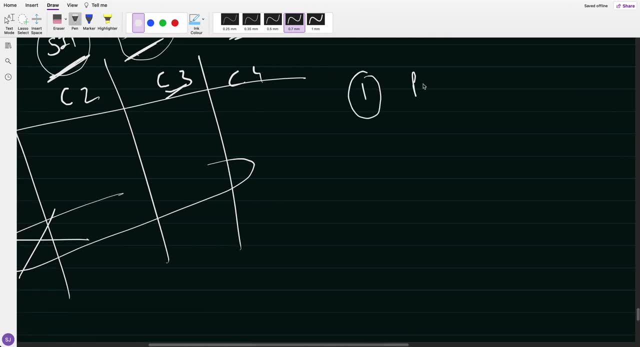 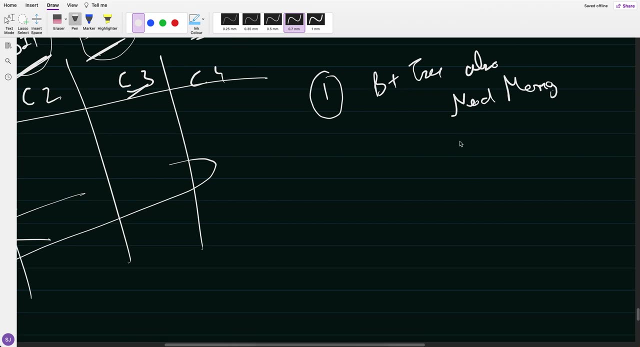 It is not easy Because there is a lot of overhead comes in. What are the overhead? First thing is this: B plus 3 also needs memory. So you have to worry about the memory also, because this is also ultimately going to store in the disk only. 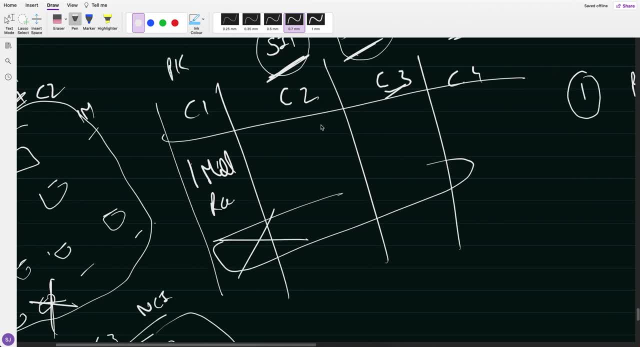 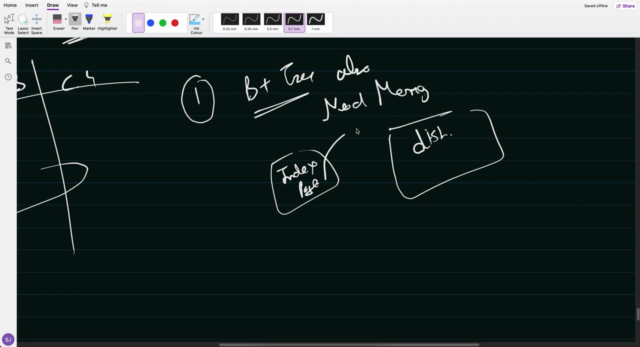 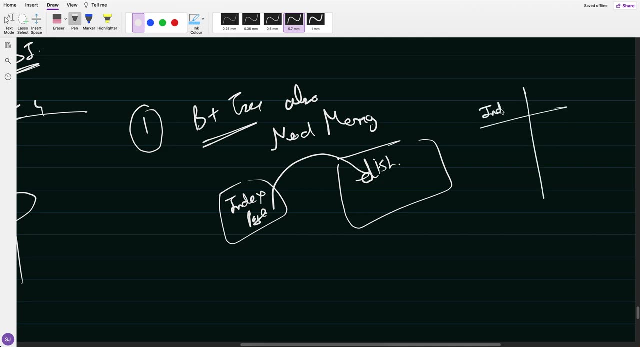 Right, and it DBMS also. whatever the data it is stored, It also stored into a pages, which is known as index pages, And this index pages are stored in disk only. So there is a overhead that it maintain the index pages. So, because I told you that, 1 million, 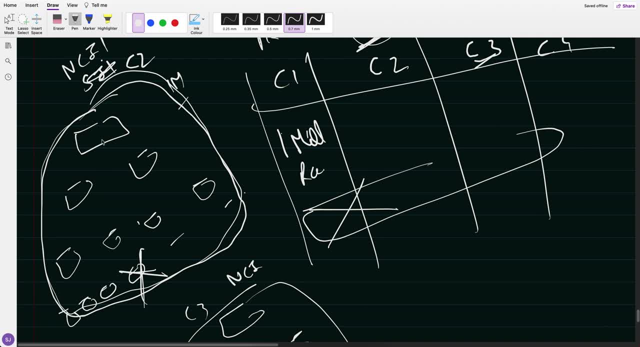 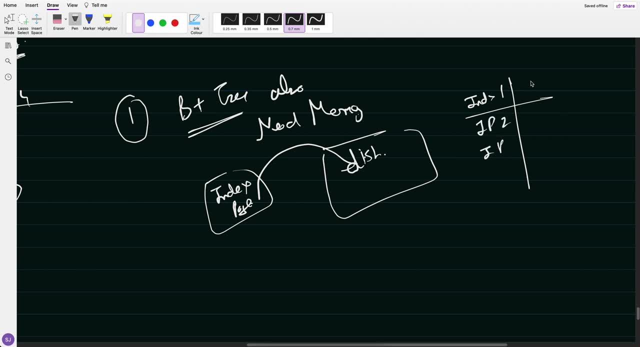 Notes it created. definitely 1 million note cannot comes into one page. It might have to create so many index pages also. index pages also comes into so many. Let's say block, block 5, block 6, block 7.. So now you see the overhead which DBMS has. 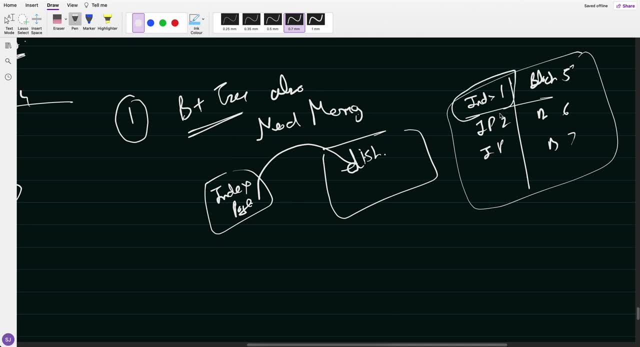 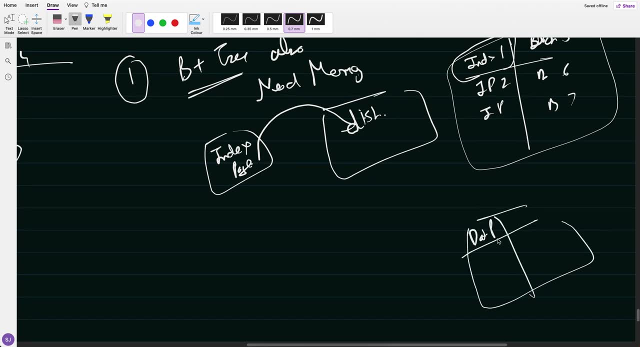 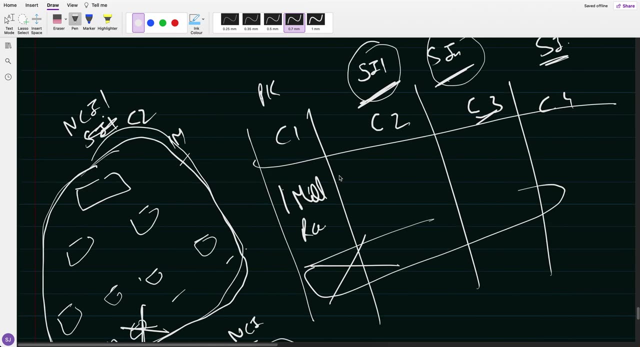 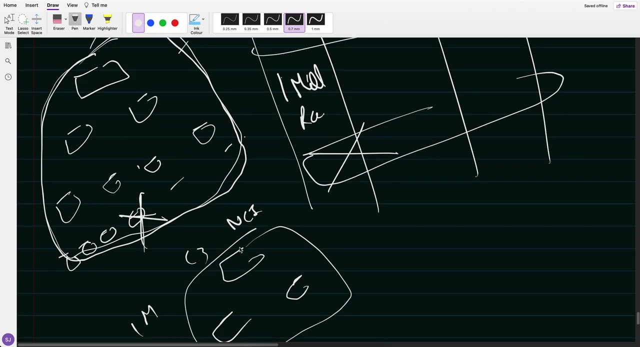 It has to maintain the index pages Also index pages mapping. Also. it has to maintain the data page where the data is actually stored and it's mapping also blocks. So just creating a secondary index, composite index and indexing will just create an additional overhead and any addition any, because anytime you add a new element 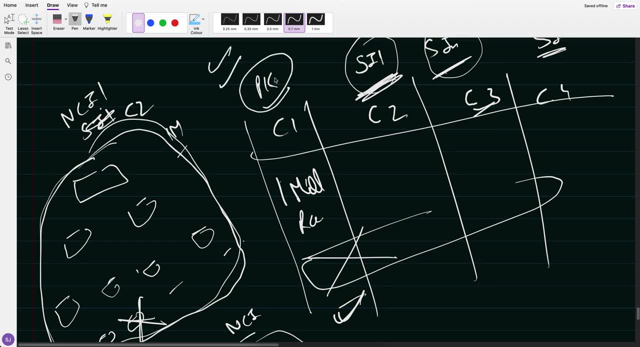 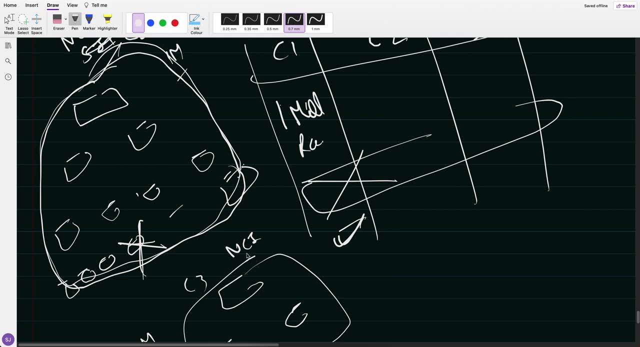 You have to update your clustered index: the primary key one, then all the secondary. you also have to update and in the update I already told you page split can happen. when the page split happen It might divide right. So index has to be update. 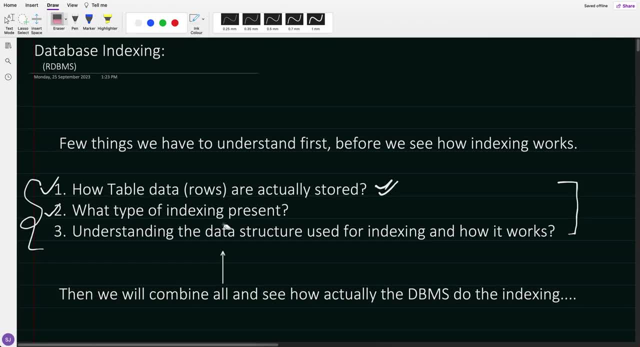 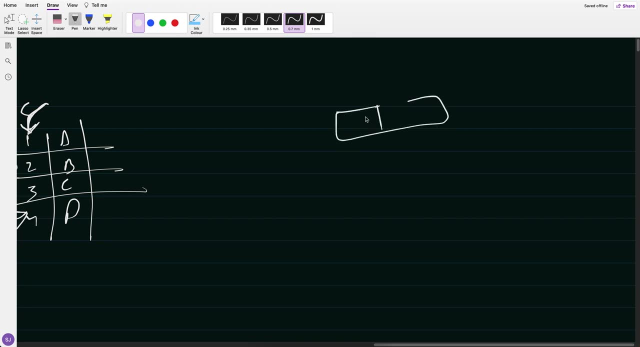 So I think it's pretty much clear, right? So now you know that what all things has to be done. So whenever, whenever you have to, It looks simple, right? So, whenever you have to insert one row, new row, what all things it does, right? 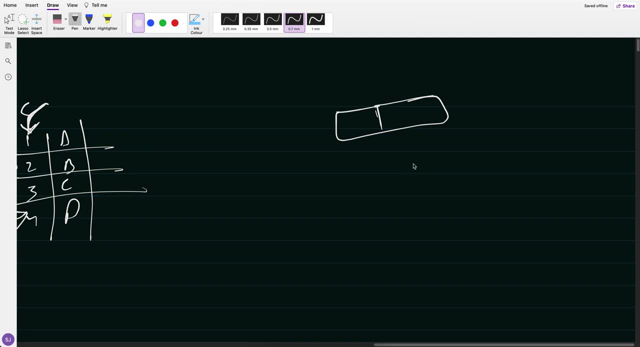 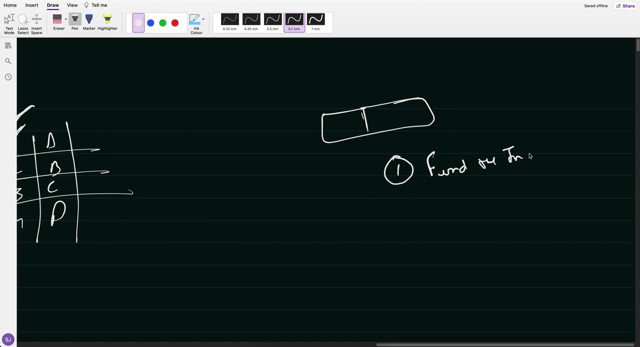 It first find an index page Right. What would be the first step? it first Find the Index page Right. So in from the index mapping: Index page 1, index page 2.. Let's say block 1, block 2.. 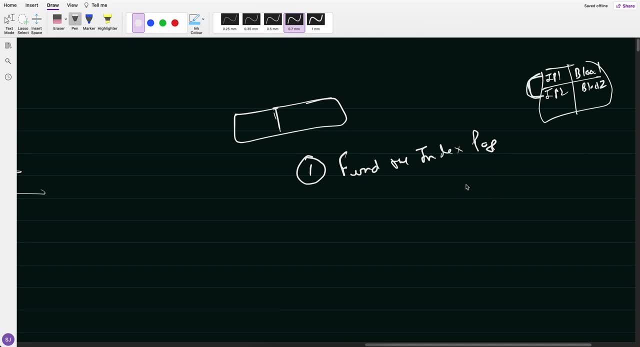 So it will first load the indexes pages into the memory Right, because indexes pages has your B tree data combination indexing right. So, second, what it will do is: or you can say that, so let's say, or I would say that instead of inserting, 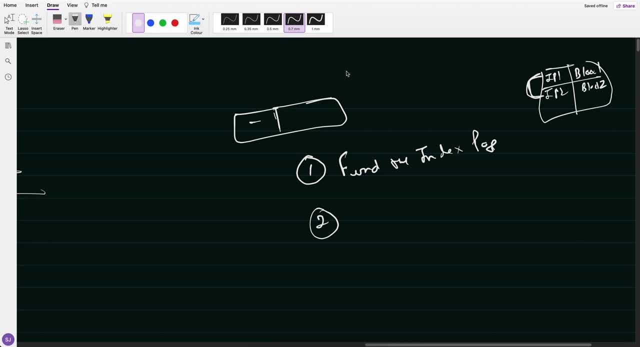 Let's say you want to search because we are talking about search query. So let's say you want to search a data with 35. Let's say I'm saying ID, So first it has to load the index page. index page is loaded from this data blocks. 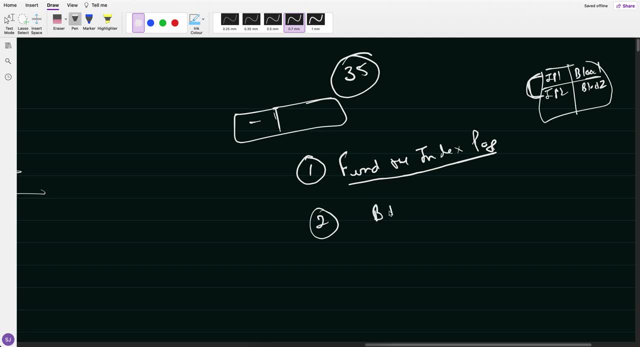 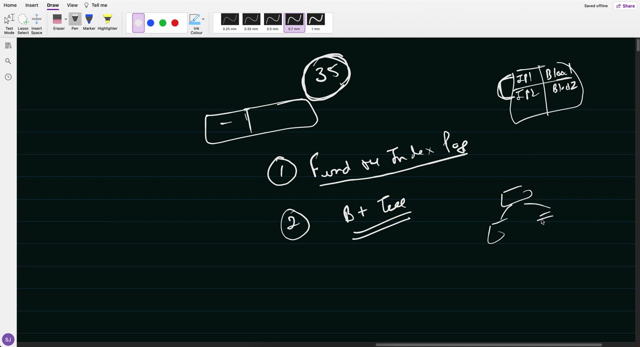 Now, from this index pages, it will run the B plus tree. It will traverse this B plus tree To find Which data page this 35 has. so maybe you have a data page this indexes has the data. So now let's say this 35.. 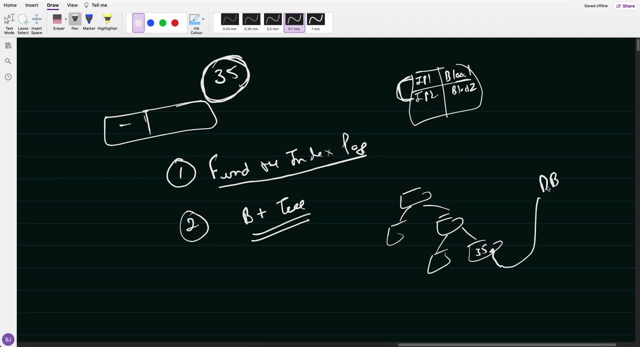 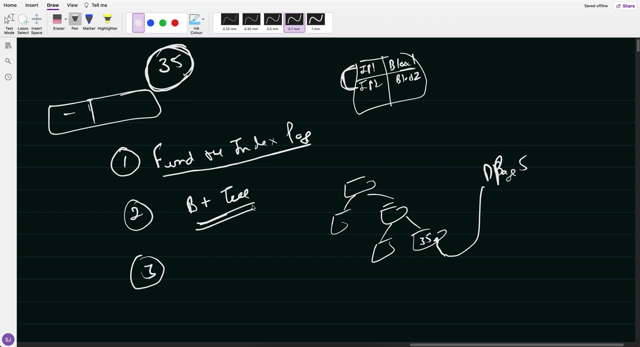 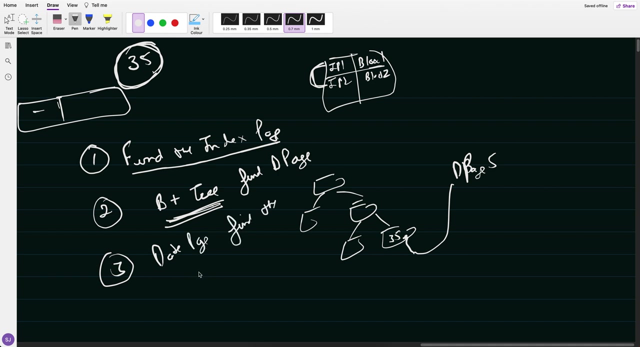 Ultimately points to A particular data page, data page 5,. let's say So now from for. second: establish using the B plus 3 and find the data page. Third step: use that Data page, Find the Data, block It. maintain our mapping right. 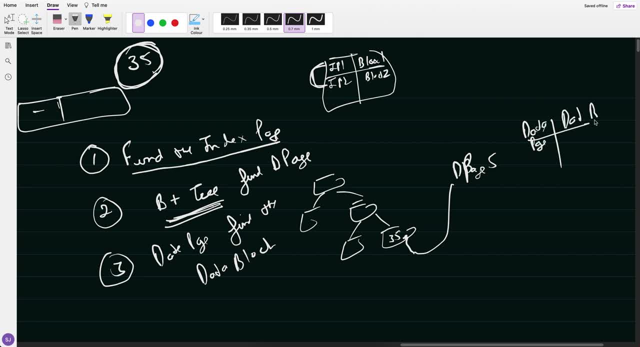 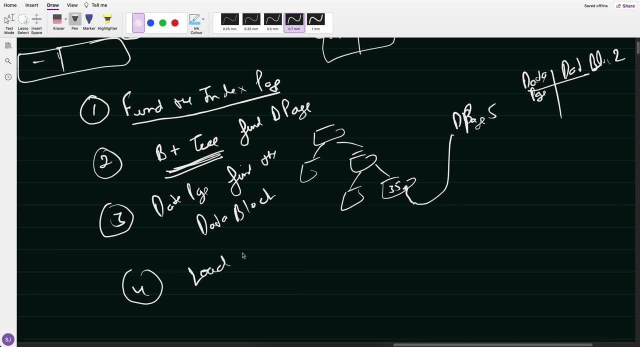 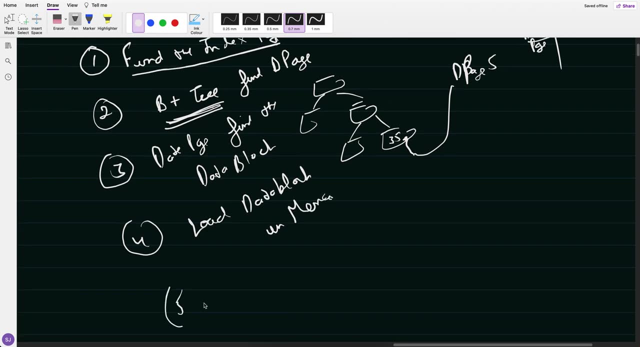 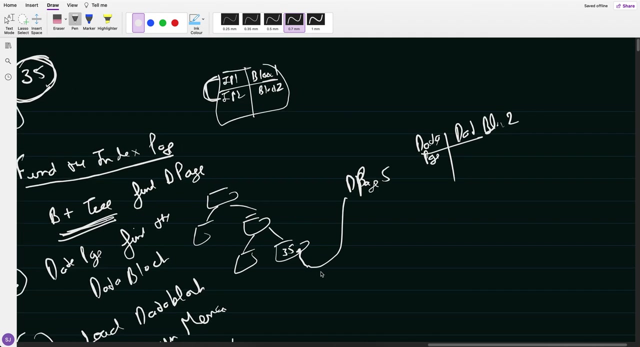 Data page, Which data block? Let's say 2. So now it can directly goes to that data block: load That data block In memory Right. fifth: read the data Right. So now, even if there are hundred thousands of data block, it doesn't have to worry. 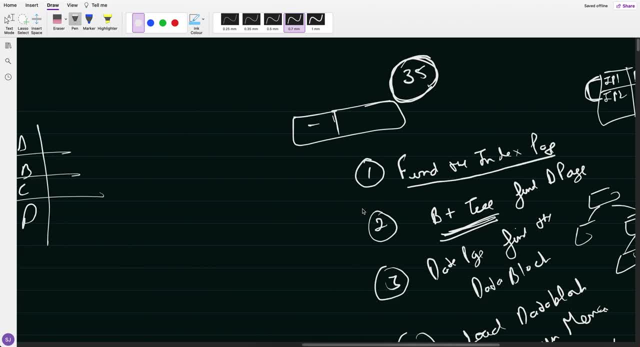 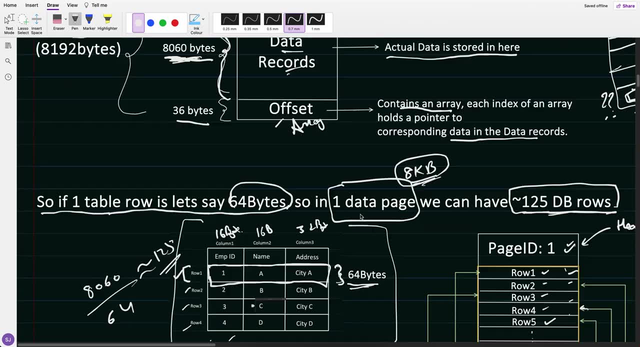 It can directly goes to that particular data Block. Okay, so this is Check it out one more time. It would be little bit clear, but this is So. many things happens Right in the background and we can discuss more, if you have doubt, in the comment section. 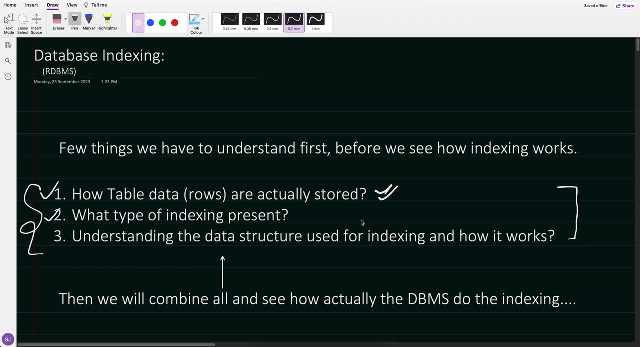 And even, if you wanted, I can have one live session where we can discuss more. Okay, guys, Thank you Bye.